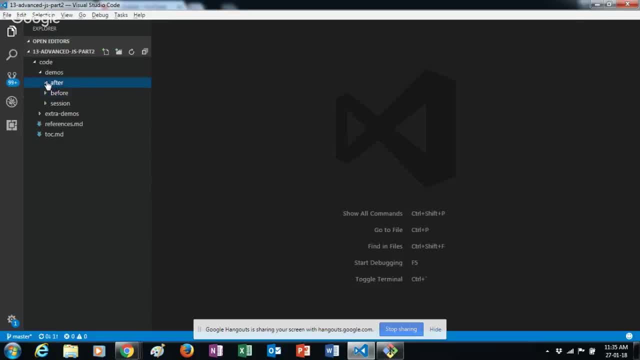 All right, So last time we had seen- okay, this is for the benefit of people who had not attended- last time we had seen some of the features, like the use of let and const. We had seen certain things. What have we seen? 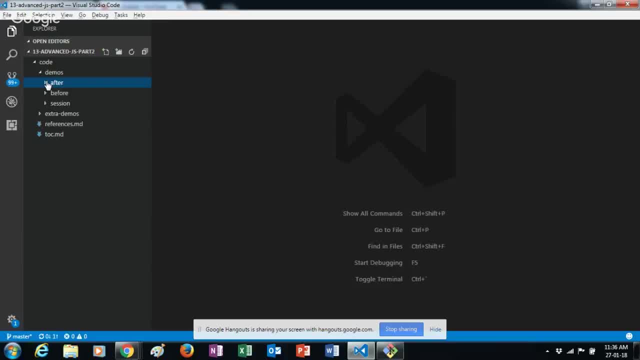 We had seen how let differs from var and all. All right. And a few of the other features we had seen. All right, Okay, Yeah, So template strings, default arguments and functions, destructuring arrays and objects. That's what we had seen. Okay, So I'll be continuing from where I left. 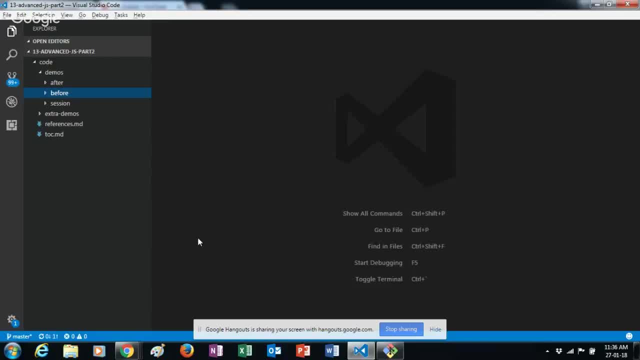 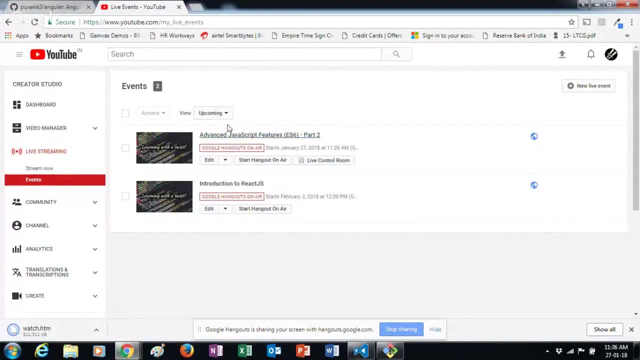 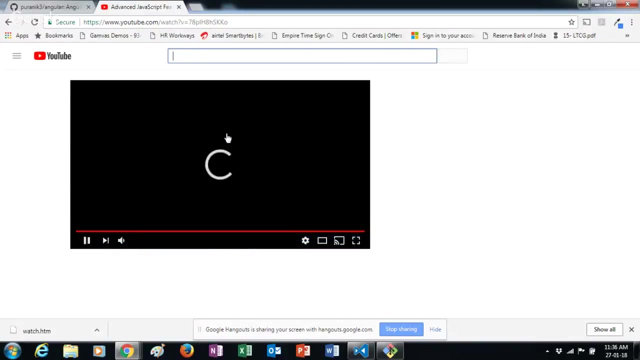 Okay And I'll start. So, before I get started, I just want to uh, uh, have a check. Is everyone able to hear me clearly? You could let me know, Uh, I think, uh, you can let me know any questions you have, If I'm able to, uh, if you're able to hear me clearly. 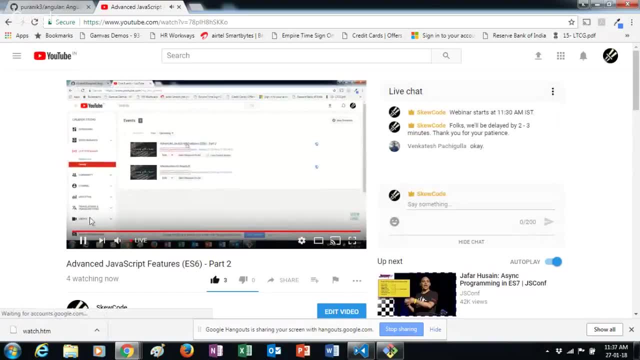 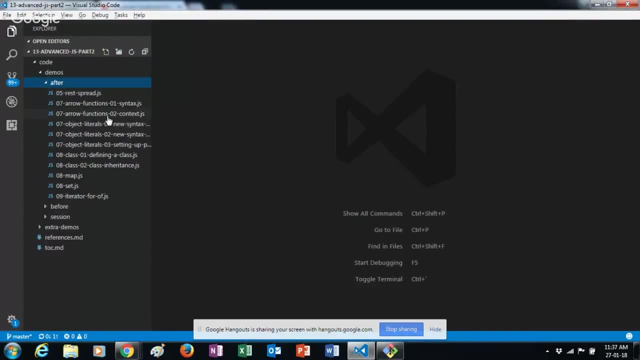 you could let me know. Uh, yeah, I think I'm audible. Alright, Yes, All right, Thank you guys. So let's get started. Uh, so, we're continuing with rest and sprite. all right, That's the first thing. I'll uh take you through. 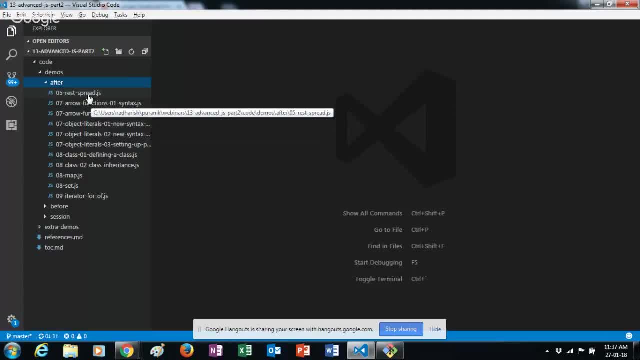 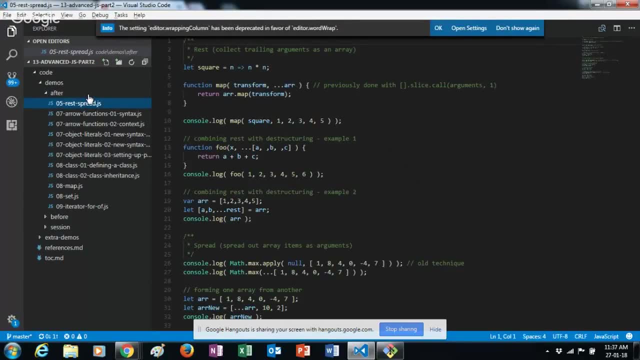 Then we'll go to auto functions today and then we'll see objects, classes and maps. So we will have one more probably a session where we cover some of the other features of ES 2015.. Alright, So coming to rest. So this we had seen a bit last time, all right. 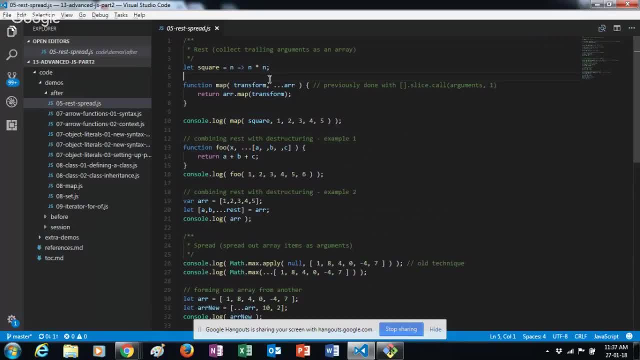 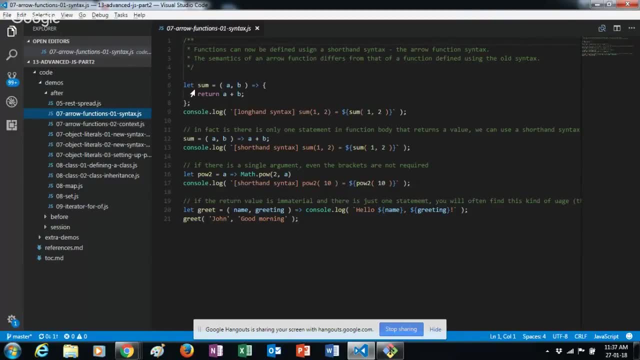 So we have created a function here. okay, Let me start off with the arrow function, because I'm using arrow functions here, So I'll start off with arrow functions. So till JavaScript version five and something like this. you'd use a function keyword. 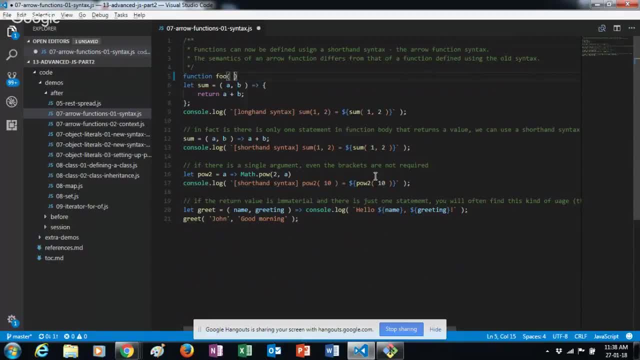 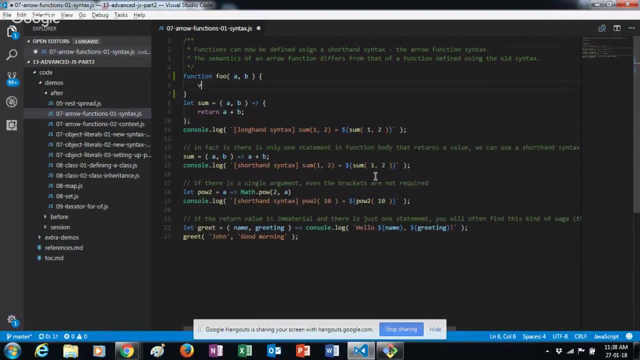 Then you'll give a name for the function, Then you'll give the brackets and give the arguments And finally you'll have the function body within braces. The function might do something. For example, it could calculate the sum of A and B. 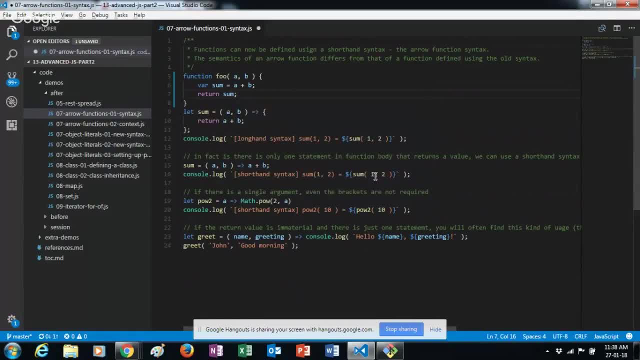 the arguments and maybe it could return it. all right, So this is the way you would write a function, But in ES 2015,, there's a new way to define, a new syntax for defining functions. that's called arrow functions. 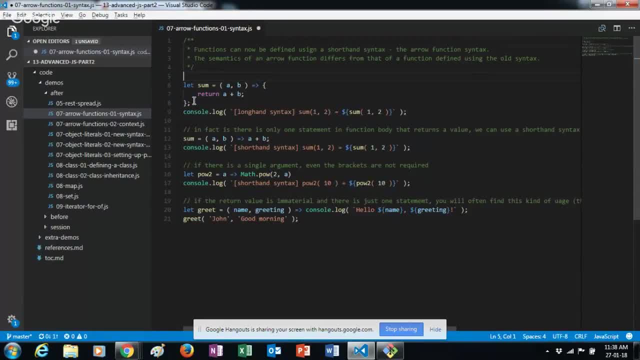 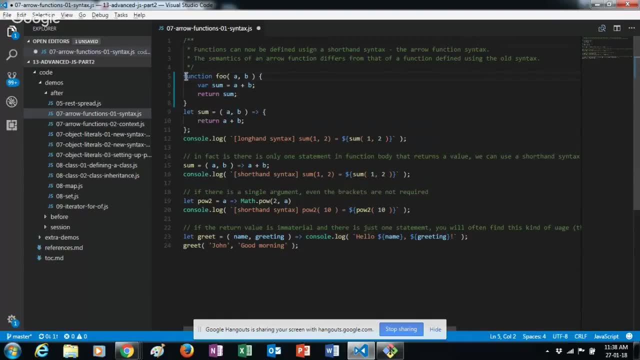 So what you do here is: you create okay, or you create either this way, Okay, or you would do this way too in JavaScript. So you'd say: okay, var foo equals a function keyword, and then the brackets, followed by the arguments. 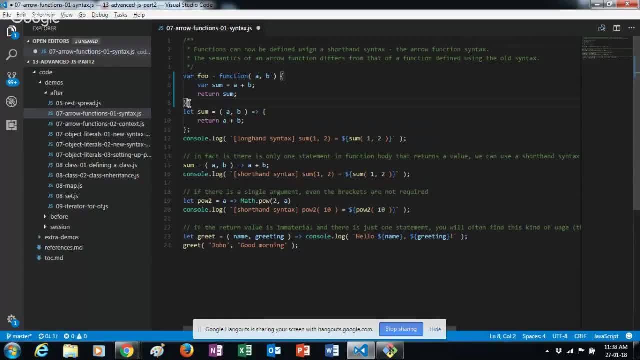 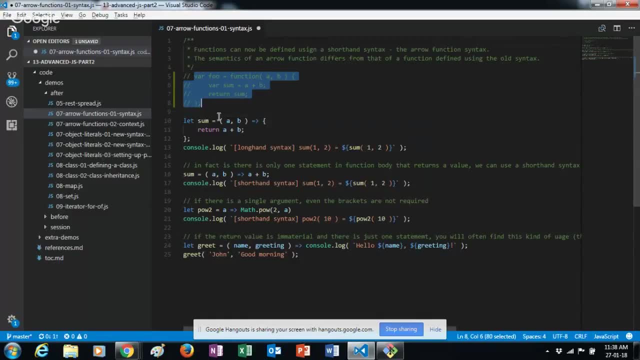 So even this way you could do, and this would become the function name. So this is the other syntax. okay, This is that in ES 2015.. So I'll just comment this out Now what you have. okay, these are the after demos. 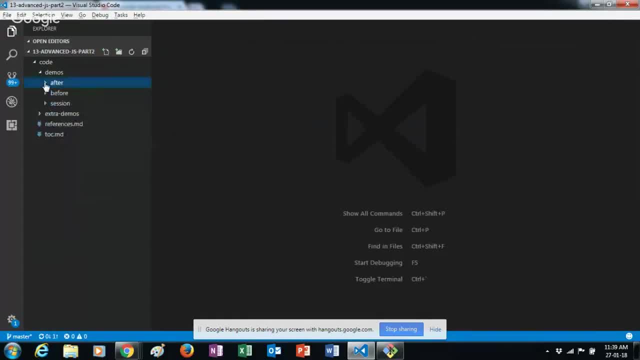 So I have to use the before demos. all right, So this is for. this is a completed demos for benefit of those for attending for the first time, And this is the folder with the comments that you'll have to follow to get. 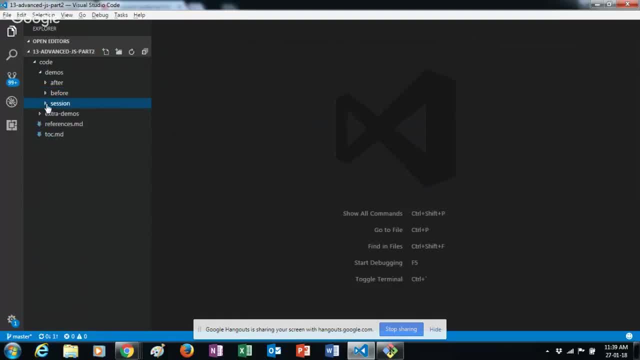 to learn about the features, And this is just a copy of that. I'll be using this copy of the before folder called session. So after is that which is a completed demos, then before and session. all right, So probably I don't have in the session everything. 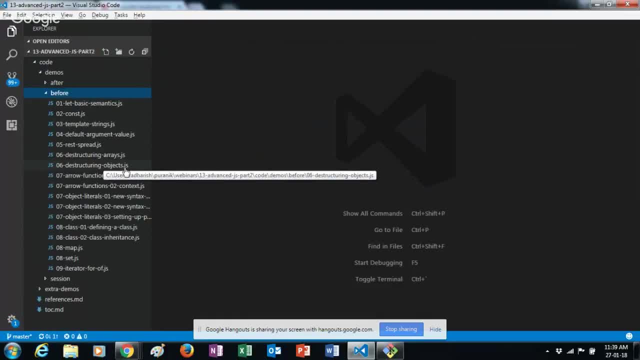 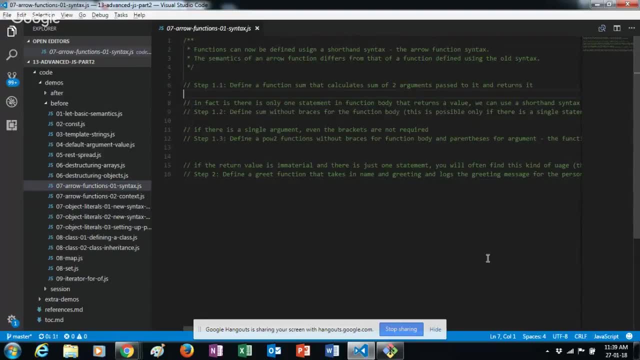 so I'll use the before folder only. So okay, so arrow functions. So now what you can do is you can define a function this way. I'll use the let keyword. I'll say let sum equal to the same thing that we just saw. 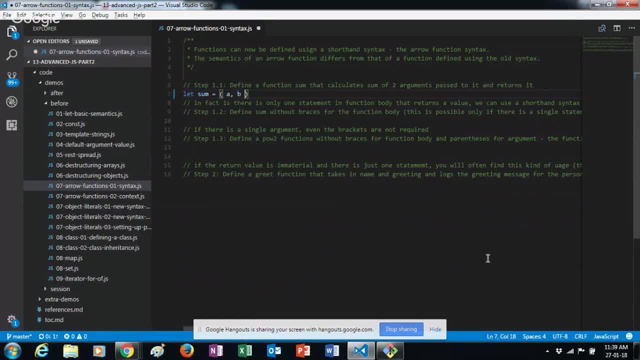 You give the arguments within brackets, like this: You don't use the function keyword And then you give an arrow, an equal to, followed by greater than symbol. Let's call the arrow operator, okay, Fat arrow. So you use that. and you define the function body like this: 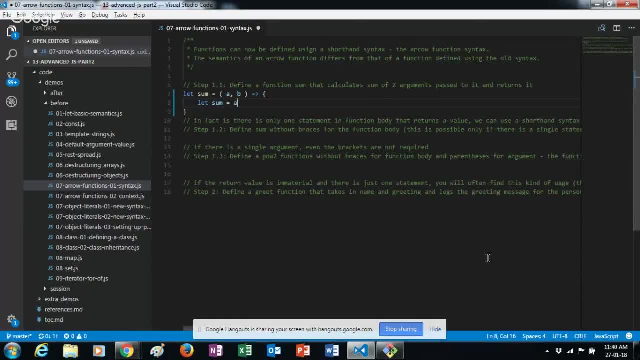 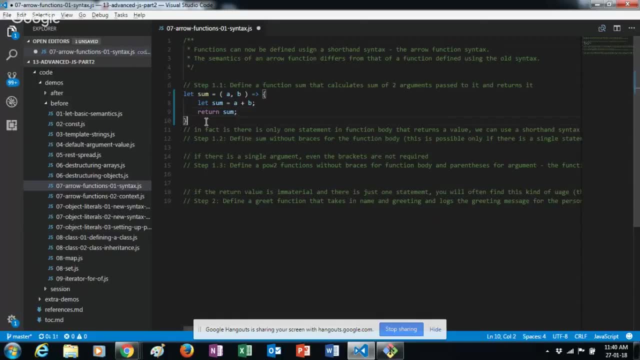 So you would say something like: okay, let sum equal to A plus B. So you would say something like: okay, let sum equal to A plus B And then return sum. Okay, so this is the new syntax Syntax example: the variable. 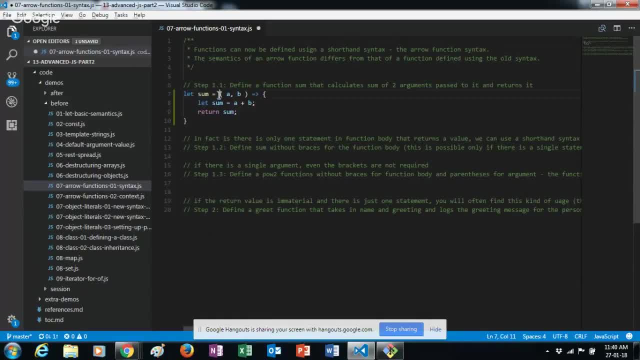 Okay, it's a function expression. So you say, let that variable equal to, So the function expression. you define it this way, which is basically brackets, arguments, fat arrow and then body of the function. Okay, so this is one thing. 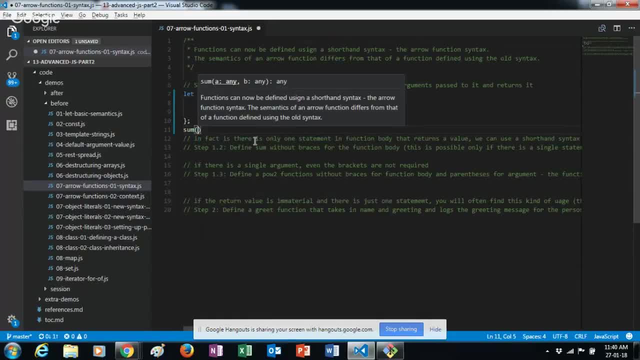 Suppose now you can execute this and see, for example, sum of A and B. So one comma two, that should give three. So let's log it. I don't have Nodejs installed on my system today, So I'll show the output on the browser console itself. 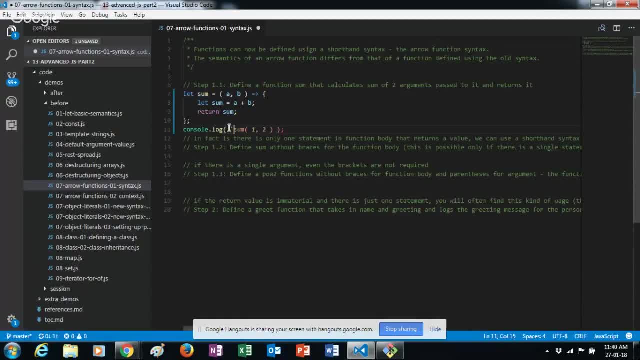 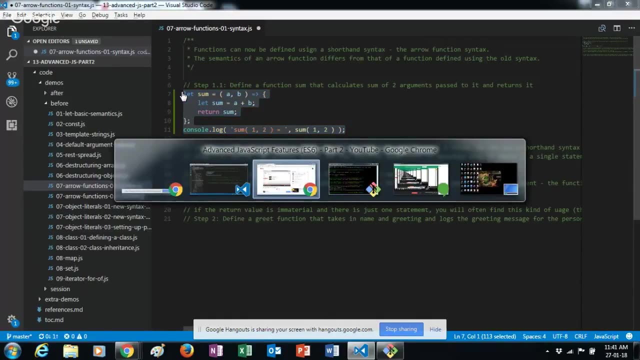 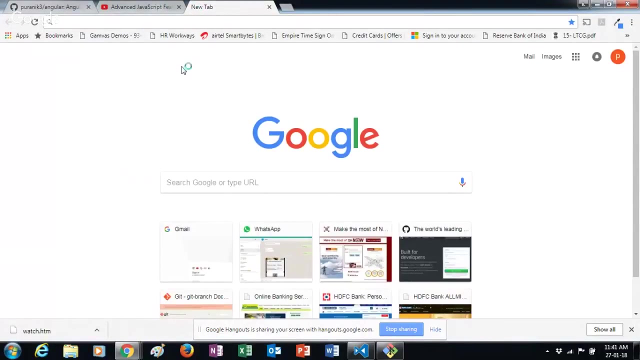 All right, so let's copy this. All right, so If I execute this, you'll see that it works fine. Okay, so let me open this in a new tab And I'll open the browser developer tools. Okay, go to. 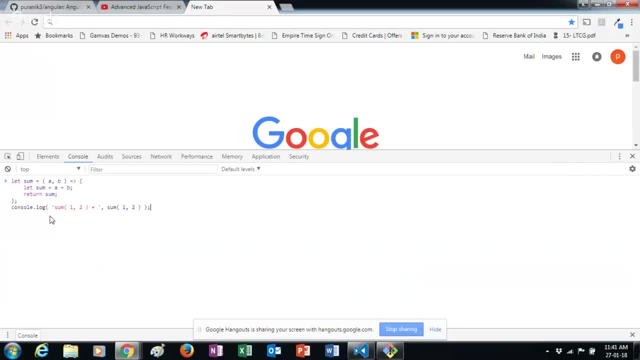 And let's execute it here. All right. so you see, sum of one two equal to B. It's printed onto the console, all right. So basically, this is the new syntax for defining a function. This is called an arrow function. 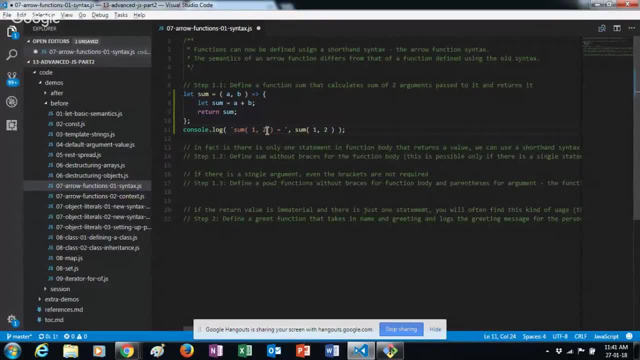 Now, this is not only a new syntax for defining a function. even the way the function behaves is different, So the function also changes. Now, what that means, we'll see in further examples. We have defined a function in a different syntax, okay. 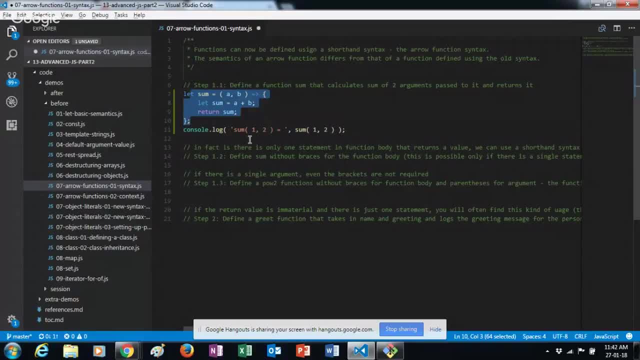 Let's see some more about the syntax first, before we move on to the way the function behaves, how it behaves differently also Okay, before that we'll just see some more details about the syntax itself. Suppose there is only one statement, For example, the same thing could have been written: 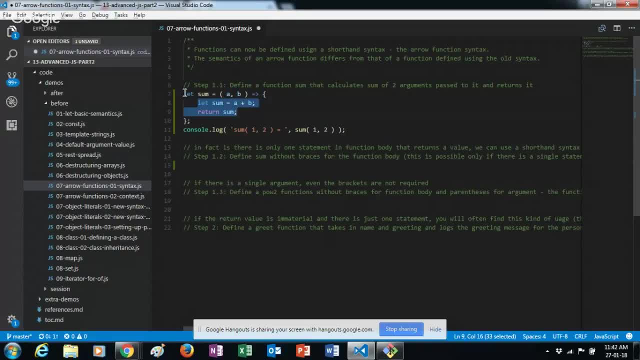 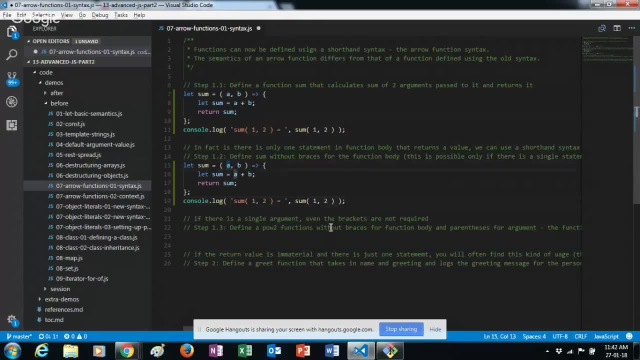 in one line: return A plus B. Okay, let's do that. So, instead of doing like this, okay, what you could do is that there is a shortened syntax or a simplified syntax where, if you have just one line and that is returning something like this: 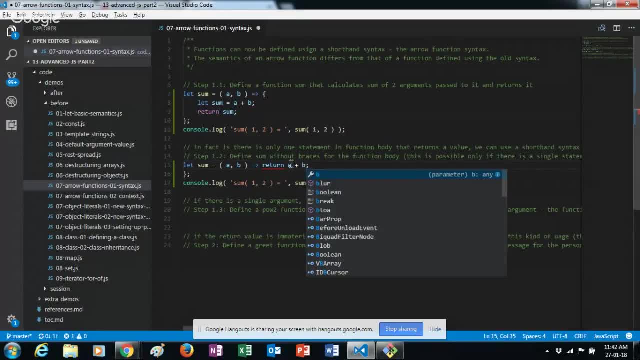 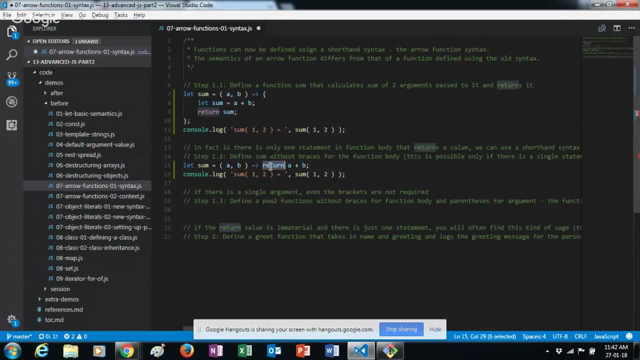 Okay, you could say: return A plus B. Single line function: body need not be enclosed within braces. Okay, this is perfectly fine. Sorry, you should not have a return value. So you just say A plus B. okay, So it accepts A and B and it returns A plus B. 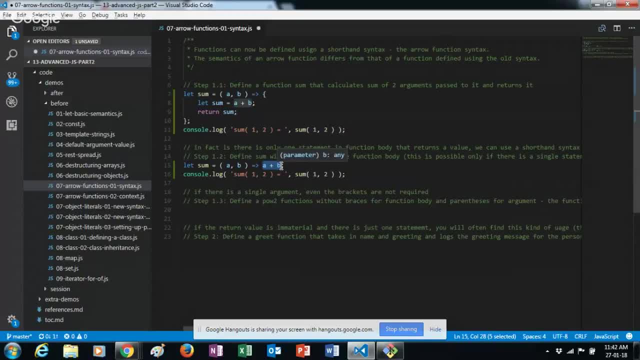 So even the return keyword is not. it should not be there. okay, In fact, it should not be there. So this is a simplified syntax. If your function body has just one, okay, return something. Return something, So okay. so that's the simplified syntax. 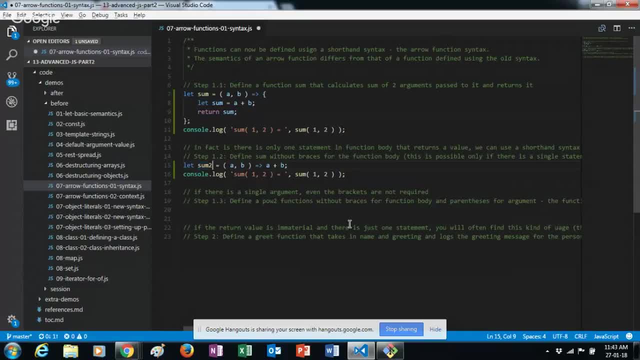 That's one more thing, And this sum would also work. I'll give it a different name, since it'll be a redefinition. So I'll say: this is sum two. Okay, and let's execute sum two and check whether it works. 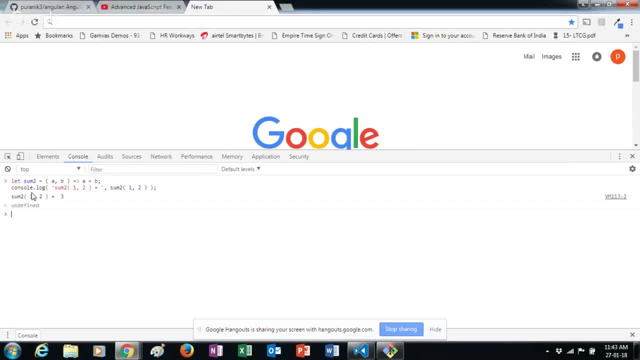 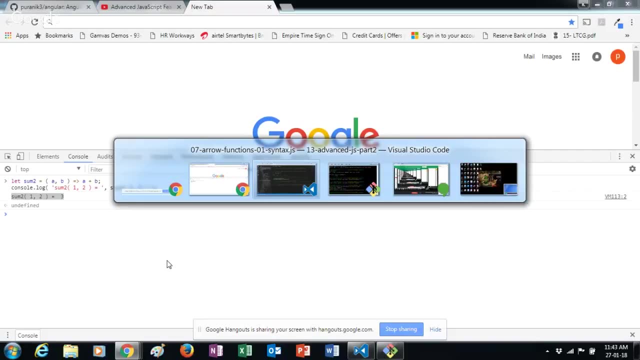 I'm not executing in the nodejs console, I'm just using the browser's console. You can see: sum of one two is three. So sum two of one two is three. So it works fine. So this is Now, if there is a single argument also. 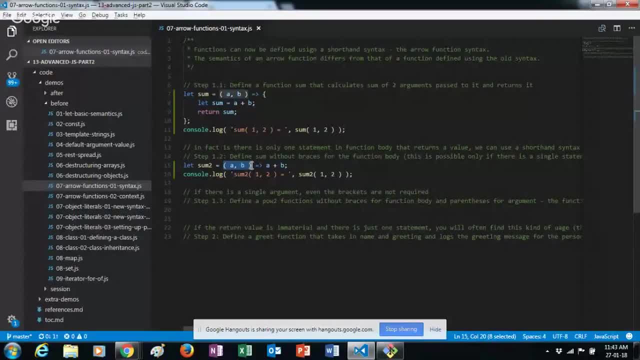 for example, there is instead of two arguments just one argument A. Let's say we have a square function or a power two function. It accepts a number and raises two to that number and returns the value, So that time you can have a further simplified function. 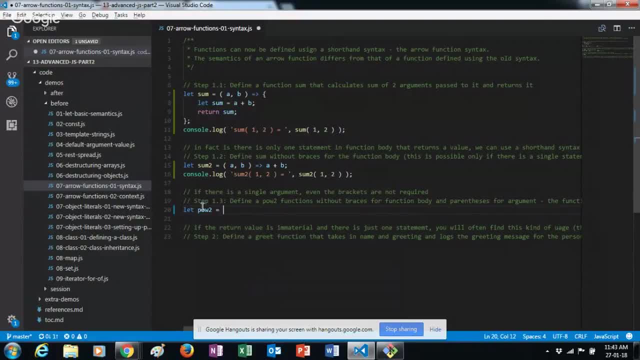 For example, let power two equals. okay, it accepts A and it returns matpower. sorry, and it returns matpower two raised to that number A. Okay, I'll call it N instead of A or E exponent, all right. 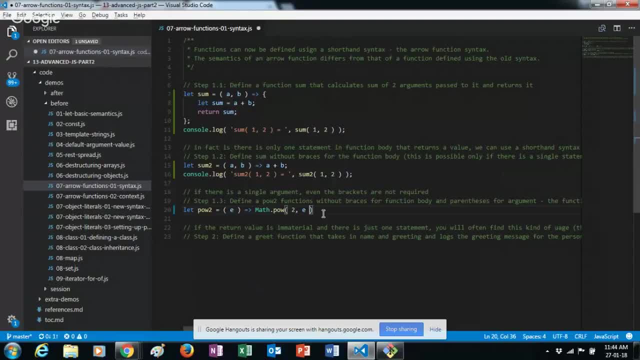 Two raised to that exponent. So of course, this could be done, no problem. Okay, syntax is perfectly okay and it would work. also, Let's say 10, power two of, let's say 10.. Two raised to 10 is 1,024,, power two 10, and this would work. 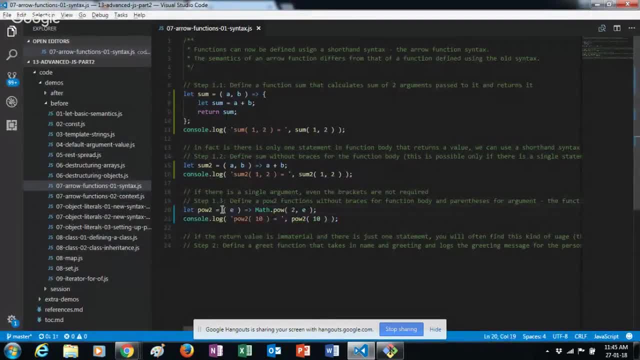 It works. Syntax has nothing wrong. But if there is just a single argument, the brackets are also optional. The brackets around the arguments are also optional if there's a single argument. So since there's just one argument E, we can even remove this. 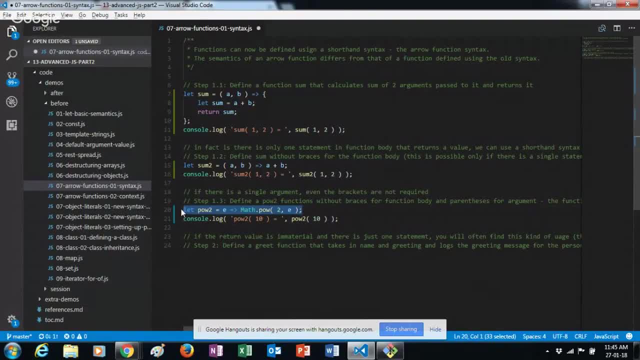 So it really simplifies the syntax, okay, But what it changes is also the semantics that we'll see next, So this will also work. Okay. now we already have something called power two, So probably I'll have to change the name there. 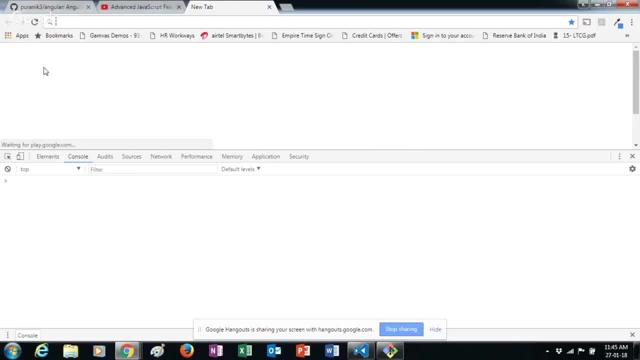 but or I can just refresh the page. So I'll just refresh the page so that global object power two is lost. Okay, So you can see that it's working. This syntax is also working, Okay. so if you have a single argument, 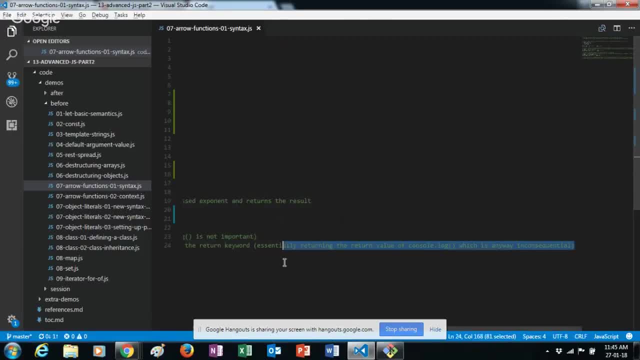 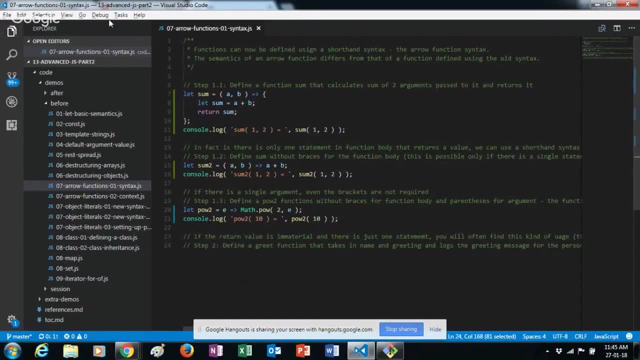 the brackets are not required. So that's one more thing, Okay, One more kind of usage that you'll usually see. okay is this kind of usage. You shouldn't get sort of unnerved by it. That's why I'm mentioning it. 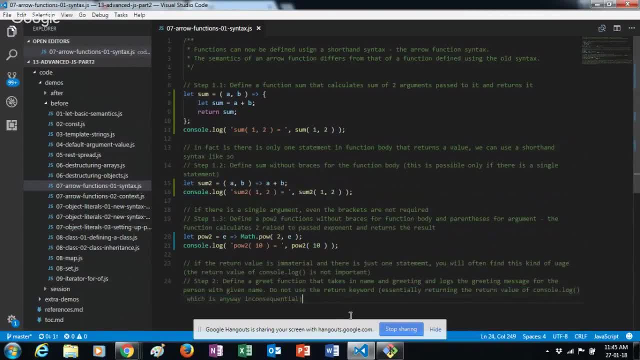 So let's see what that usage is. So you'll see that a lot of times people will do this Let okay, let's say there's a greeting function and the function basically takes a name and it wishes the person good morning. 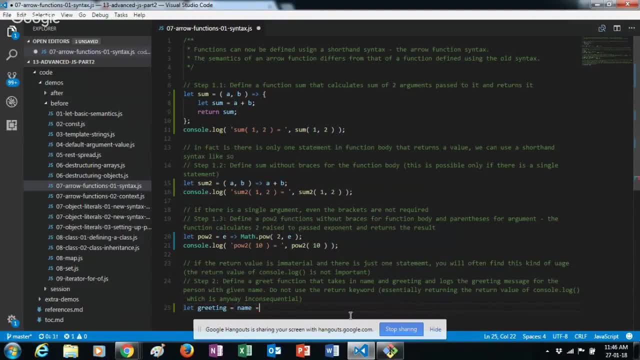 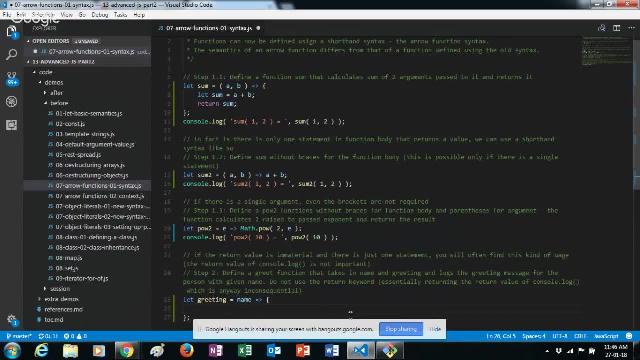 Okay. So let's say you would do something like this: Okay name. And then you don't want to return something, You just want to print. So you have a function body where you say: because if you just say like this, like we saw here, 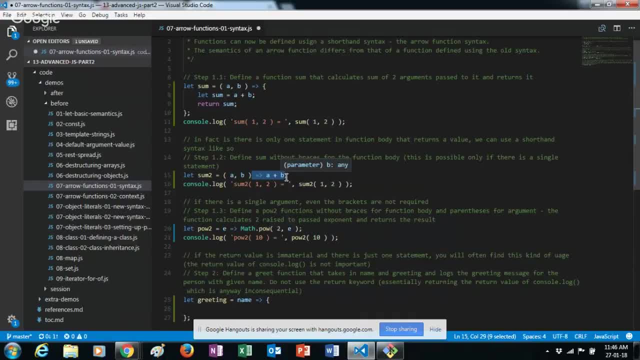 then A plus B is a return value. It is equivalent to the function body having the statement return A plus B. Okay, This one here, So greeting, equal to name. it accepts name and it returns, Let's say, name. It returns name plus, okay, say exclamation space. 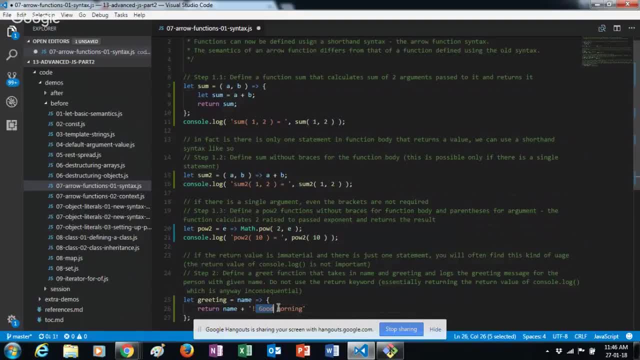 Good morning, Okay. Or let me put this in front: Good morning, Good morning, Good morning, Okay. Okay, All right, And then let's wait for a second, because it took some time. My keyboard is still bad. 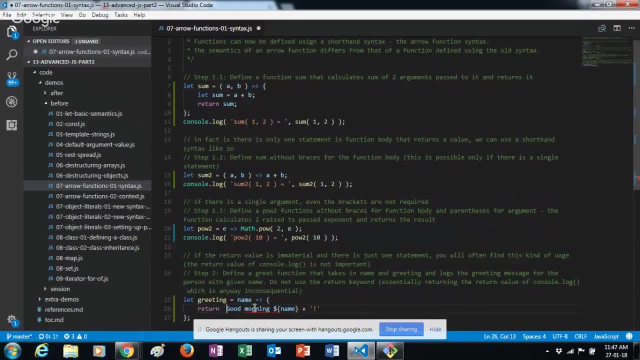 So ten minutes each. Now it's OK. Change Badge: Now I got a new changed, It's all right. And then this: or we could even use our templates index, which we saw last time. Okay, If you miss last webinar, you can look into it. 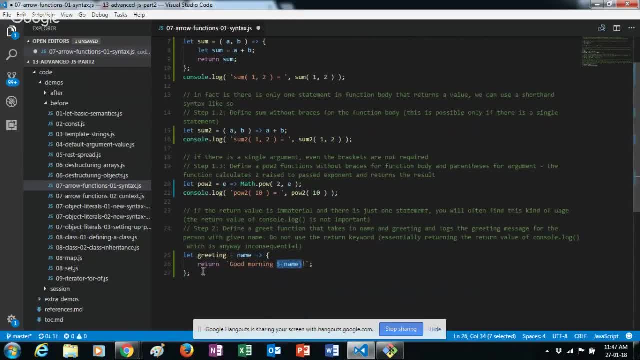 how it works, all right. so this would be a function that takes in a name and says: good morning that person. so let's try that out. so I'll say, okay, console dot log. okay, actually, let me do a console dot log here. it is, instead of returning, okay. 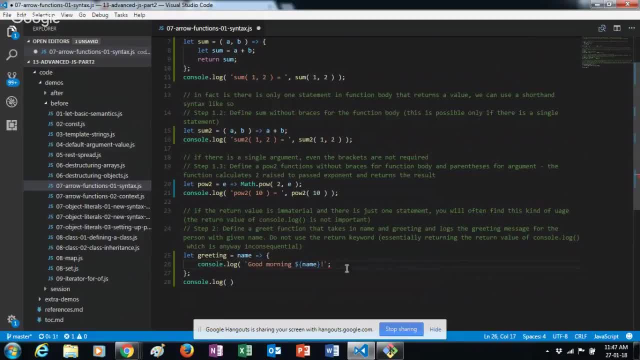 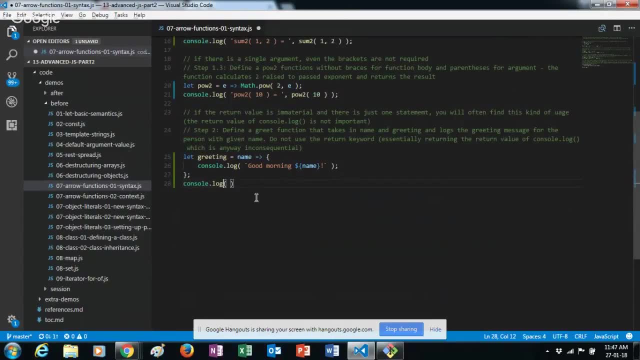 that's the point I want to show. actually, console dot log. okay, good morning John, or whatever, or is what. where is the thing pass? so let's say we call that function greeting, sorry, we call the function greeting and say John, right, so now it's going to print to the console, no doubt so if you run this. 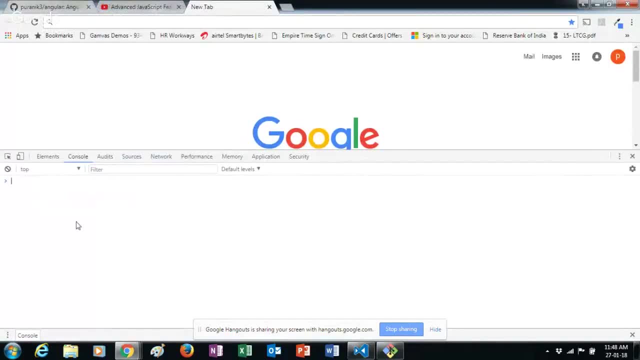 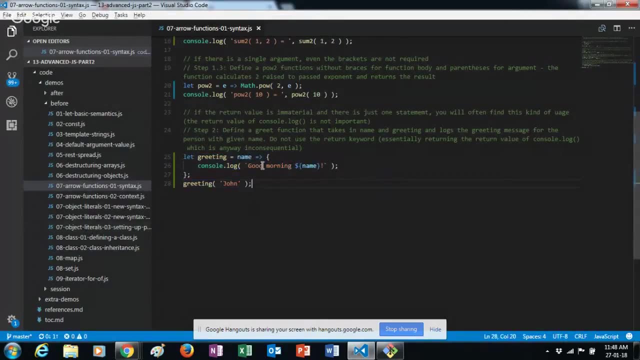 you see here: good morning John. it says: now you would also see people doing something like this. now, this is not returning any value in JavaScript of a function does not return any value by default: undefined. the value- special value undefined- is returned. okay, so you'll find many people using this kind. 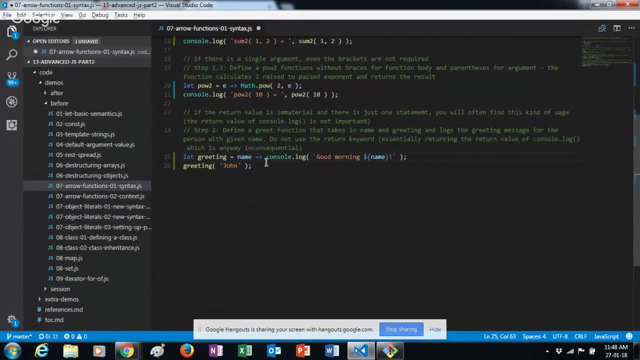 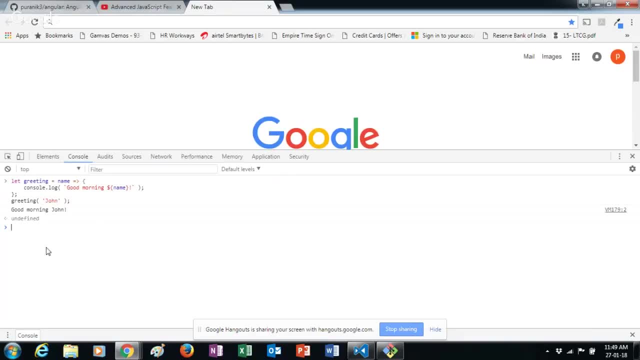 about what console dot log returns. okay, console dot log function as such will return undefined. okay, okay, so let's say you print out something, it'll return undefined. that's what you see here in this line. okay, it has logged FDH, FGF, and then it prints undefined. that's the console dot log. 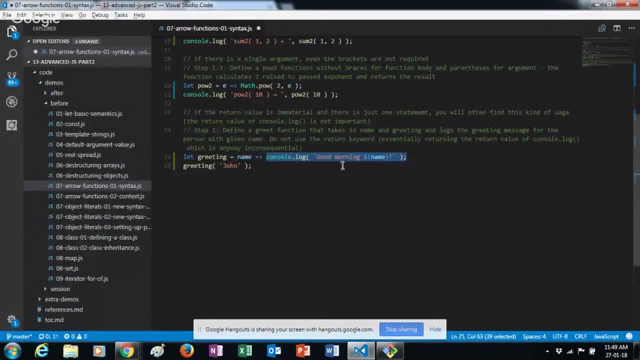 functions return value. now, it doesn't matter what console dot log returns, nobody cares, okay. so this: though this function returns undefined, it is doing what we want, which is logging on to the console. so many people use this shortened syntax. okay, without the braces, even if the return value of the function being 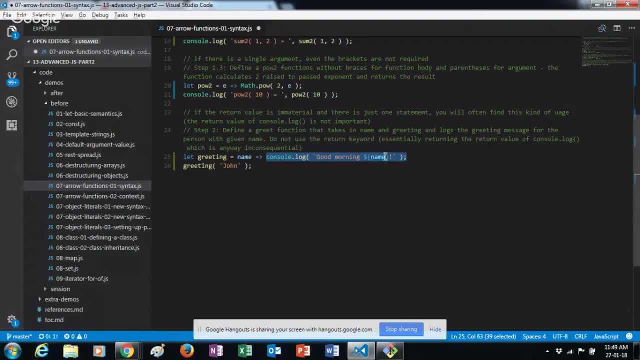 called at that point of time is immaterial, basically okay. so you will find this syntax being used like this. also, you shouldn't get put off, since it's not going to return what console dot log is doing. what it's returning, no, we don't care. it is of course, returning whatever console dot log returns, which. 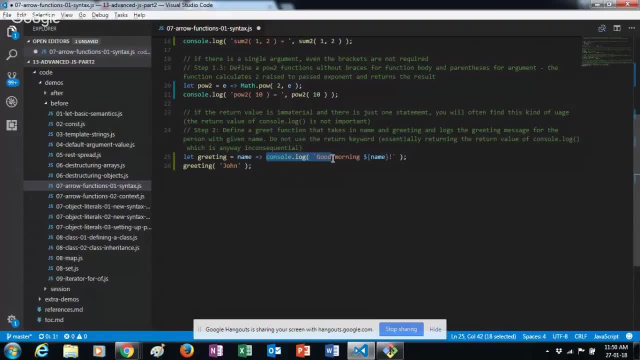 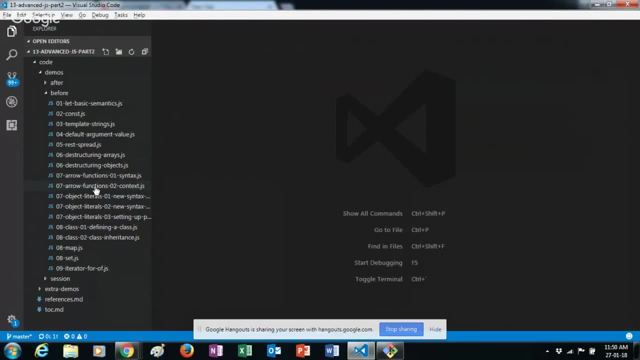 is undefined, but we don't care. greeting will return, also undefined, but we don't really care. all right, so this is short, so we use it. so that is basically the syntax of arrow functions. okay, if you have any questions, as I said, I'll take it towards the end of the session. so now, moving on to, I'll take all your questions, definitely. 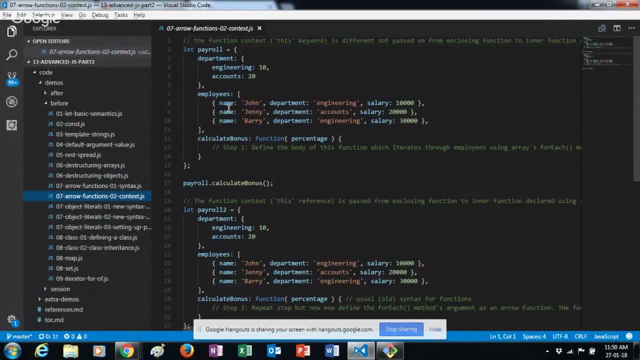 but in the interest of time, I'm doing it at the end. all right, so the semantics. how does it change them? now? this is a simple object written in es5 syntax, except that it's using the let keyword, which has three properties: Department, Employees and calculated bonus. Department is an object, all right. 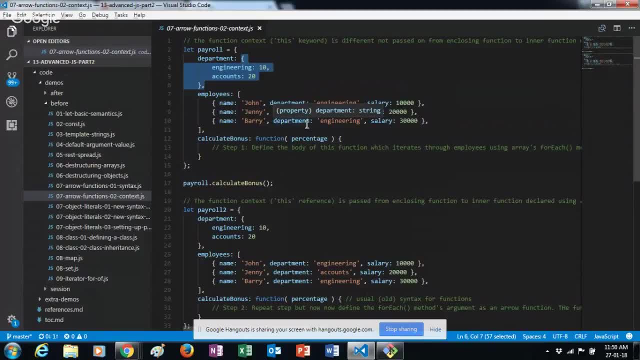 with two properties. again engineering 10 accounts 20. this represents the percentage bonus, let's say after the annual bonus is being given. let's say it's and the company has decided to give bonus. okay, this may seem very high percentages for companies these days. definitely they're trying to give this. 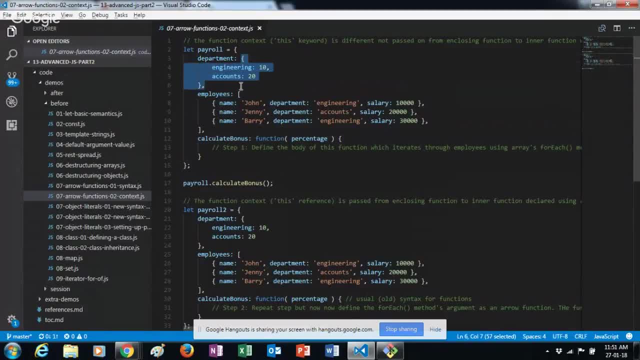 much. but let's say 10% for engineering, 20% for accounts, and these are the people in different in the company. let's say okay, so it's an array of objects. each object represents one person in the company, so the department the person belongs to is also there and the salary of the person is also there. so we need. 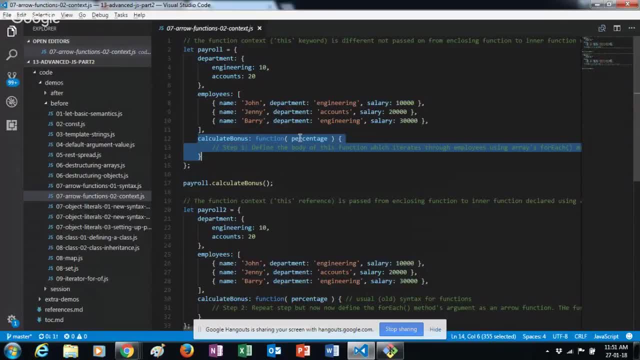 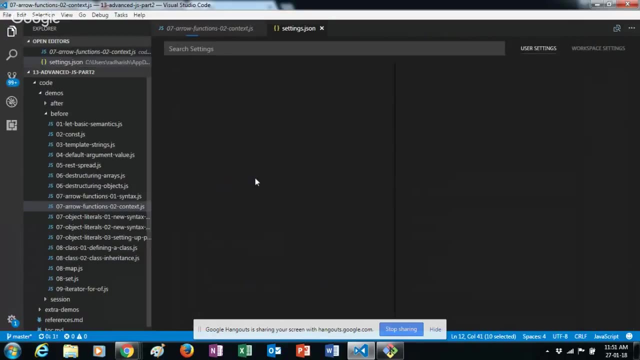 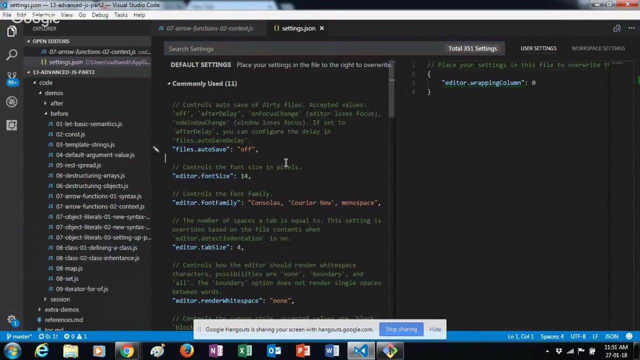 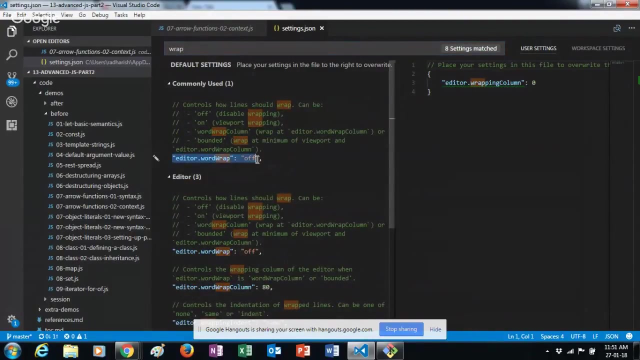 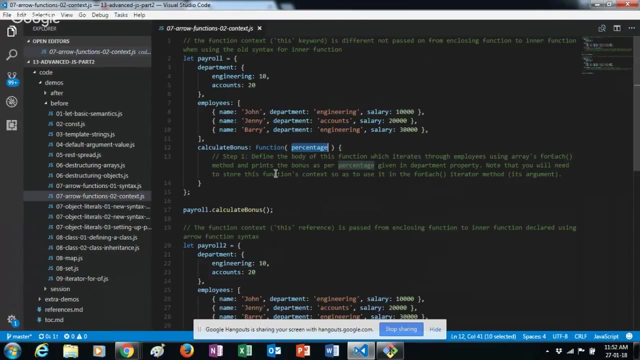 to write this calculate bonus method which will accept the percentage. okay, and let me just set some setting. I just wanted to wrap around. it's little difficult to read what I've written. so what we want to do is calculate bonus will iterate through the set of employees, the percentage and all, so it 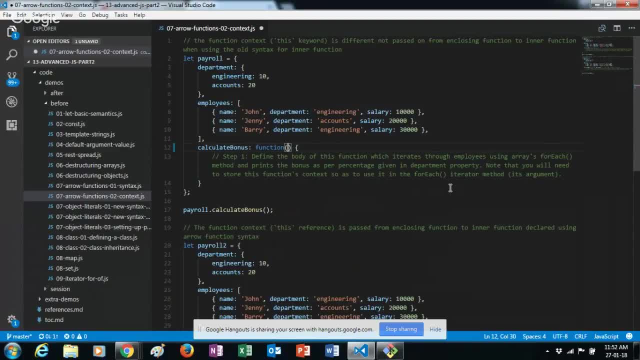 should it want to accept a simplified form with shall only the profit and we accidentally let's call hundreds of dollars and self current half. they can a mistake. so it should go through the list of employees, find out which department the employee belongs to and calculate the bonus. so, for example, uh, john belongs to department engineering salary. 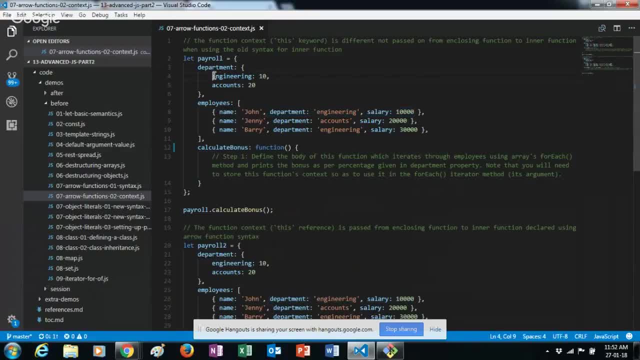 is ten thousand dollars, let's say: so, ten percent of that. okay, maybe it's christmas bonus, not diwali bonus, so ten percent of that would be thousand. all right, so that's what it needs to do. so you do something like this. let's say: if you do a for each, i'm using a for each specifically here. 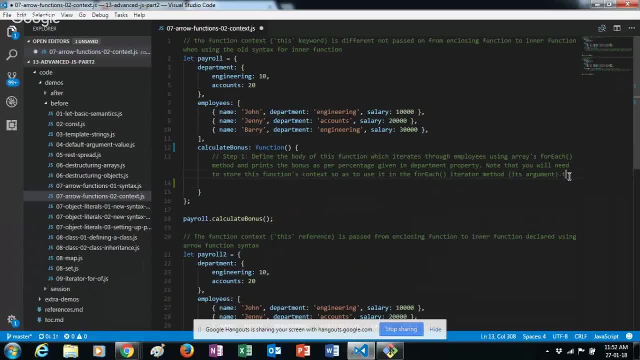 and not for a follow, for a specific reason. so we need to go through in this function here we need to go through the set of all uh employees, so this dot employees. this refers to the object itself, since they know its calculate bonus is a method of payroll. 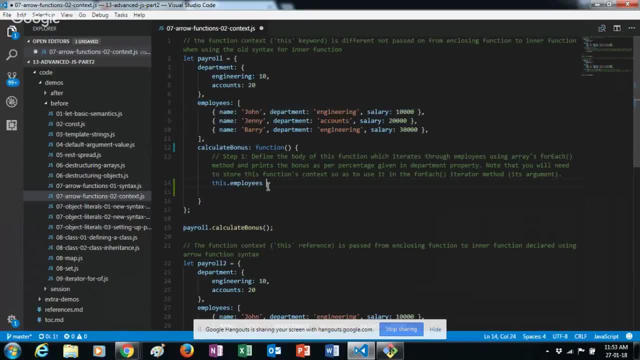 it'll basically be payroll dot employees. okay, so go through the employees for each. okay, i'm using the uh es5 for each, and then you need to pass a function to for each. okay, here again i'm assuming knowledge of for each. here there's an advanced, yes, uh webinar. so for each and it'll accept. 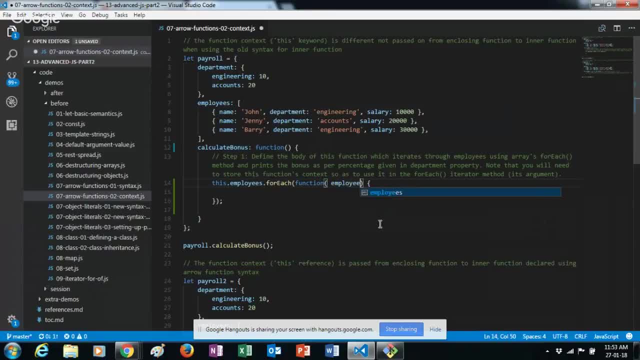 okay, it accepts many things. the first one would be the uh object itself, the item of the array, so the first one in the first iteration, and so on. so for every employee we need to calculate the bonus that would be the employee salary. okay, the item array, items, salary, property times. 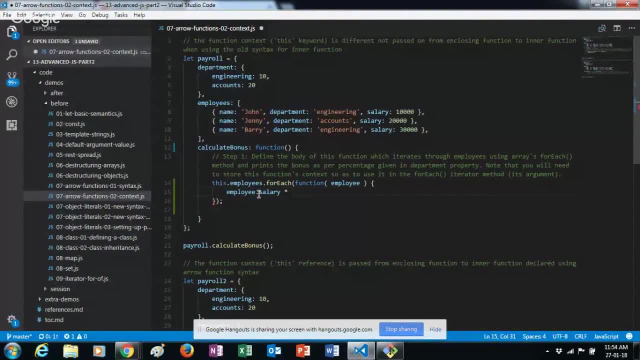 we need to find out what is the uh department. all right, so you may say, okay, this dot. this is a very common thing to say. so you may say this dot payroll. sorry, this dot department. and what is the department that would be the employees department, employee dot department. okay, so, basically, employee dot department would be that arrays. 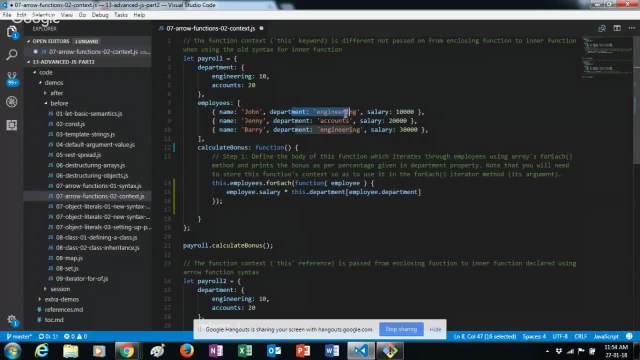 uh that arrays, uh, uh, this thing, that array items, uh department. then uh, this dot uh department would you would think that it would refer to payrolls, uh, payroll, uh department object, uh, whatever is the employees department. so that would give the uh percentage bonus for the department. all right, so you would think that this would calculate the 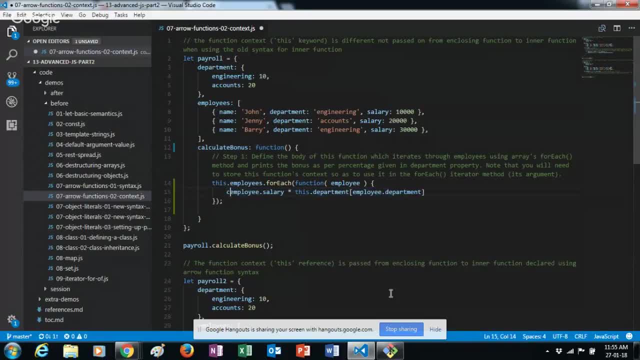 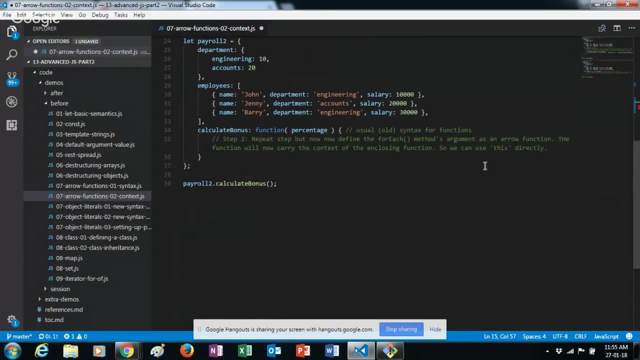 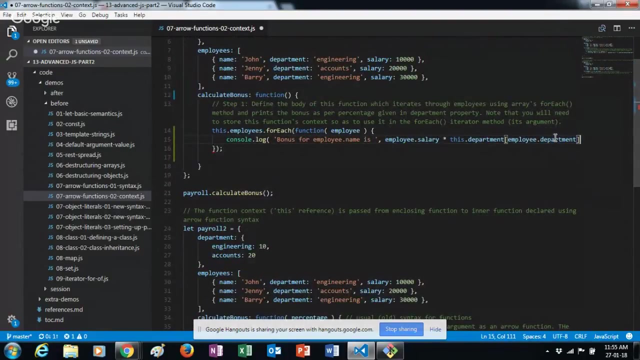 bonus for that employee. okay, so let's log that and see whether it really does. okay, so bonus for bonus for uh, let's say uh employee dot name is uh, employee dot salary times: okay, all right, so this is the thing. so let's see if this works, all right. 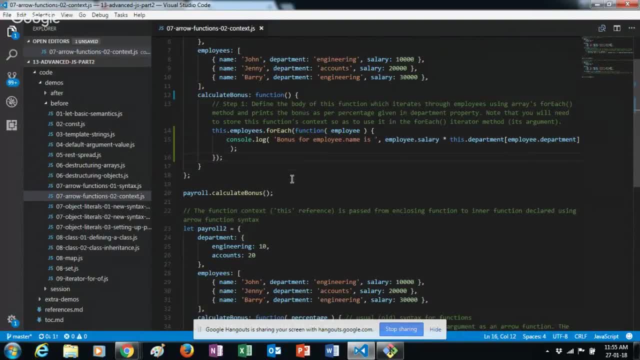 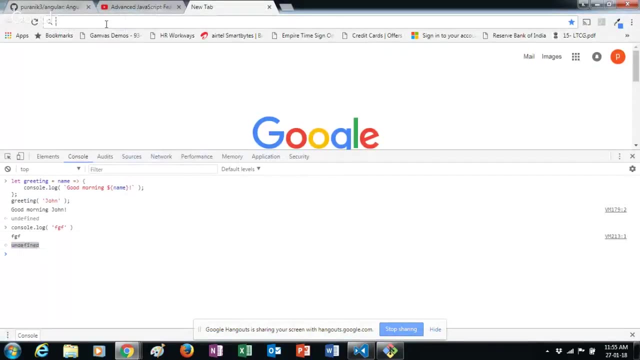 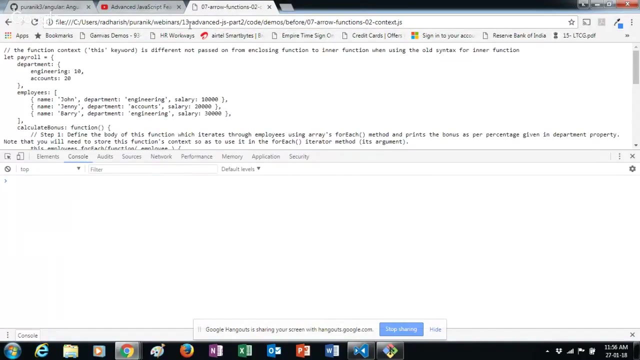 all right, so this is the thing. so let's see if this works. all right, all right, all right, let me run this. okay, so we have run this. all right, so now we have. oh, what have i done? but there's a js file. okay, so i have to run this in the console only. so 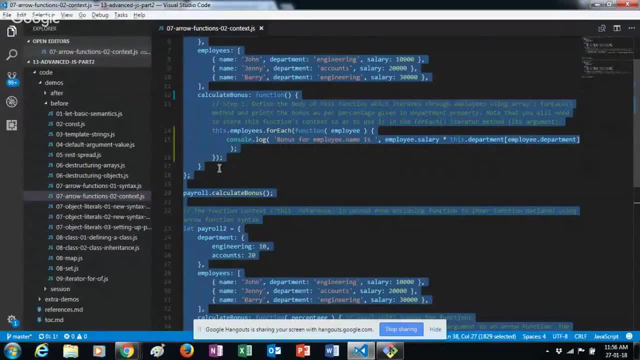 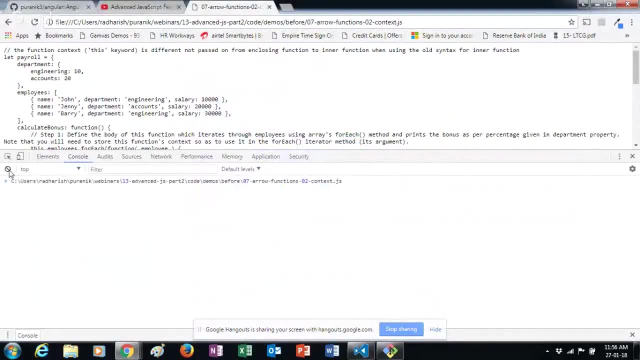 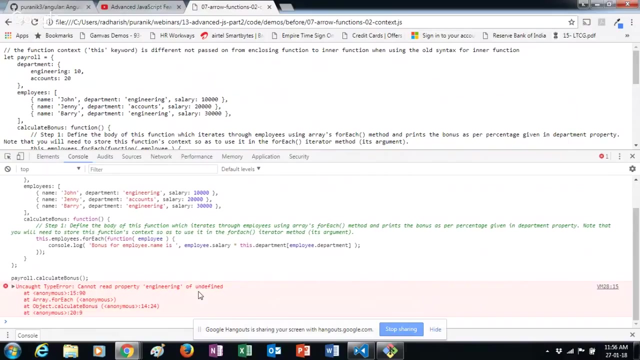 let me copy this entire thing, or let us do this: much only up to calculate bonus. all right, so you can see. here cannot read: property engineering of undefined. it says it's throwing an error. now what is the error here? so it's actually throwing an error at. 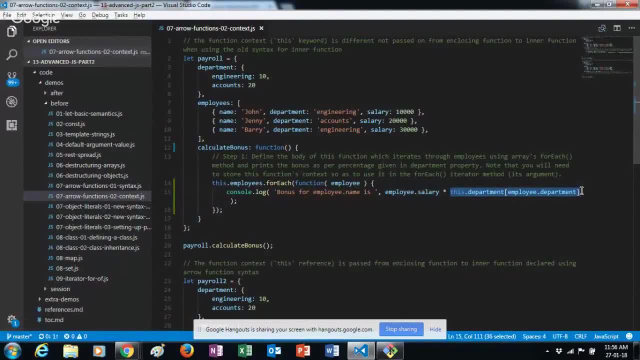 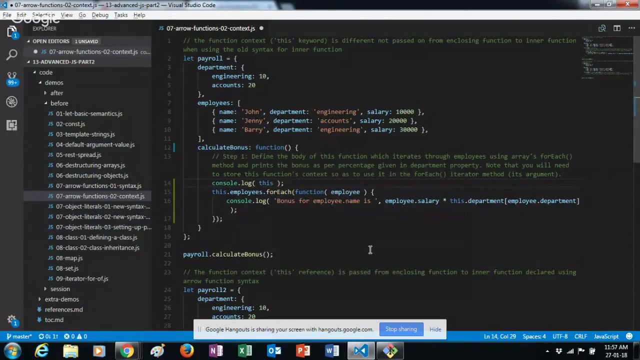 this point. okay, this dot department cannot read property, department of undefined. this seems to be undefined, or at least there's not. department is undefined, so this department is undefined. so the problem is that this in the calculate bonus function is different from the this. so the context of the calculate bonus function. 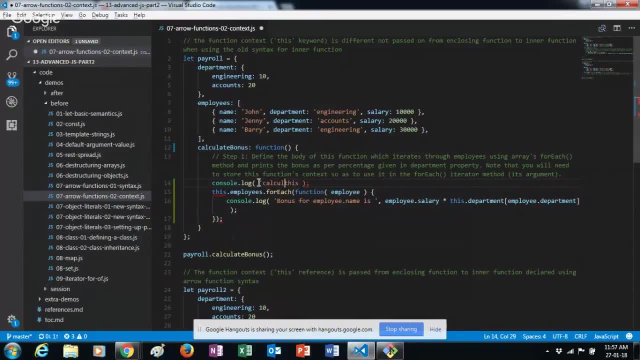 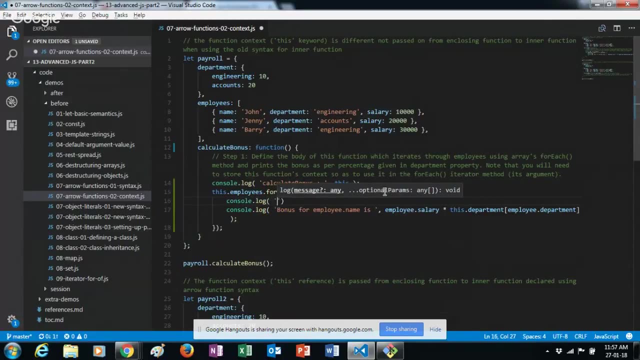 is different from this is the calculate bonus context bonus and this is the. this is the for each iterator methods. okay, this is a for each iterator function. this functions context. you'll see the two are different. okay, if you log that this here now. this is a well-known problem in JavaScript, so 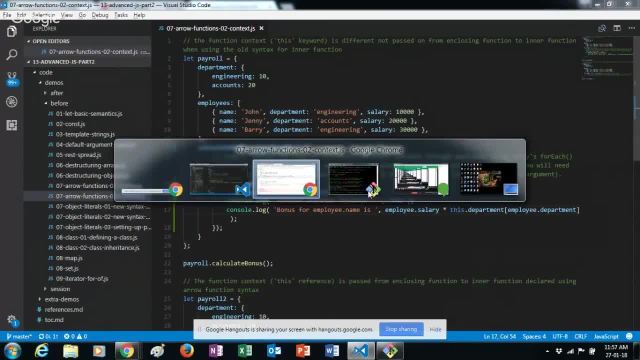 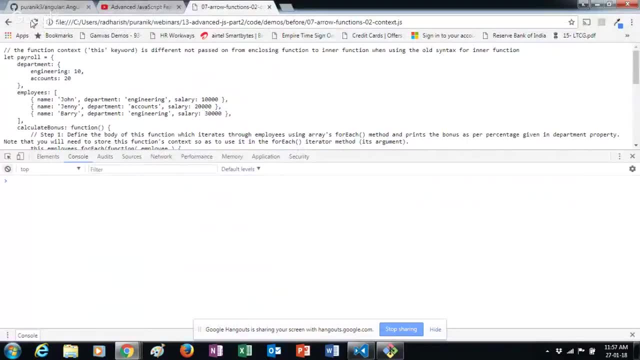 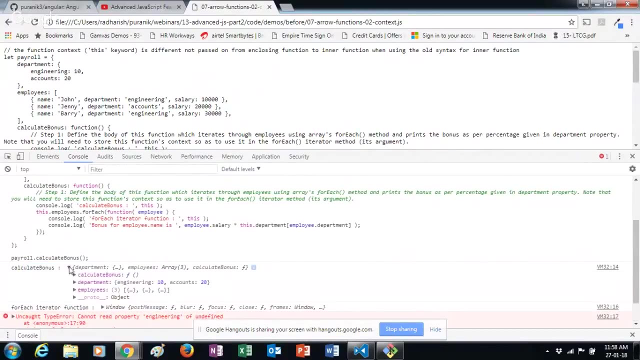 you as a well-known solution also, you just store the context, use it in the inner function. so now, if you see this, let me refresh. first see this: you see that the this here is: this is the payroll object, whereas this here is the window object. okay, in the second one is a window object for each method. 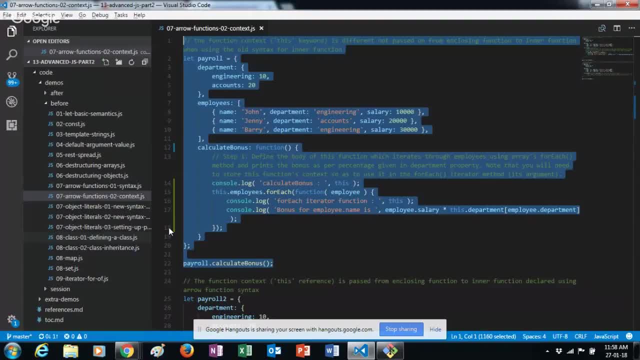 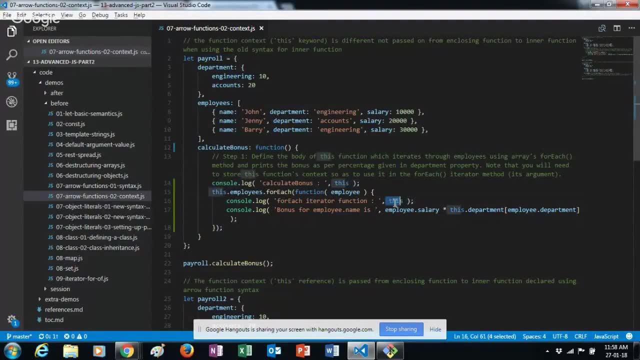 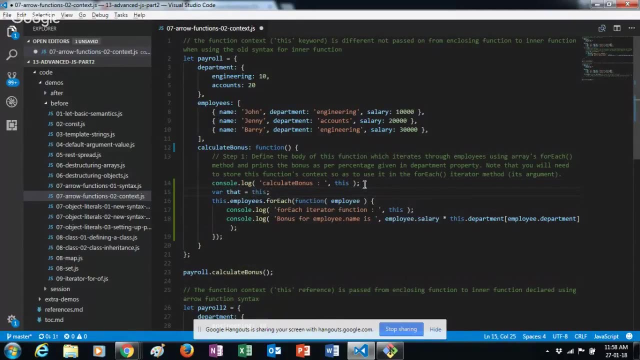 but in the calculate bonus. this refers to the payroll object. so this here refers to the payroll object, whereas this here refers to window. use this here, though. so well known solution for this is store it in some variable- let's call it that or self- those are common names- and then use that here instead of this. 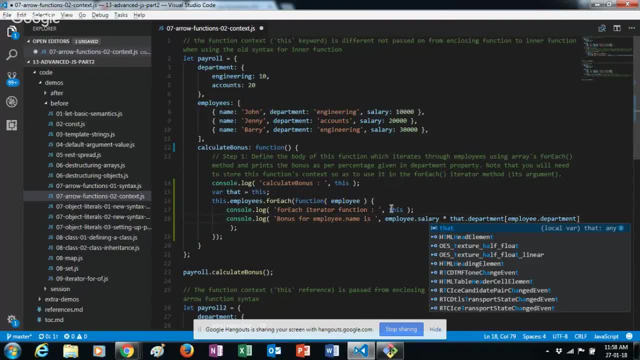 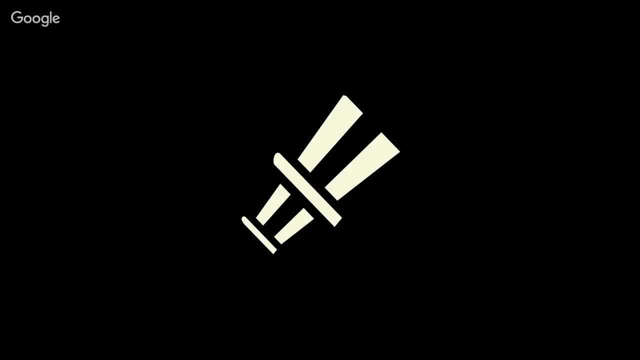 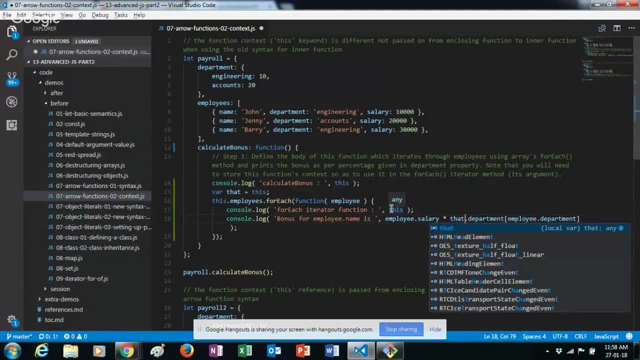 may not know about that. the function context is different. usually when you start up with JavaScript, you're not so experienced- it's very easy to make this mistake. okay, it's a very mistake that each and every one would have done at some point of time. right, it's the most common mistake, one of the most common. 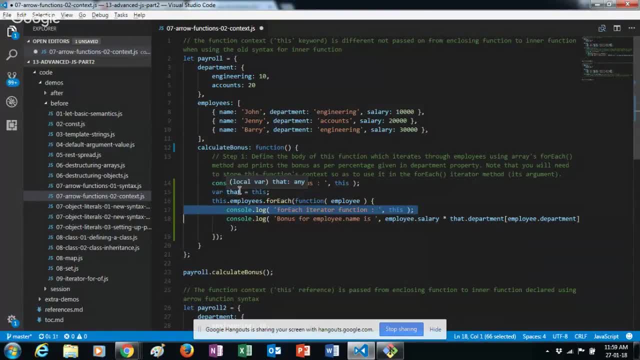 sticks in JavaScript. so to eliminate this kind of bug, okay, g-s 2015 has changed the semantics of arrow functions. so in an arrow function, the, the context gets passed on from the outer function to the inner function. so if you use arrow functions, okay, let's do the same with, so the inner function. okay, of course, this also could change. 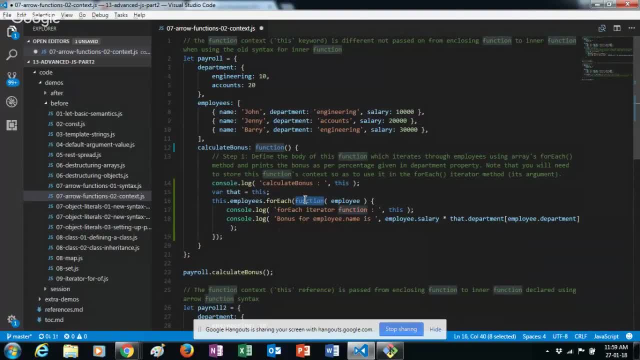 but it won't make any difference. but for the inner function, if you use arrow function syntax, so you say employee and then fat arrow. of course it's only a single, uh, single argument. so i don't even have to give brackets around employee argument. so employee it takes. 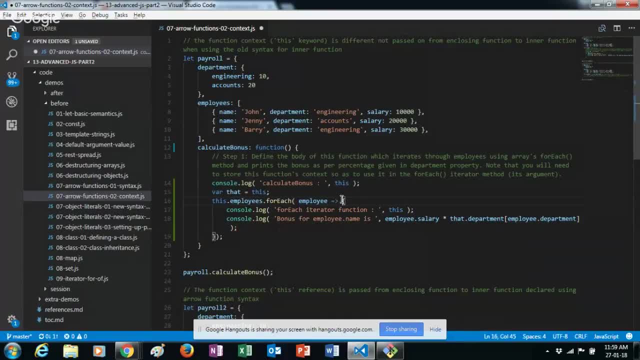 employee and it returns. sorry, and it does this. this is a function body, so it's a multi-line function body, so it does this. so now that this will can be used because the context of the outer function calculate bonus that this from the calculate bonus is passed down to the. this 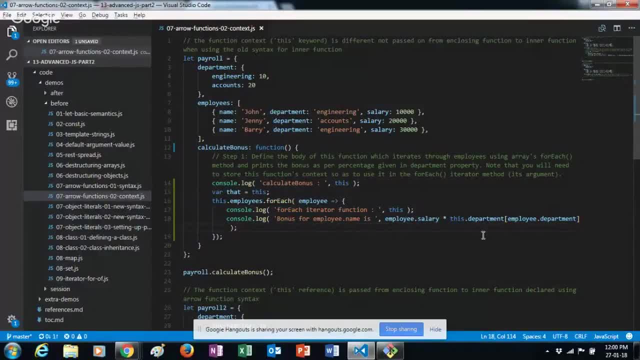 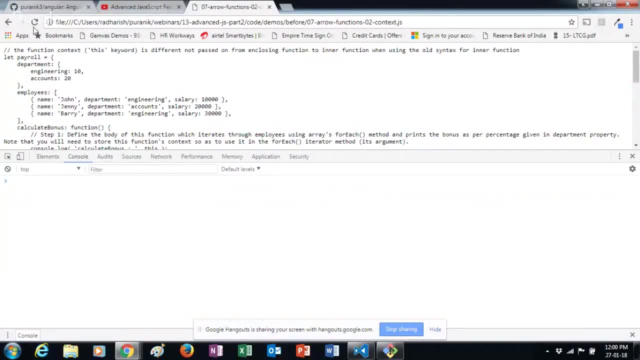 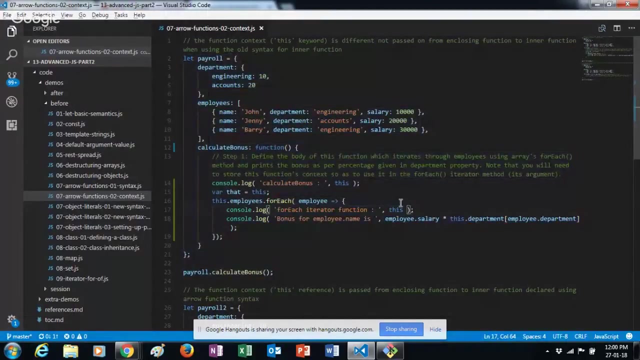 therefore, this will work. all right, let's execute this and confirm for ourselves. copy this: all right, and i have to refresh because i've used the let keyword. all right, so now you see it calculating perfectly okay. bonus for employee. this thing is so much for this thing and some of these things. i made a mistake in the thing. i didn't divide by 100. 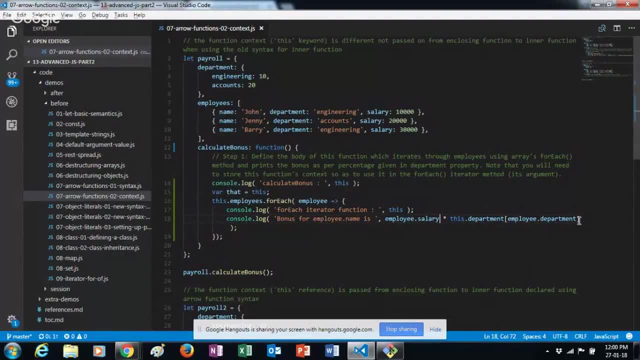 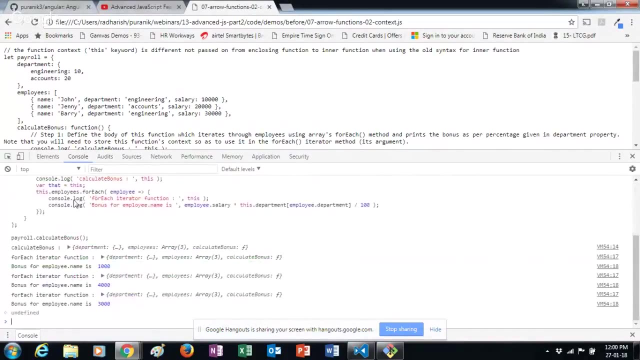 otherwise it's working perfectly okay. so into this, divided by 100, get the percentage. so all right, so it will work perfectly now. all right, so it's working perfectly. thousand rupees for- uh, i made some mistake again here, but that's okay. instead of the variable, i printed out employeename, all right. 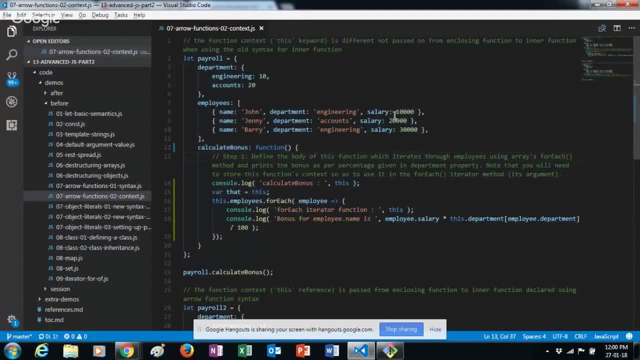 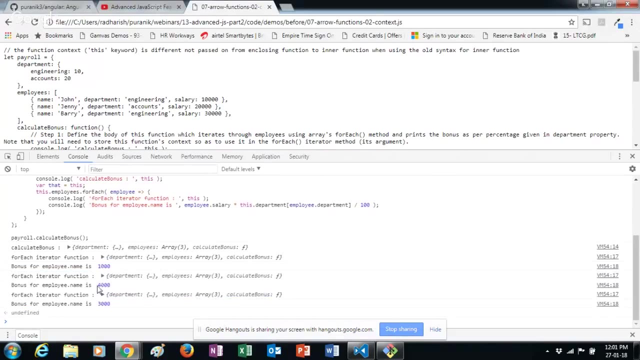 so the thousand, four thousand, three thousand, all right. so it's calculating perfectly. you can see here it used 20 percent, right, because this person is from accounts. so 10 percent is 2, 2 000.. 20 percent of that should be four thousand, and that's what it's done, all right. so the logic is: 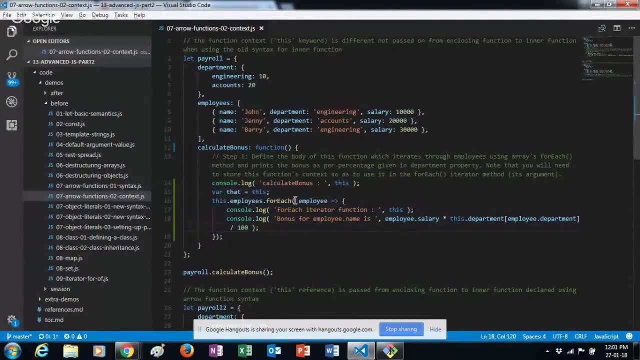 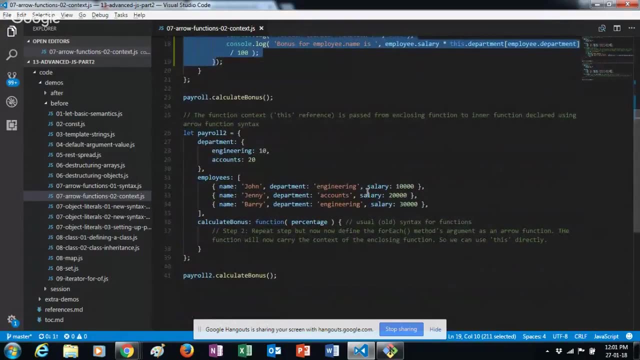 also fine, and the context is being passed, because we have used error function here. okay, so that's one way in which the semantics of error function is different from a normal function. okay, the use of av defined earlier. so that's one thing. all right, so the same thing has been repeated here. okay, that's what i just explained. 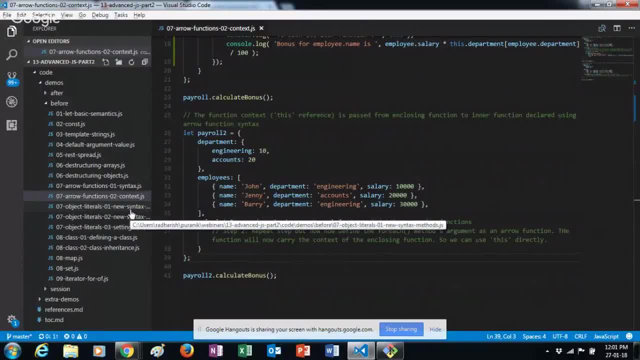 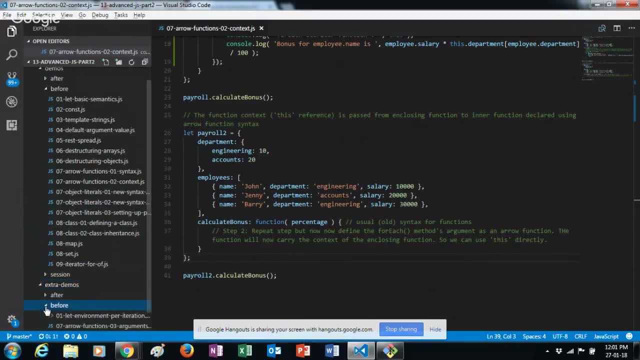 so there are other ways in which also the semantics changes. i'll just mention that. uh, that is an extra demo so you can try it out after the session if you want. by just following the steps, the arguments object is also passed from the outer function to an inner function defined using arrow syntax. 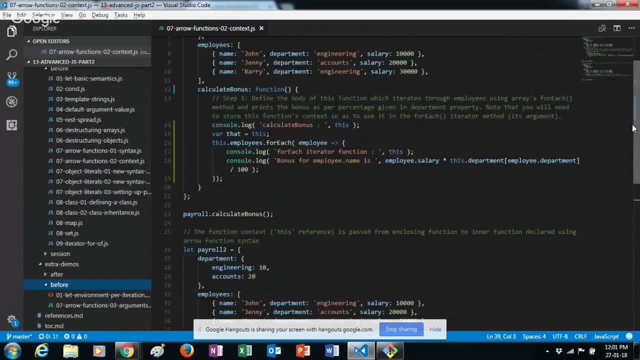 just like here, we define the inner function in the for each iterator, which is an inner function for calculate bonus method. okay, this is the inner function and this is the outer function. similarly, if you the arguments object will also be passed. okay, so if you consolelog arguments. 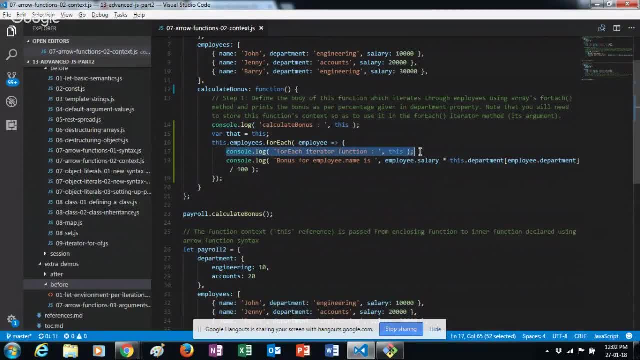 instead of this here and you consolelog arguments. here too, both of them will be one and the same. okay, the arguments. object is inherited, you can say sort of, by the inner function from the outer function, if the inner function is defined using arrow function syntax. okay, so the semantics. 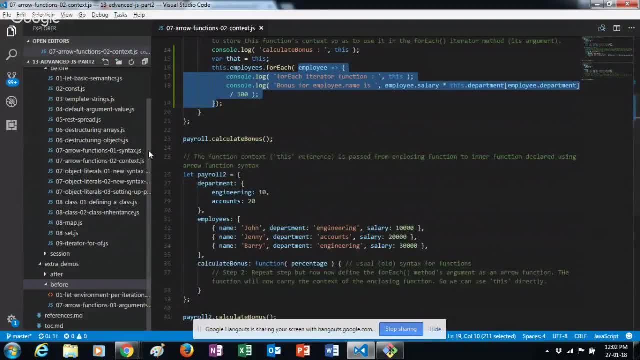 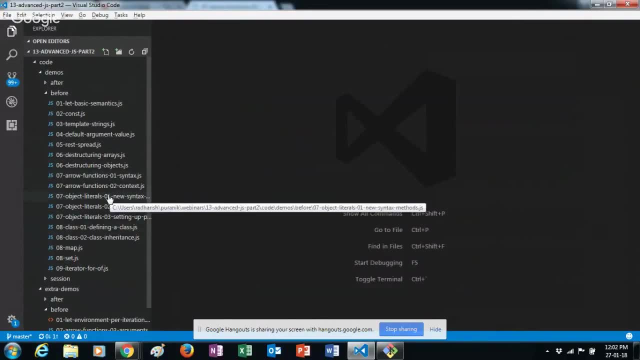 changes. so that's one more way in which it changes. okay, but i'm not going to deal with that. you can, uh, you can, explore that as an extra demo for that. all right, so let's move on to the next topic, uh, which is basically rest and spread. okay, this i had not called last time, because there is an arrow. 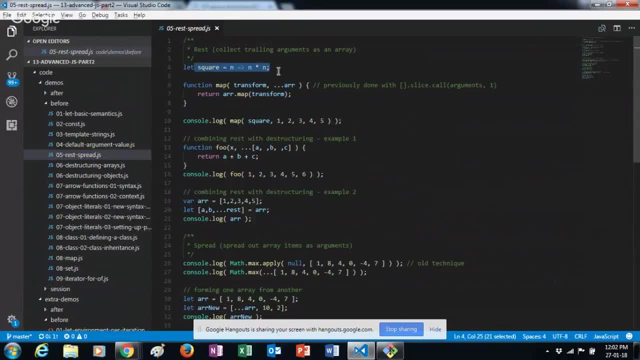 function syntax being used here. all right, so now we understand the syntax very well. this is a function that accepts a number and it returns the square of the number. all right, n into n. now, this is a function map. all right, and we had actually seen this last time too. 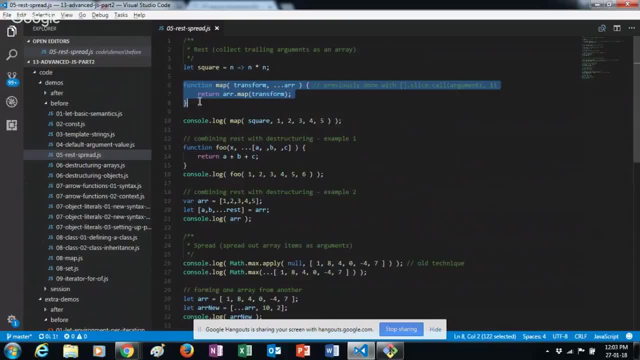 so i'm not going to repeat it, i just refer you to webinar 1, where we had seen how the rest operator works. so what we have done here is we have defined a function called map, which will take a function as its first argument. in javascript you can pass. 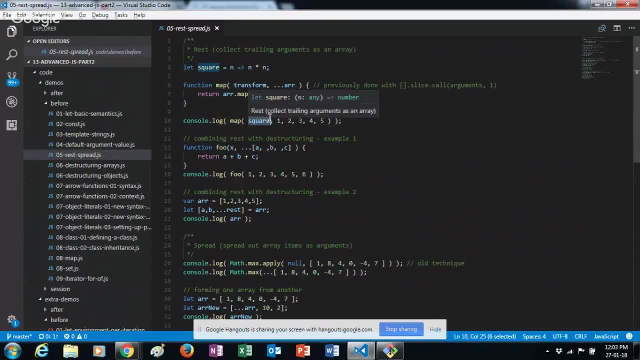 functions to other functions. so map is accepting a function- square- just like for each that we saw. now it accepted a function. so map accepts a function as a first argument- square- and then numbers after it, any number of numbers. so what it will do is it will actually perform. 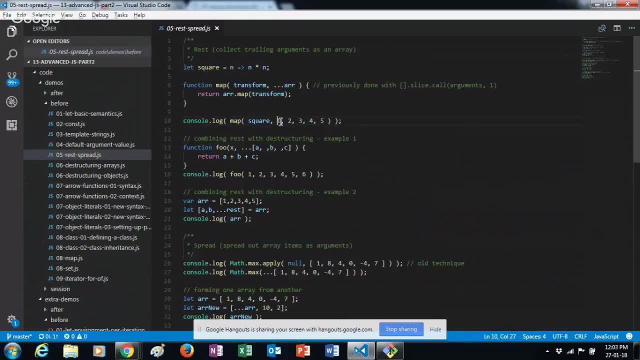 uh, it will return a new array where, for each of these items- okay, after the first argument, that is, each of these items- the square of that number will be in the array. all right, so you might write something like this, a function you might have written before, like this: uh, like this actually. 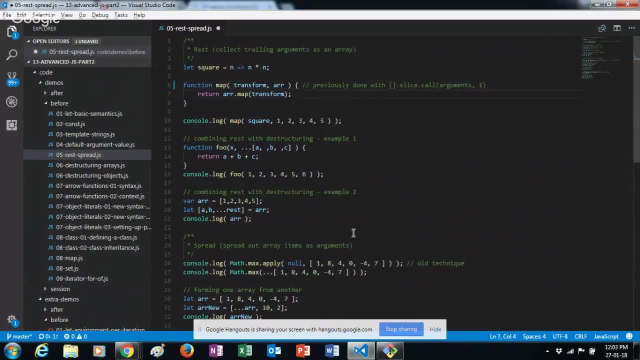 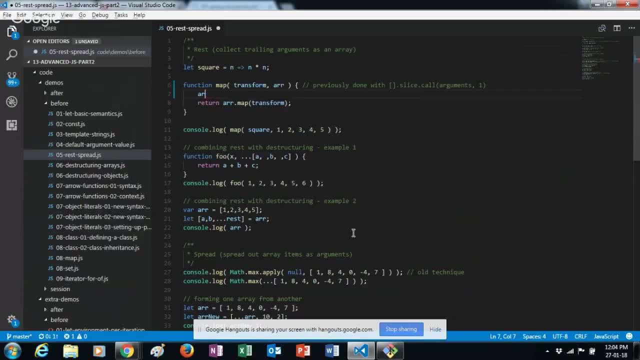 okay, this is. i'm just repeating from last time, so i'm not stressing too much. i want to go ahead instead of dwelling on this. so, array, you would earlier have done something like this. first of all, i'm not going to explain this again, because this is es20, uh, 11, that is es5, uh. you would have done something like this: array, dot. 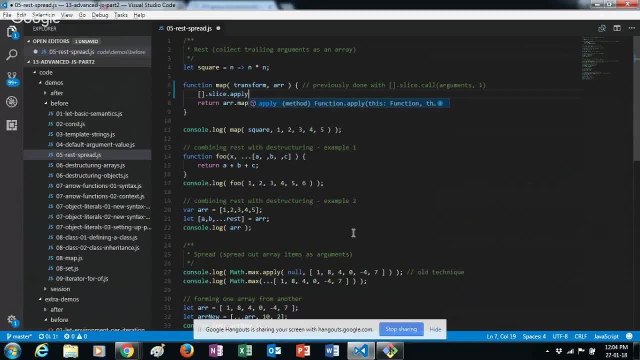 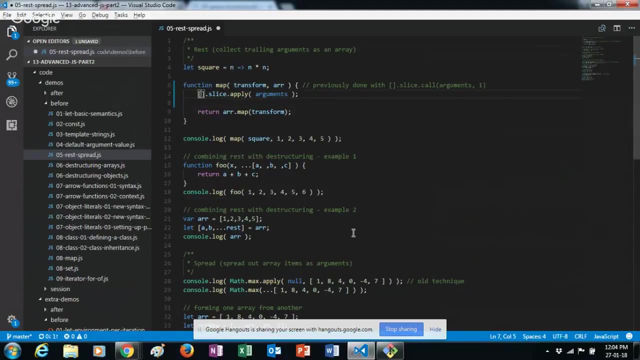 slice dot. uh, apply okay. uh, array dot. first of all, you would have taken a subset. you'd have taken a subset by saying: array dot, slice dot, apply arguments, okay, this would give the array. so if you see what this is, let numbers equals. you'll have to pass the context which would then be required in this case. so null come arguments. 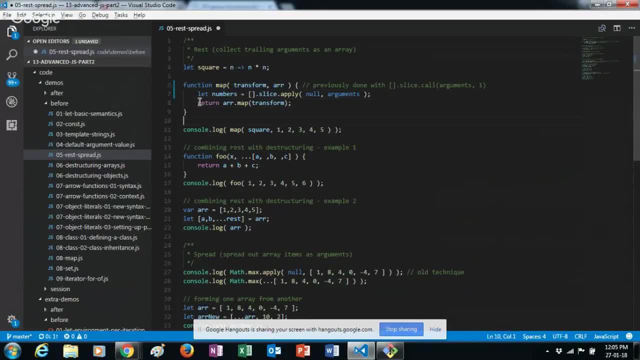 okay, and then let me comment this: this i've explained in the last webinar so you can refer to the last time. so, um, and then call this function like this: okay, so let's see if this is working. first of all, so it should print out this numbers. let's say i'll return number. sorry, first, 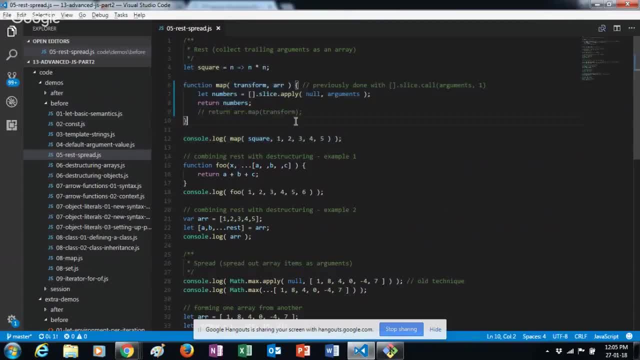 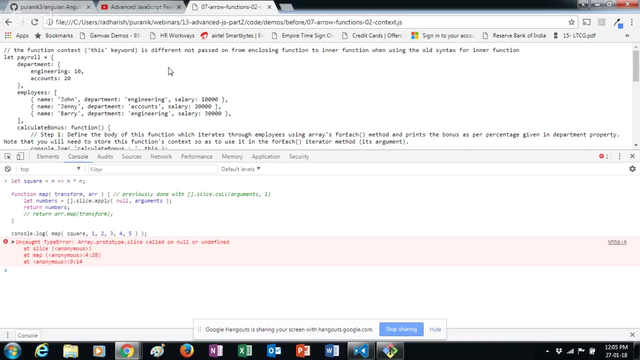 all right, all done. all on defined array. dot slice not apply. okay, it should be called on arguments. sorry, it should be called on arguments and you'll pass the arguments to slice as okay. this is 20. there's the s5, so i'm not dwelling on that. you can probably check the net how it works. 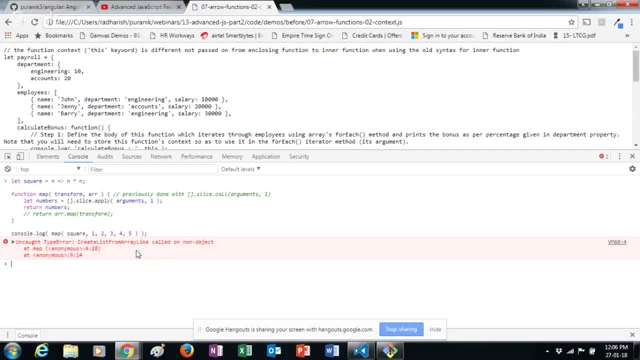 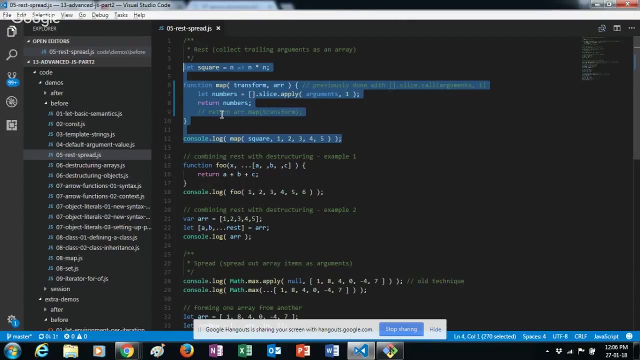 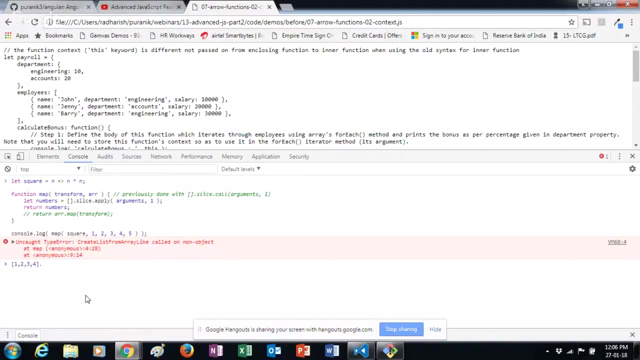 okay, create list from array like, uh, from array like, called on non-object array, dot slice not applying arguments function, so so, so, so, so also. so sorry, i have let me just check some things. so so i'm just creating an array like object. array like object is nothing but an object whose. 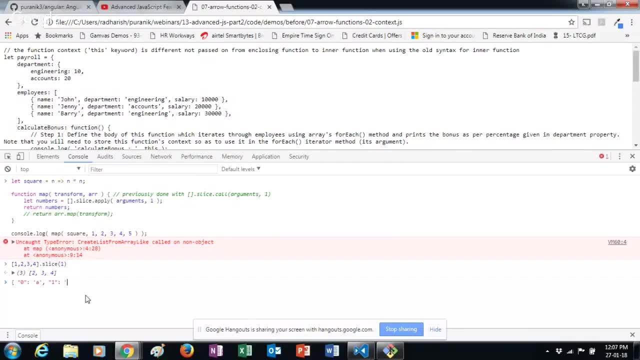 indexes are numbers 0, 1 and so on, and you can see 0, 1 i'm using, and which has a length property which will hold, uh, the total number of items, so two in this case. okay, let me store this in some object. okay, so if we say array, dot, slice, dot, apply on this obj, and let's say one, 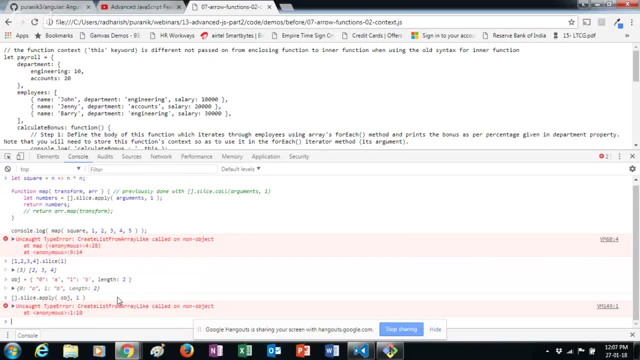 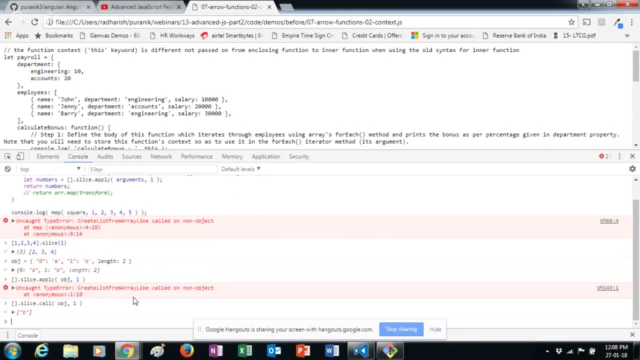 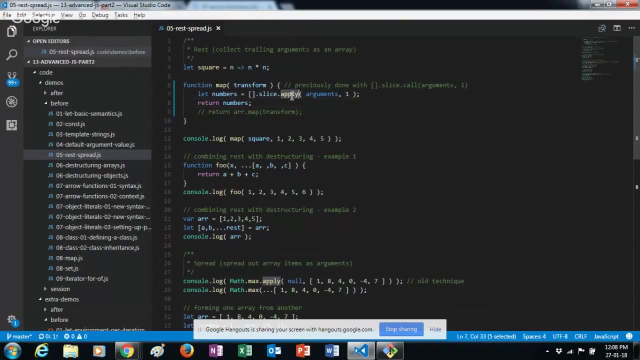 same thing comes. okay, hurry, dot, slice, dot, apply on the onion, all works. why doesn't work? okay, because i'm passing actual arguments, not an areas argument. okay, so i have to use call here. all right, because this thing here is not an array. okay, you'll use apply when you have an array as the uh, uh, an array having the arguments being passed. 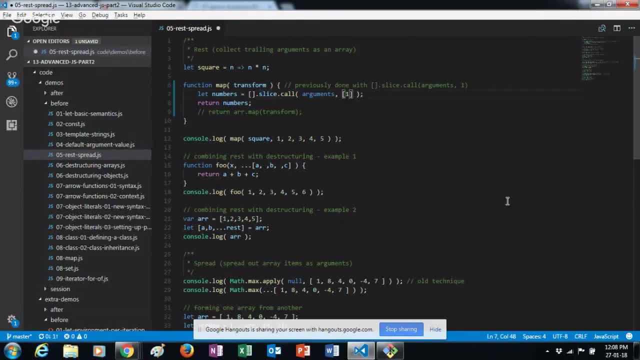 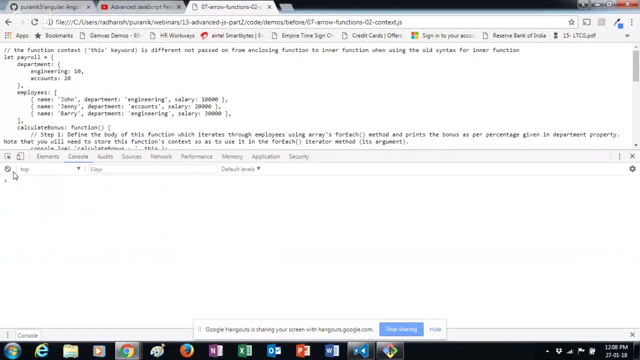 to the slice method. okay, this you can read up somewhere online if this is not comfortable. all right, so this will work. so this is going to return our uh square. okay, so i have to refresh because of the let. okay, you can see that it has actually got the 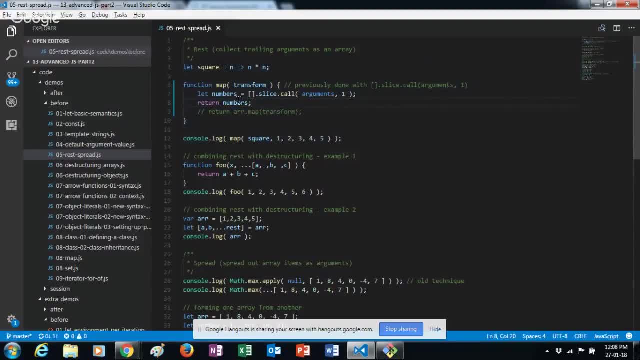 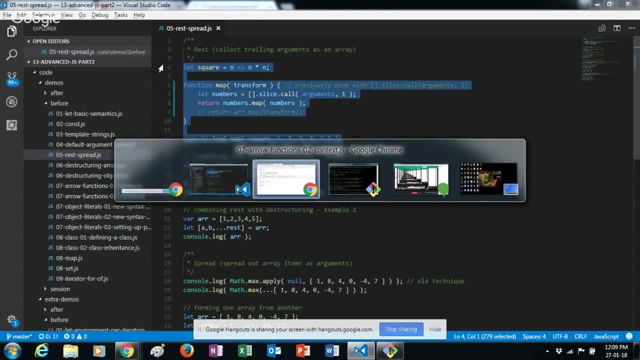 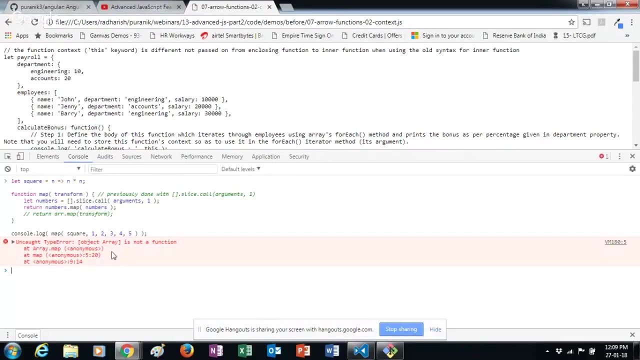 slice thing. now you can just return. you can. once you get the slicing, you can just say: okay, return numbers dot map instead. so map will return a new array where every item will be squared. all right, so this will do what we want. so we have a map. i missed out something. array is not a function. 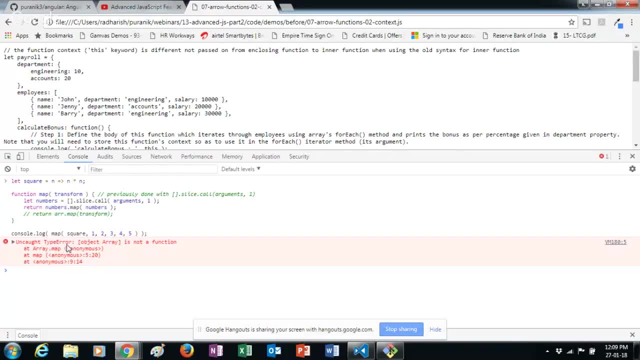 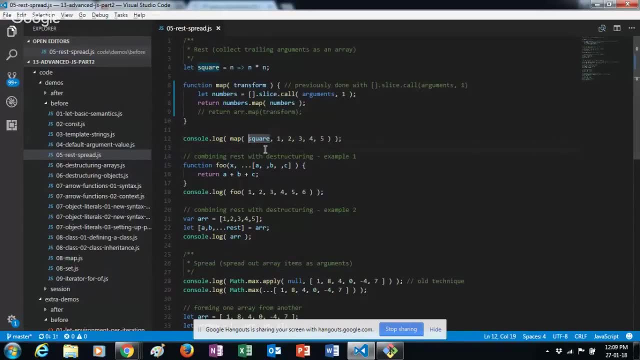 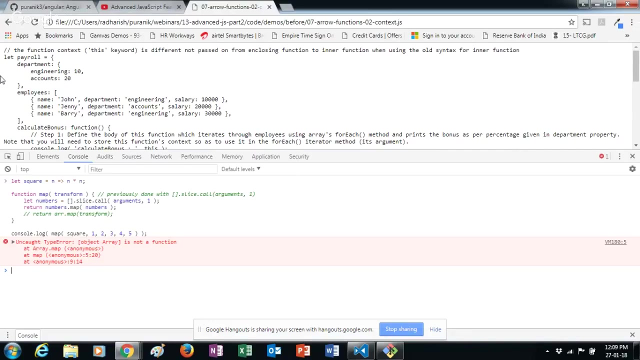 Har Discord. okay, so we'll whites the smoke and run some things. return numbers: okay, i may be doing some mistake here. map. i've called map here. this is a map, not numbers. transformation function will be the. I say yeah, okay, so we get an array where each of those items is transformed. it's become in the square. 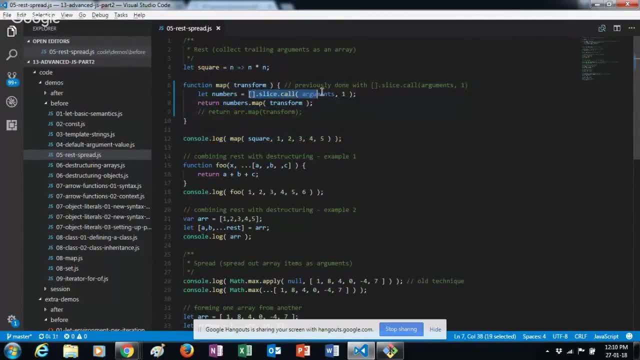 now, this definitely is. anybody who is learning JavaScript will get put off by such a syntax. okay, now what's happening here? we are not getting into the details of this, but JavaScript is 2015, has something called the rest feature, which will simplify this. all we want is whatever is passed after the first. 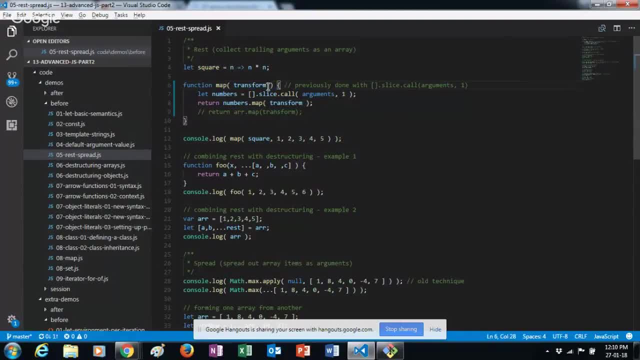 argument. we are not even holding them in variables here. okay, we are not even holding them. we are using the arguments array instead, which will hold all the arguments passed at runtime. we want to omit the first one, which is actually a function, and then take only the remaining the rest of the arguments- okay. 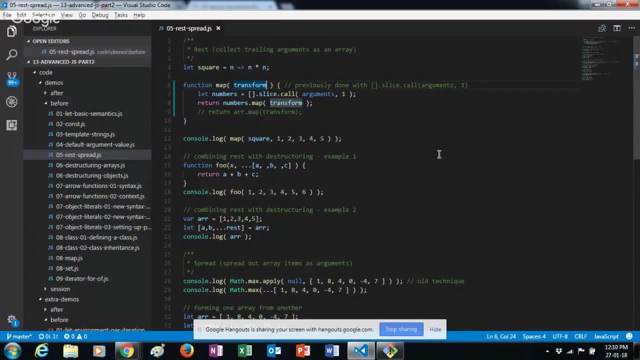 rest of the arguments. so what you can do is you can give the rest operator here. so after the first one, dot, dot, dot and call it whatever you want. let's call it numbers. so what will happen is when this map function gets called, the first argument goes into transform. copy to transform. 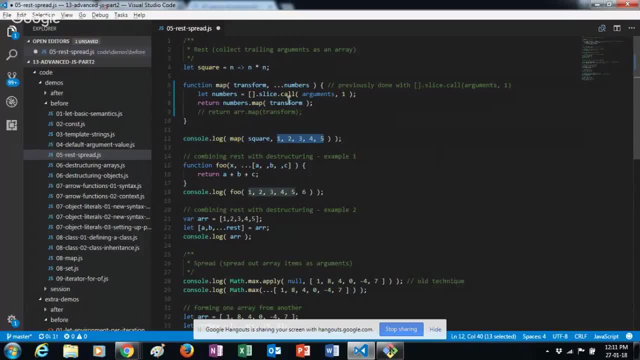 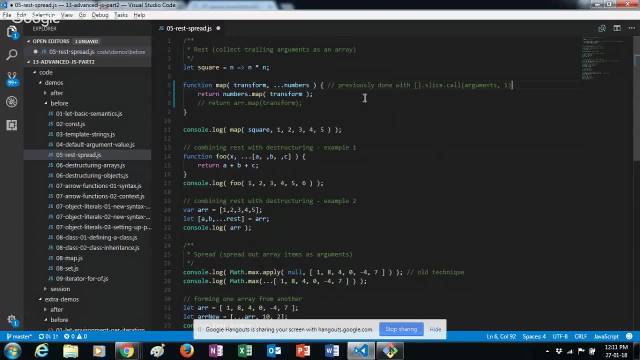 the rest of the arguments are collected into an array which is going to be called numbers. so this means the rest collected into an array called numbers. it's as simple as that. so now what you have, you don't require to do any of this in the stuff. 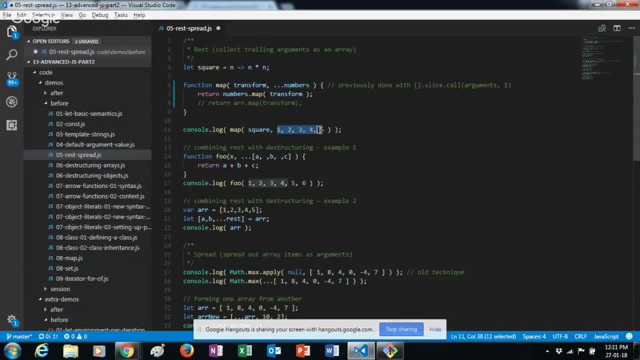 all you need to do is numbers is already an array which is going to be having the items, or now the items one, two, three, four, five, numbers, dot, map transfer. that's it, as simple as that. and since this is returning, you can further. if you're going to use something like your arrow syntax, you just say: okay, let map. 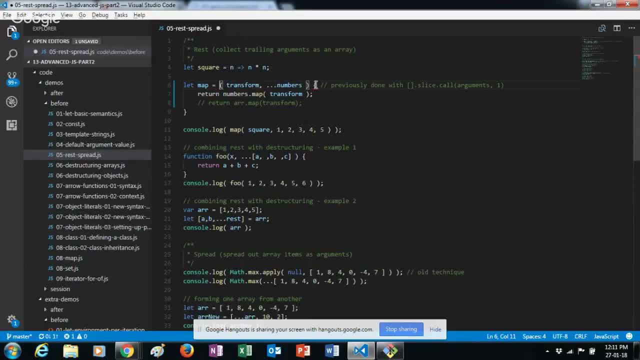 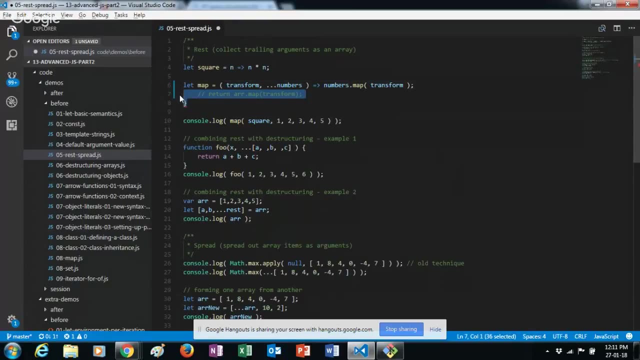 equals. okay, transform, and it accepts one transform argument and the rest you collect into an array called numbers and return. it's a single thing, so you don't require the interpreter. so you see how much it has simplified. not only it has simplified, not only as it reduce the 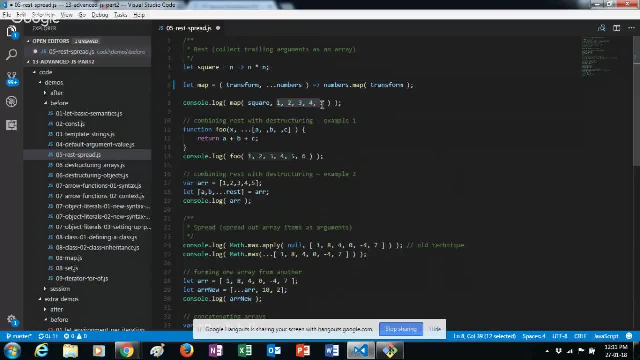 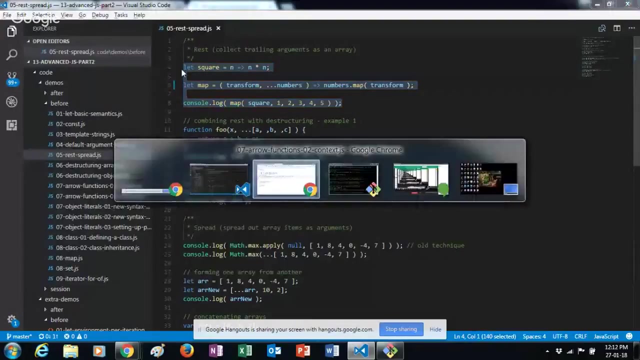 number of lines. it has really simplified because here you don't really have to use all that circus of array, dot slice, all that. okay, it's collected automatically in an array because you've used the rest operator, rest of the collection directly on it. all right, so as simple as that. so now, if you see, you can see that we are still. 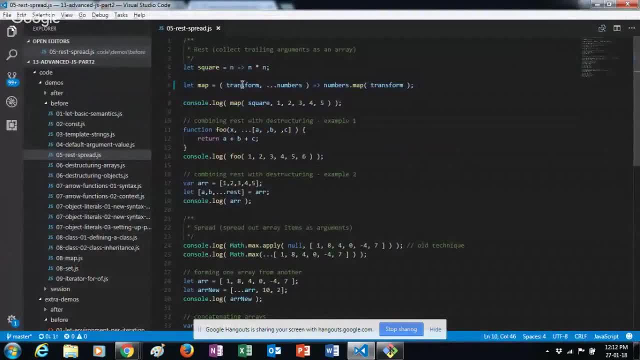 getting the same result. so that's the rest operator. so after whatever leading arguments, the fire, the training arguments, the whatever is training, if they are, they'll be collected into an array called numbers. so all these are collected into an array called numbers. so that's the rest of it. 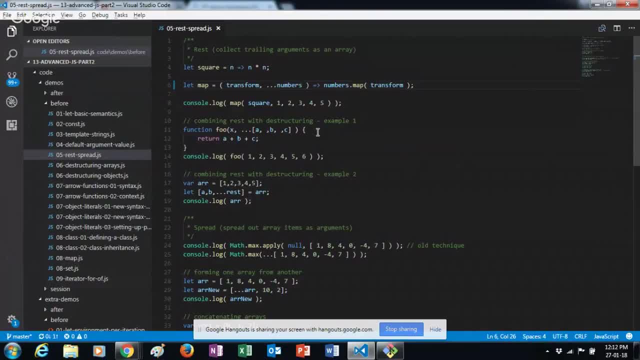 now you can combine rest with destructuring and all now we have already seen destructuring last time, so I refer you to that if you are not able to follow this. so let's say we have a function foo like this which is going to accept a lot of arguments. if you say X comma, so one will get copied to X when. 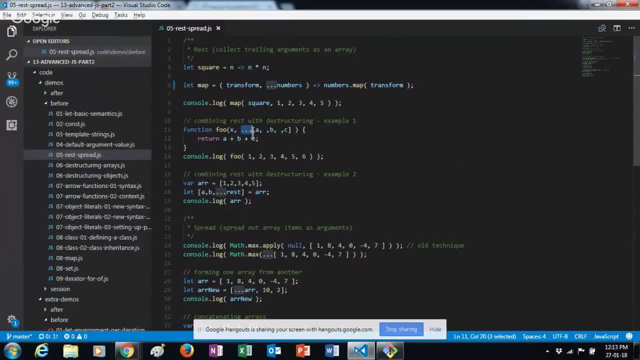 it's getting called, and then here we are using the rest operator. okay, so all the rest of the things are going to get collected into an array. so now you're going to have an array which is going to have two, three, four, five, six, five items. then what you're doing here is you're destructuring them. we had seen this. 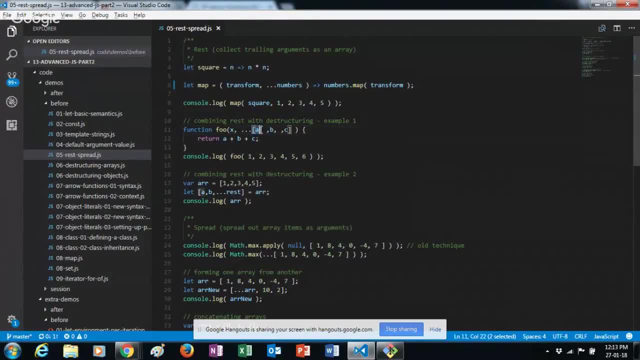 last time. so you're going to create local variables a, B and C. a is going to have the first one, then you put comma, comma, so I'll skip one. item B is going to have the third in the array. so the array is two, three, four, five, six, the. 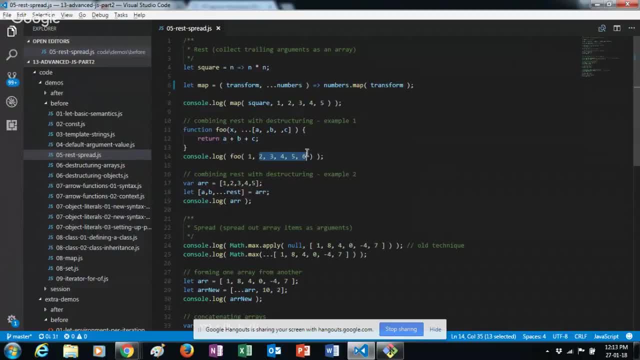 rest of the arguments. so two, then three will be skip four, five will similarly be skip B, comma comma C. so five will be skipped and six will get the value. two will get the value four and C gets the value six. so you are selectively. have extracted three of the arguments from the trailing arguments. okay, so you have combined. 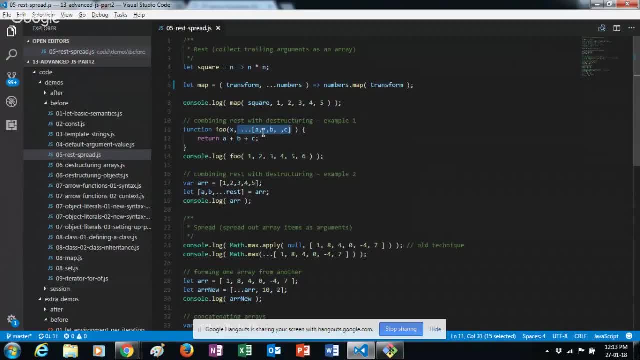 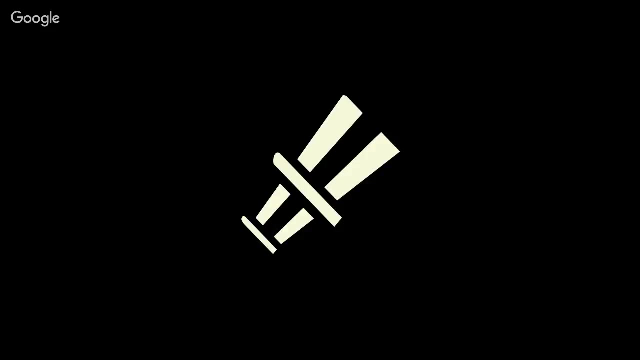 destructuring with the rest. so return a plus B plus C will be 2 plus 4 plus 6, so 6 plus 6, 12. all right, so this is going to well and go. all right, so 12. so this is really, really simple. if you had to, why create variables when you? 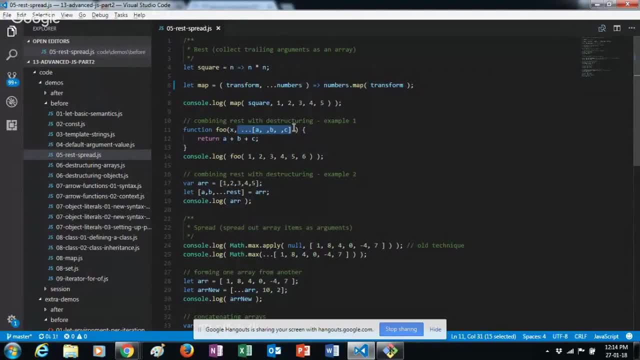 don't require them, why create maybe a, D, a knee and F and you're never going to use it? so I just wanted the first, third and fifth from the training arguments or second, fourth and sixth from the actual arguments. total number of arguments passed. all right, so we are extracted and we used it. you can even combine them. 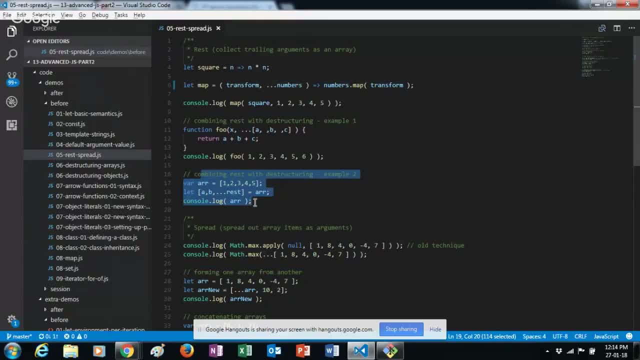 when you're. you can combine destructuring and rest when you are getting the return value, for example. you can combine the rest when you are getting the return value, for example. when you are getting the return value, for example, or something like this, and array one, two, three, four, five, or something like this, and array one, two, three, four, five. 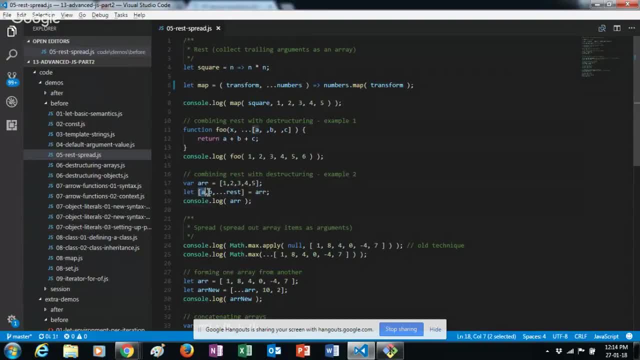 now you're forming variables like this, so you're destructuring a comma B- so this you know very well from last time. so a, b will get the value 1 comma 2. then you put dot, dot, dot- that is the rest operator- and created a array itself. 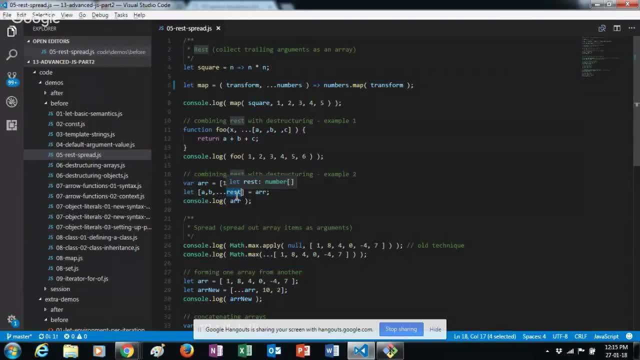 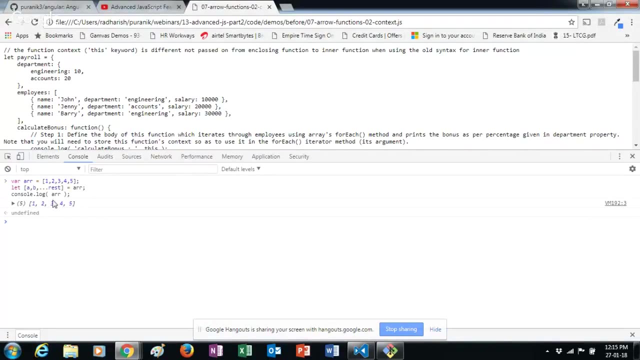 called rest. you could call this anything. you called it rest, so this is going to have that trailing numbers, so it'll be an array with 3, 4, 5. if you lock this, this will be an array with 3, 4, 5. okay, so that's. uh, we have logged arr, so it shouldn't be arr actually, so it should be. 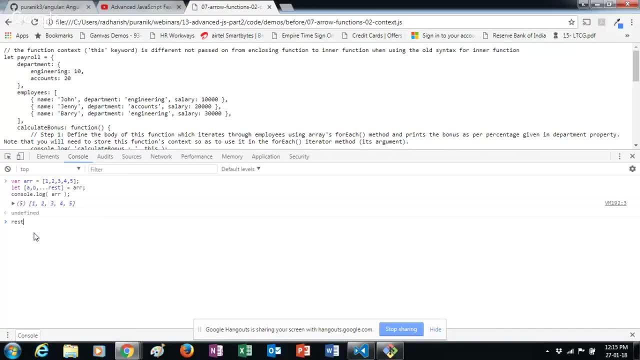 the rest. okay, let's log rest. okay, you can see, rest is three, four, five. so this way we have created an array with the trailing destructured. we are using destructuring so it's going to collect the trailing things into an array. you use rest so it's collecting as an array. dot dot dot, so it's collecting into an 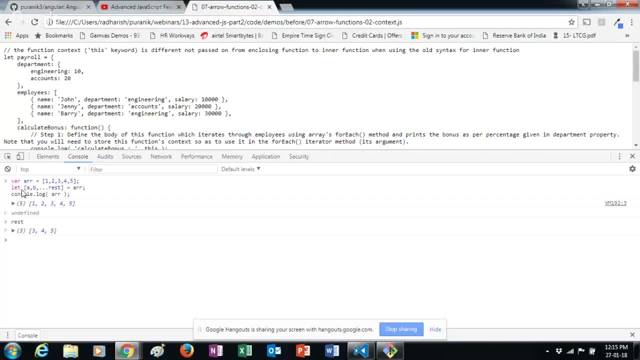 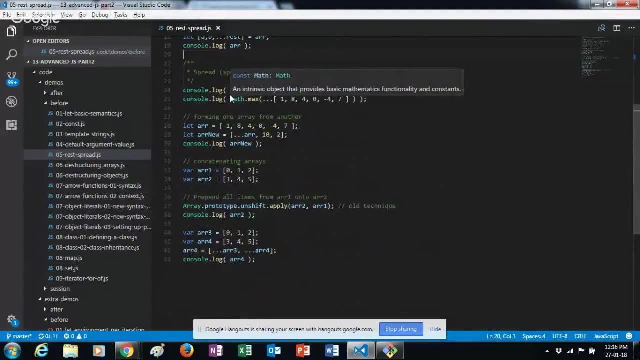 array called rest. and then we have used destructuring here to create three variables- ab and rest- and get the values from arr into them. this way you can combine destructuring with rest and it can be really powerful. it simplifies a lot of things. again, spread is one more operator. okay, it's overloaded. the dot dot dot operator is overloaded. 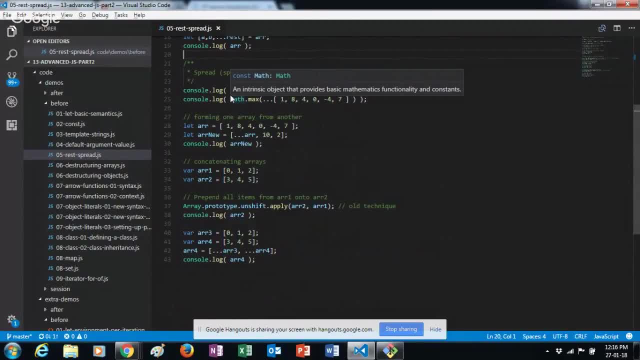 so you shouldn't get confused. the rest and spread are related in that you can consider them as- uh, what do you say? the inverse of each other? uh, and they have the same: they are overloaded. so the uh, they both are represented using dot dot dot. so don't get confused. you should know the difference between rest and spread. it's. 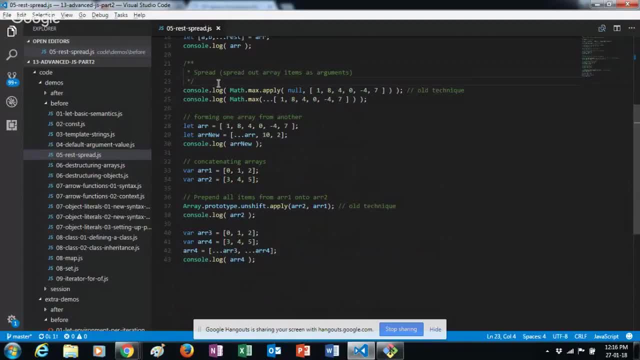 very easy. this is where people get confused. you should be: uh, both are represented using the same operator: dot dot dot, the ellipsis operator. okay, but there are two different things here, like: so they're inverses of each other. okay, so they're related, but they're not the same. it's easy to get. 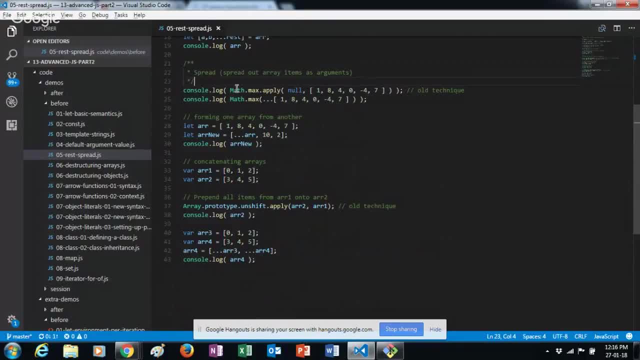 confused. so console dot log, for example. this is how we would uh. again, i'm not going to details of this. this is basically going to find out the maximum in the array given array. so array one: eight, four zero zero minus four, seven, so the maximum is eight. so this is going to be the 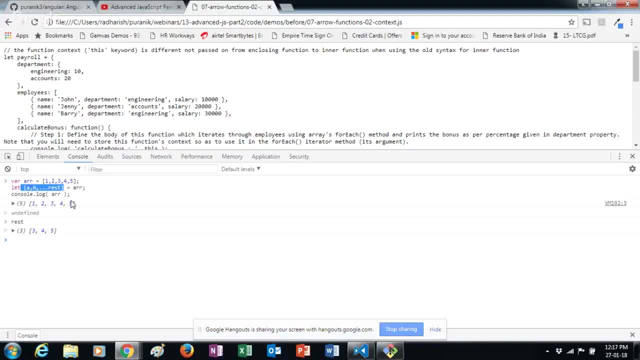 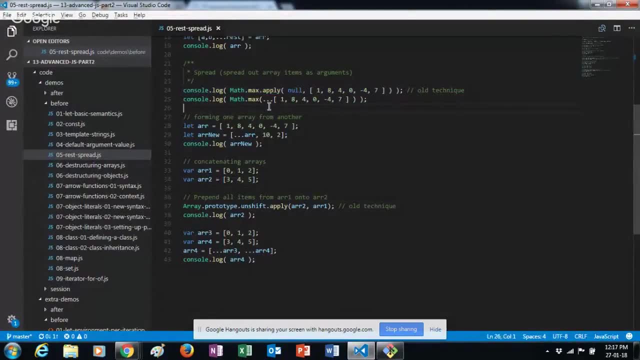 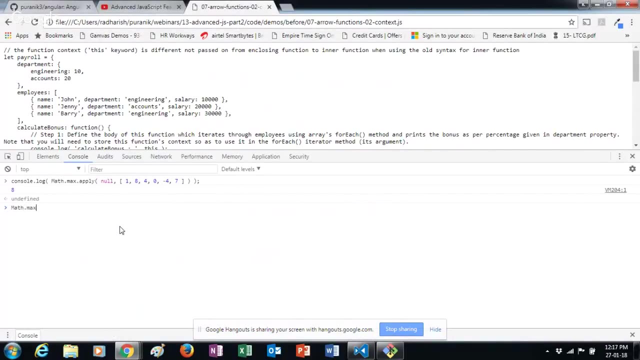 maximum. anybody would get put off by this kind of syntax it gives. but now with the spread operator, okay. so what the spread operator does, basically how math dot max works, let's see, because that'll be required to understand the spread operator itself. so math dot max app accepts any number of arguments. okay. 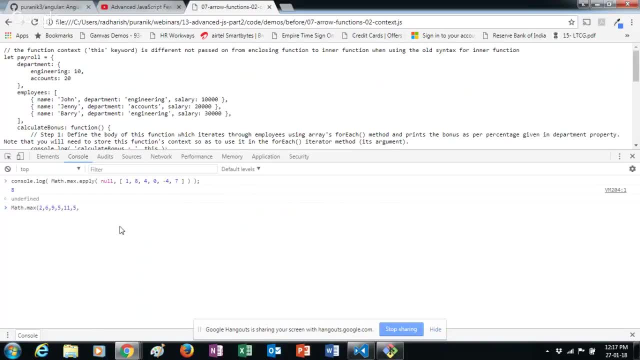 and you can see it's not an array of arguments. it's any number of comma separator arguments, basically, and it gives you the maximum 11 in this case. so what we want is comma separated arguments here. right, we don't want an array. if you give like this, it doesn't make sense. okay, it doesn't make sense. probably it will return. 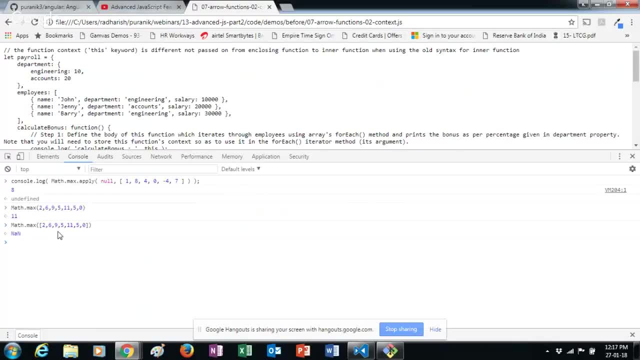 the entire array. that's all it will do. it says nam. in fact, it says i give up. all right, because this is not a number. it was expecting numbers. you passed an array. so the important point is, if you're going to use mat dot max, it is going to accept comma separated values of numbers. 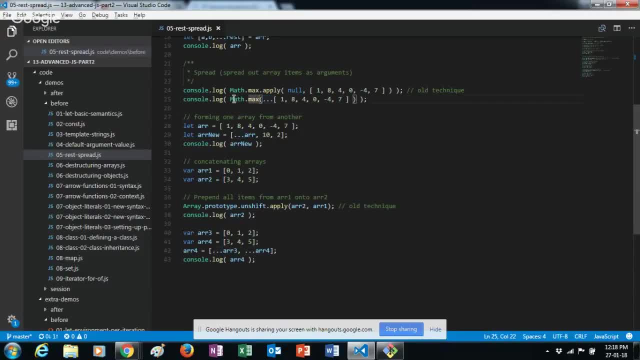 so arguments as numbers, basically any number of arguments. so mat dot, max. let's say you have an array earlier, if you, you had to find out the maximum array array. this is how you did it. you're not going to details of that, but it's definitely complex. that's the point. now, all we need to do 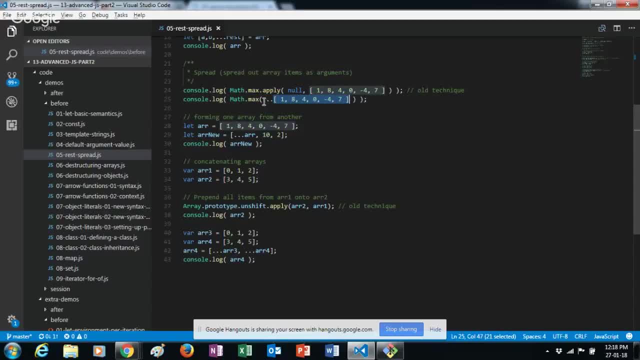 to convert an array to a comma separated list of values is precede prefix: the array with dot, dot, dot. this is called the spread operator. okay, important point is it is not the rest operator, it is the inverse. you can say it is not the rest operator, it is the inverse. you can say it is the 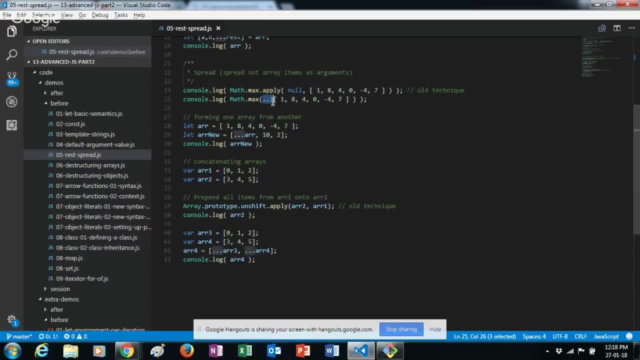 rest operator. rest operator is used to collect arguments into an array. this is used to break down an array into arguments. you can say or comma separated values. so this array is now broken down into it's equivalent to saying: when you apply dot, dot, dot, it is equivalent to saying this: 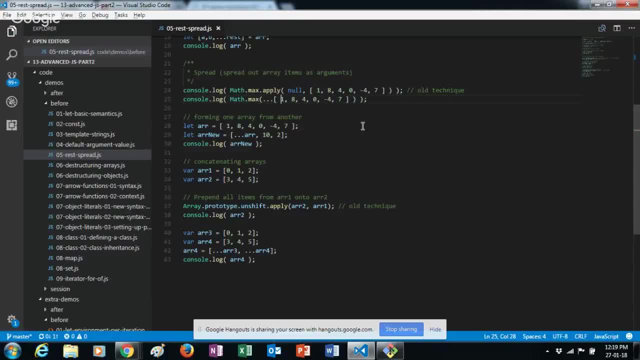 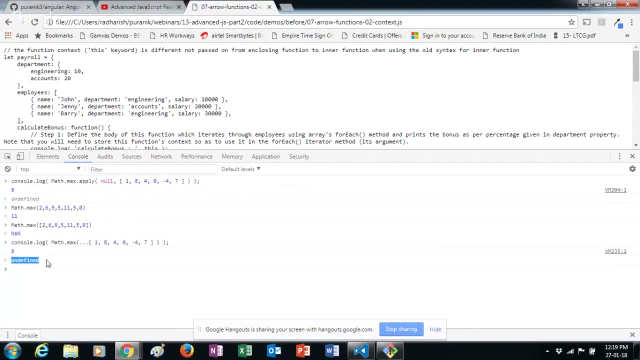 okay, so exactly, it does exactly this. so dot, dot, dot, the array. so now you have an array whose i to have become arguments to mat dot max. this will also work, but this is much more understandable. okay, this is the consolelogs. return value: so eight. this is much more understandable when. 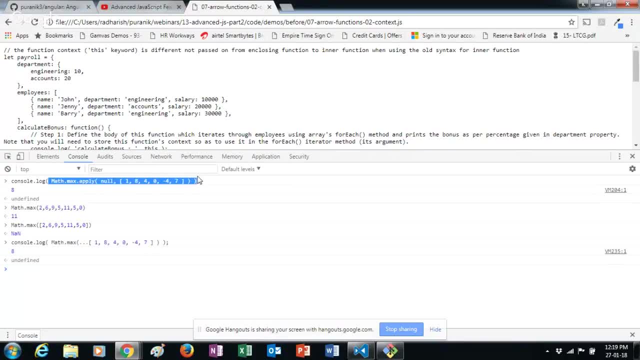 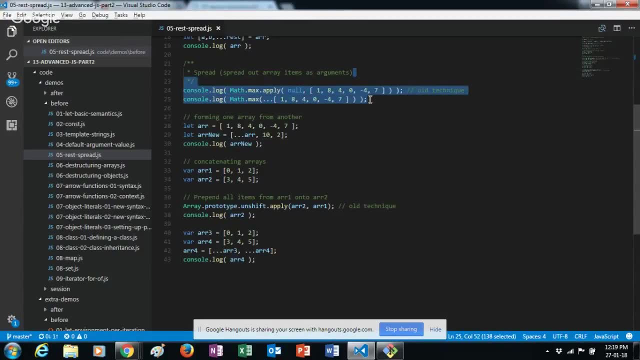 compared to saying mat dot, max dot. apply null comma array. all right, so the essential idea of rest and spread is to eliminate such cryptic usages in javascript. okay, so that's one thing. so we have seen the spread operator is used to spread out and array items into arguments. 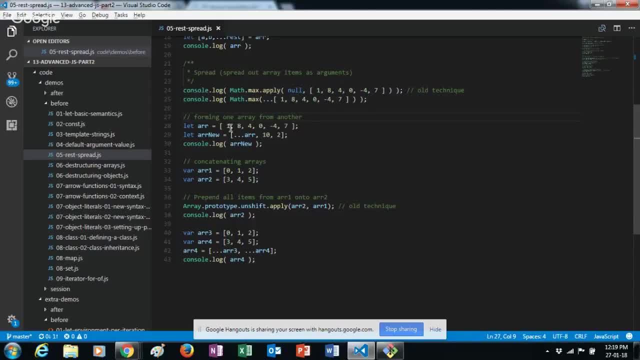 if you want to form one array from another, then also you can use spread. so what you will do? so basically, you can concatenate arrays and stuff like that. for example, you have an array here, one, eight, four, zero, whatever- and you spread it out, so you're creating a new array. 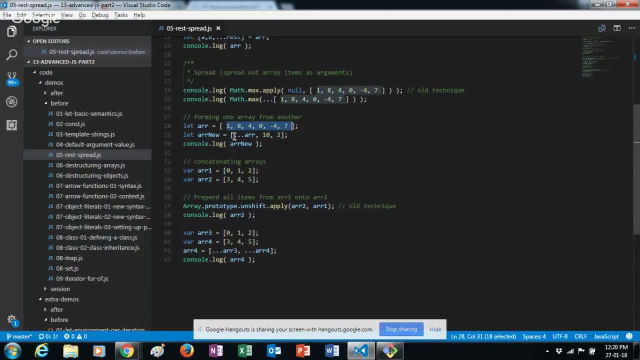 that time what you can do is the items in the existing array, you spread them out, you make them comma separated and add two more. see, it's very simple when compared to arrayconcat. you just said dot, dot, dot, whatever items are there, just spread them out and then 10 comma 2, that's it. 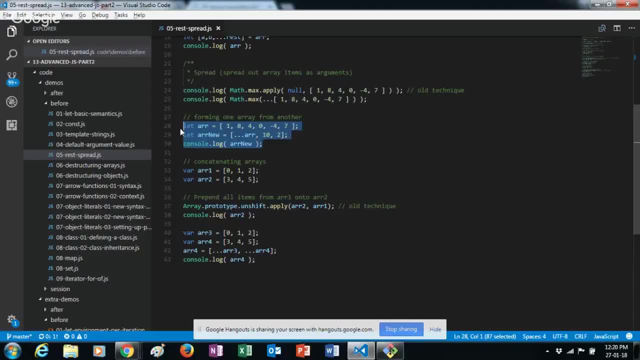 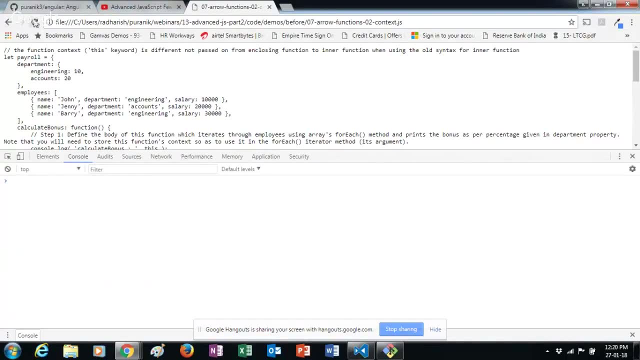 so this will be a new array with all those items plus 10 and 2 at the end. all right, so i have to refresh. okay, so you can see all the new array. new is nothing, but all the old items of arr, items of error, plus 10 and 2. errors items and then 2 after that. 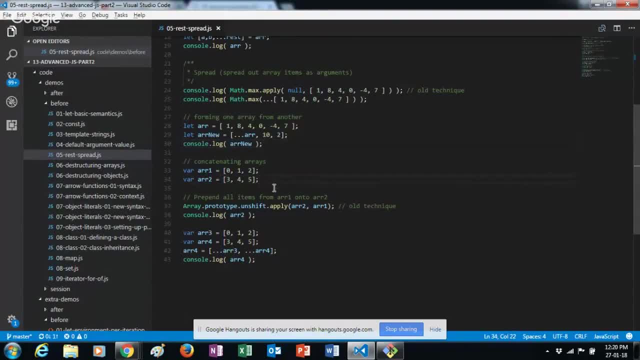 so very, very straightforward. okay, so it can be used for concatenating arrays. earlier you would have done some crazy stuff like this: arr 1, 2, 2 arrays, array dot, prototype dot, unshift dot apply. okay, so we are not going to the details. even looking at this is very difficult. 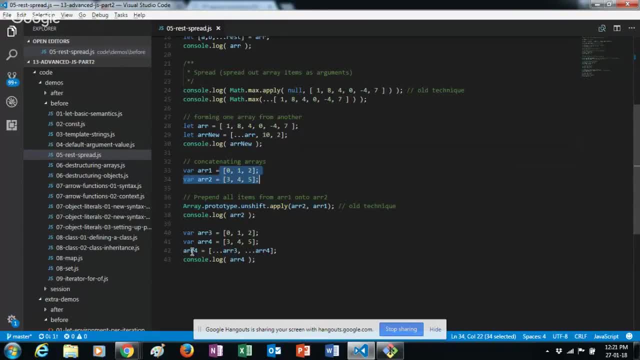 all you wanted to do is concatenate these two arrays. now you just use the spread operator, so two arrays. you create a new array where you spread out the first array, three items. you spread out the second second array. that's it right. so dot dot dot. here are three dot dot rr4. that's the items of the new array. that's it. 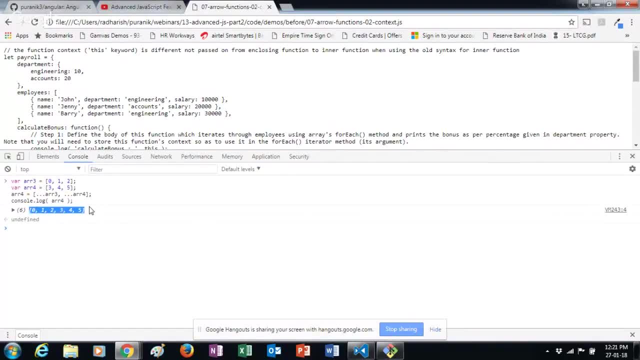 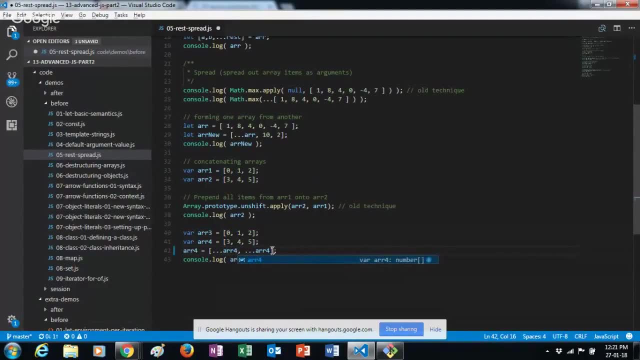 there you have a new array: zero one, two, three, four, five. so you can, you could have. you could have put array four items in the beginning also if you wanted, all right. so instead of like this, also, you could do. so it's up to you what you want to do. 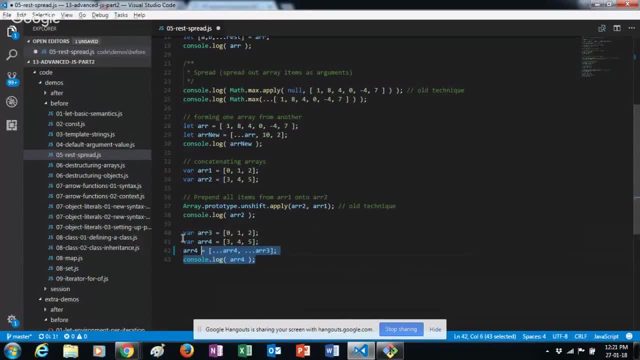 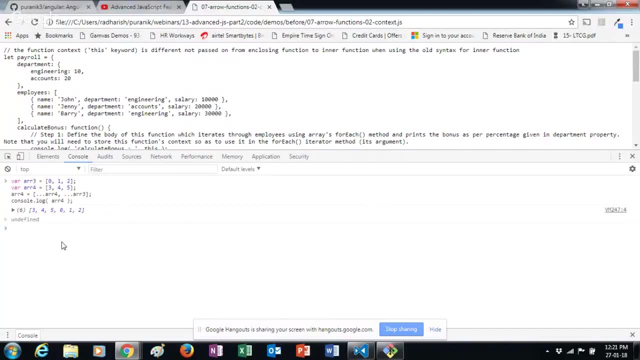 so you don't have to worry about shifting and shifting or push pop, nothing like that. this time you put array four items first and then array three items next. dot dot dot, arr4, dot dot, comma, dot dot, rr3 are the items of the new array, square brackets. 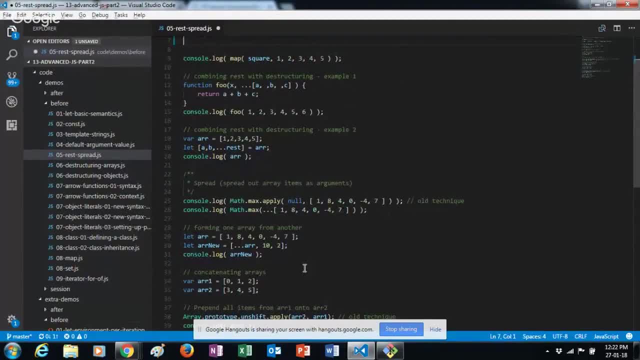 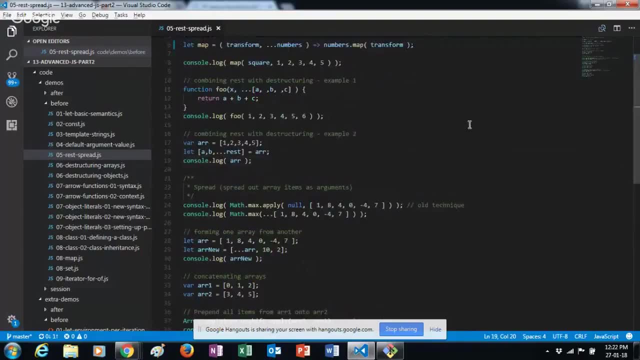 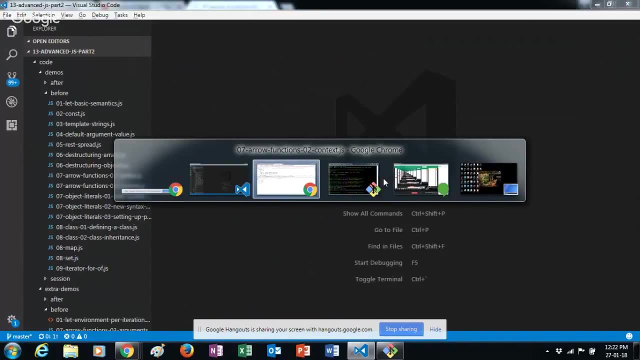 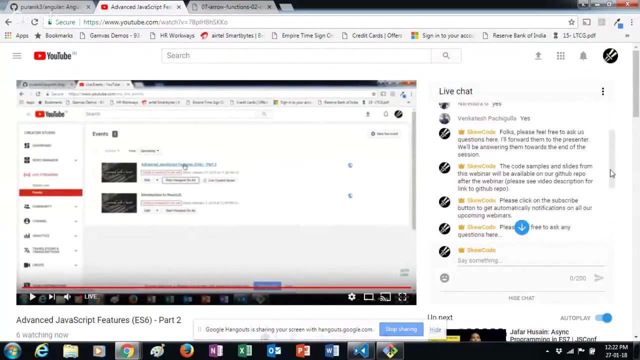 okay, leave it at this, all right. so that's about rest and spread operators. all right, since we have done few things, i might take a few questions. now. let me take a few questions. is there any questions? let me just check, all right, any questions? folks, i don't see any questions. okay, please feel free to ask any. 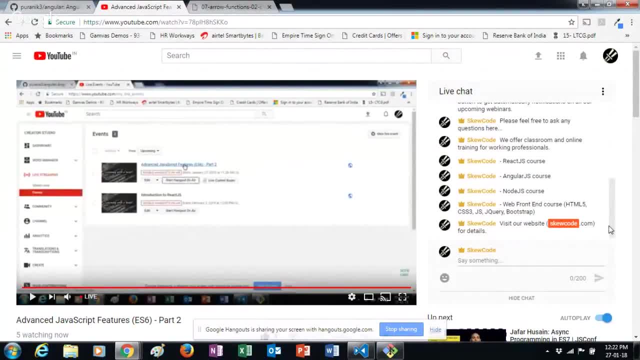 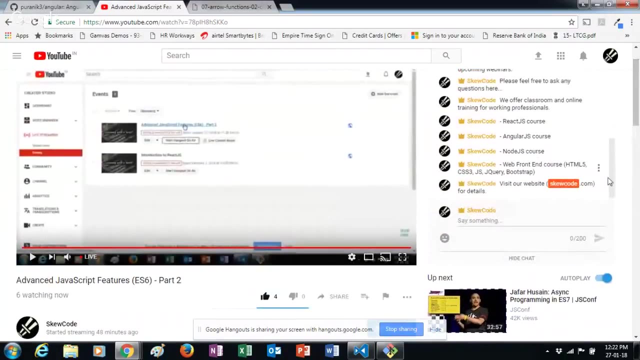 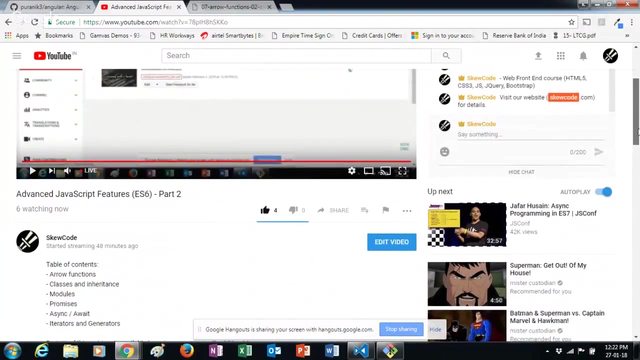 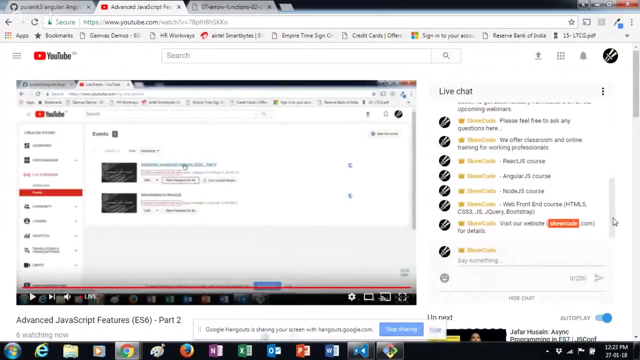 questions, but once again, let me just check whatever you have. any question, come to me, i will answer them for you, okay. okay, you have- as I said I might not take it immediately- any questions folks, alright, so I think, no questions, I'm just checking the live chat. no questions at. 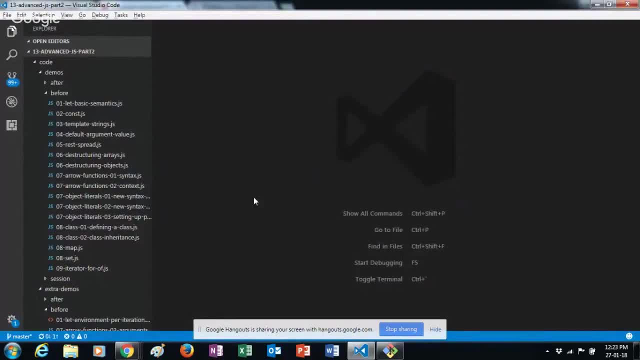 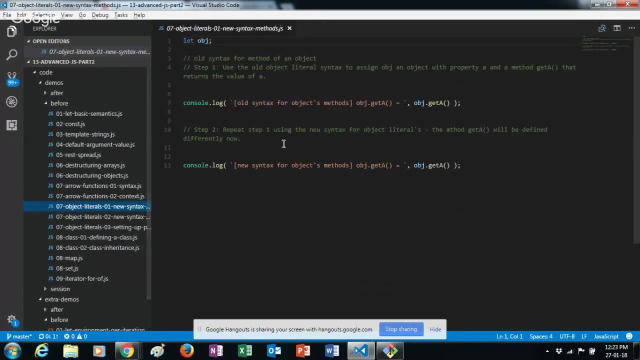 all right, so let's continue. so we have seen rest and spread. we have seen arrow functions. now it's a time to move on to object literals. so we are going to object-oriented JavaScript. all right, so that is a new syntax for object literals in JavaScript. so let's make you so if you have to. 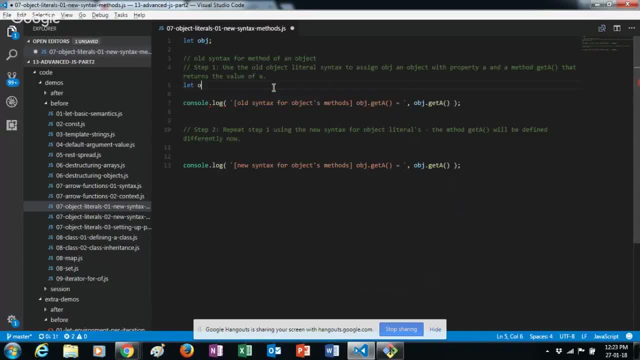 declare a variable. earlier I'm using let. do that. you would say probably VR, obj in old syntax. so let obj equals. you would have said something like this: and let's say there's a property, a, whose values in the same one, and then you need to define a method. let's say, get a, which will get the value of a. so you would say: 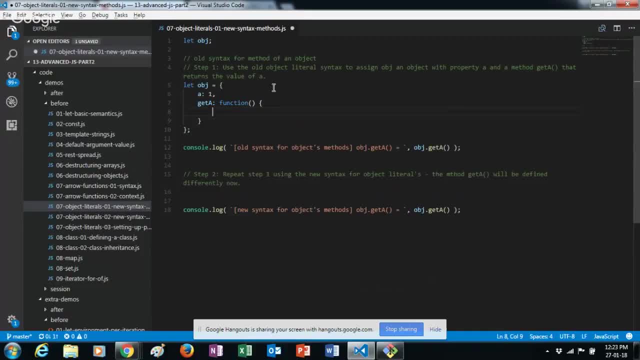 something like this: get a is a function but basically returns the value of the a property, so this would refer the method get it. So, within the method, this would refer to the object of which it's a part. So obj, So objh. 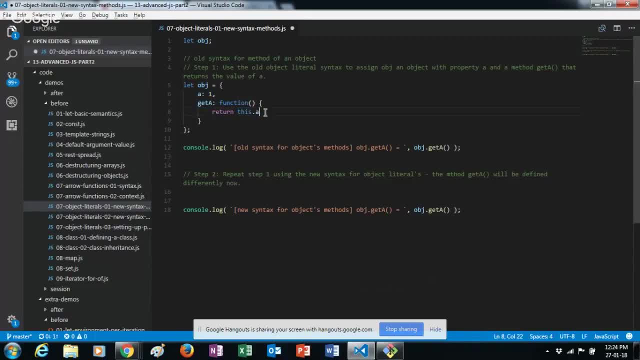 Get a is a part of obj, So this would refer to within that method, obj only. So you do something like this. All right, This is one. This is the old syntax. Of course it would work. So you get something like this: 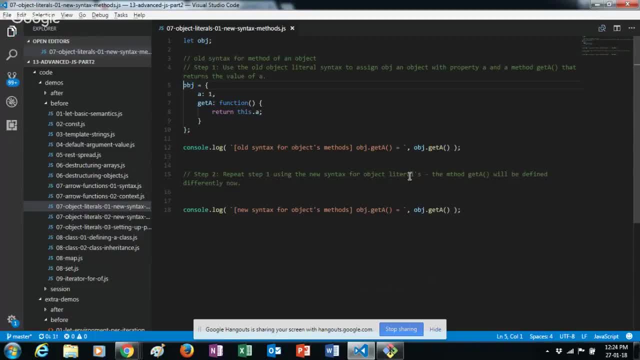 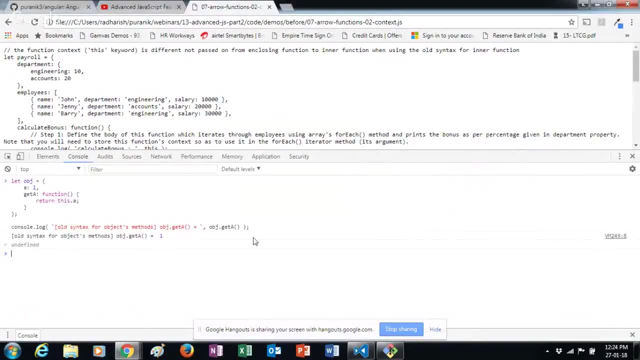 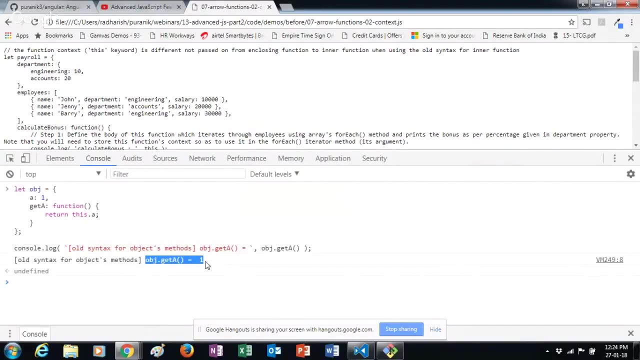 There's already a let obj here, So I may not have done that. All right, So you can see that it works. All right, Objget a is equal to one, So it has got it In the new syntax. it's simplified a bit. 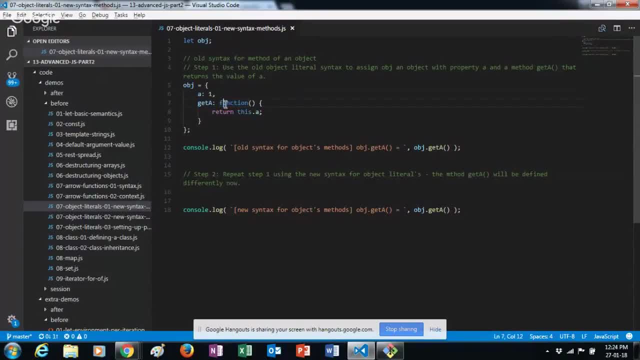 So if you have a method, you need not say method, name, colon, function, the function expression. Instead you can simply say like this: Okay, So properties, it's like this Key colon value. But for methods you can just say like this: 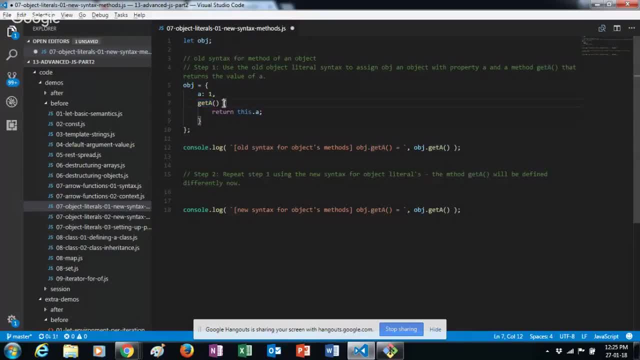 So the method, The method name, Arguments within brackets- and the function body, Method, body. All right, So you can do this. This is a simplified syntax, So this will also work. The slide thing- the old syntax, still continues. 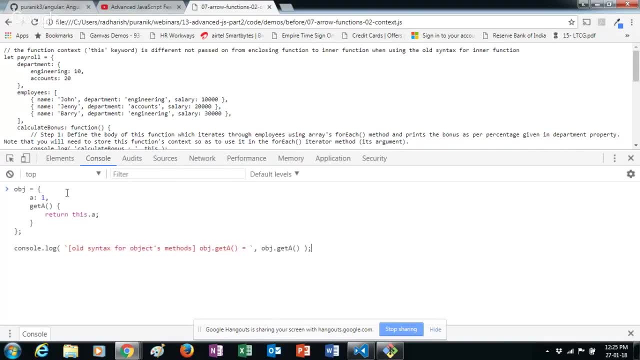 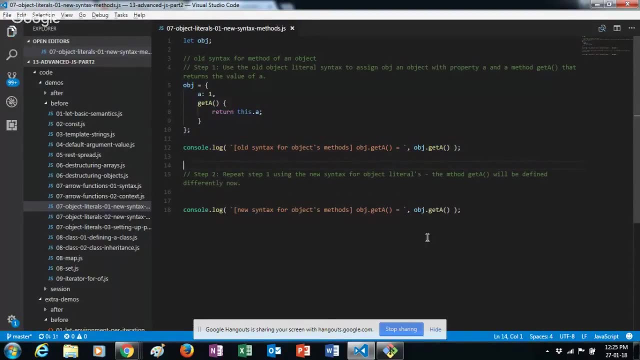 But you can also use this new syntax, which is simpler, So you can see here it still works: Get a is one, It returns one, So that's one thing, All right, So that's exactly what I just did. 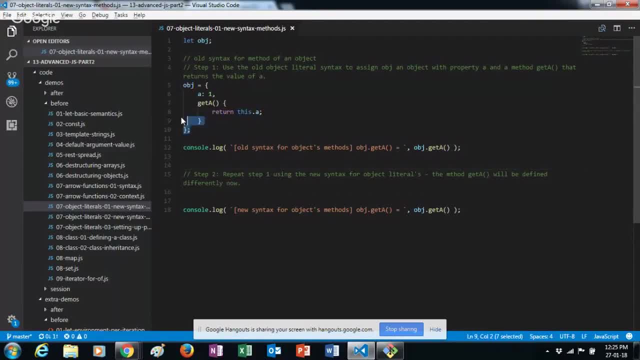 Okay, This is the new syntax, Whereas the old syntax would have just told: get a colon function. I comment this out since okay, or I can even let it be Okay. So that's the difference between the two syntaxes. 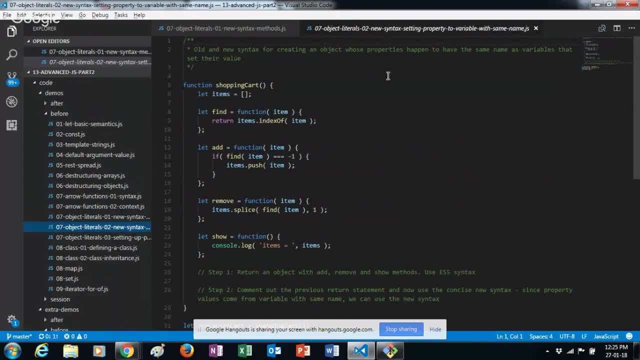 Object literals continuing. So when you're creating an object, So when you're creating an object, So when you're creating an object whose properties have the same name as variables that set their value, then that's a new syntax. What I mean is, let's say, this is a standard module pattern. 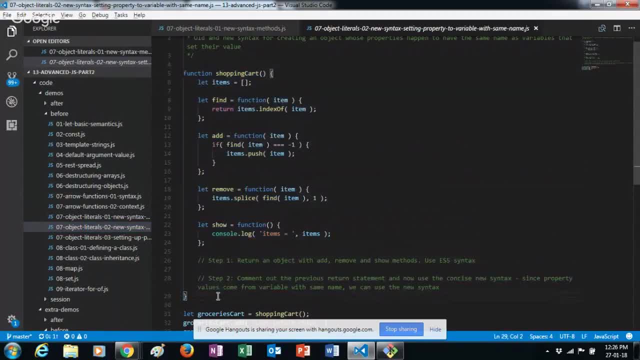 Have the module pattern. well and good, But if you're not aware, you'll have to refer somewhere. But that's not the main point of this: Be able to follow to a great extent. So the thing is, this is a function which essentially represents a shopping cart. 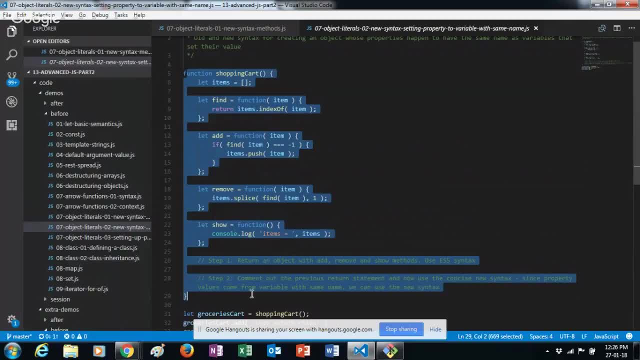 Everything related Everything related to a shopping cart, like adding items to a shopping cart, displaying the items, removing items, all that functionality is encapsulated, sort of, by this function called shopping cart. It's basically the module pattern. These are the private variables. 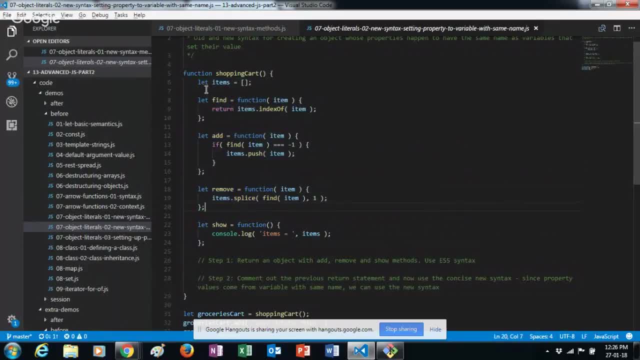 And then you, selectively, you want to reveal- Okay, This is called the revealing module pattern, So you want to reveal only certain ones, certain methods. So you basically return an object like this: This is a very, very common pattern in JavaScript, so I'm not getting into it. 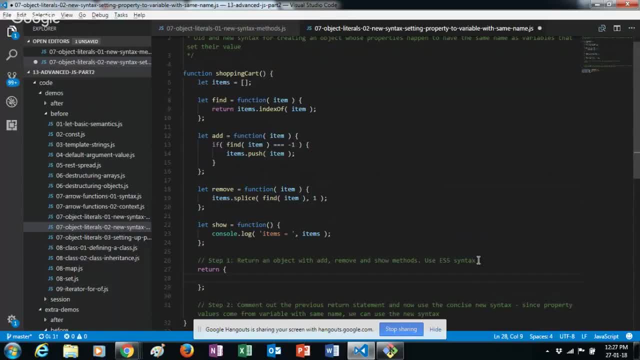 So if you are, I guess, if you are quite experienced, a bit experienced also, you should- you would definitely have come across this. If not, please check for module pattern. You will get some material on it. The point is, we are returning an object here. 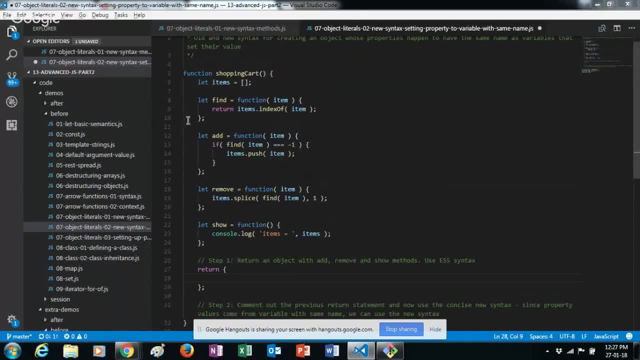 Okay, Which is going to look like this. Now to the outside world. I don't want to expose find function, So I want to reveal it To the outside world. I want to share this, So share the add function. 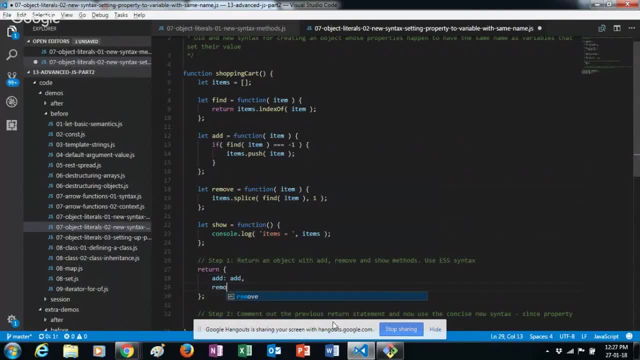 So I'll reveal it this way: Okay, Remove, I want to share with the outside world. Show. I want to share with the outside world. So these three methods are the public interface. Okay, The one object that's written basically has these properties. 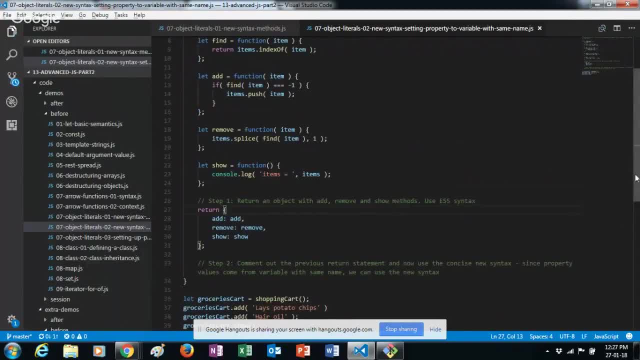 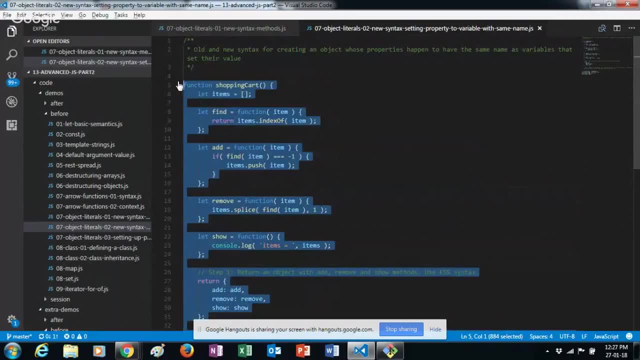 Now, if you see here, of course this will work and the shopping cart will work fine. If you see this code, when you execute it, we'll be able to create a shopping cart, add items to it, and so on. 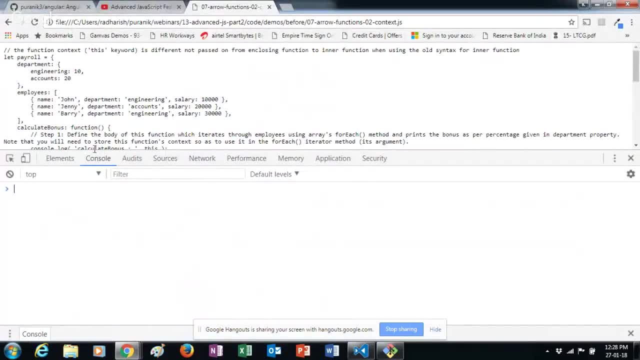 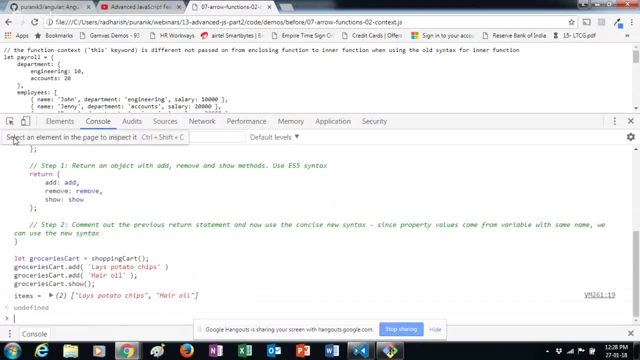 So this is going to show it. Okay, Works fine. Brosseries cart: we have added these things And then we are saying show. So the two items are being shown. It's working fine. The module pattern itself is not the point of this demo. 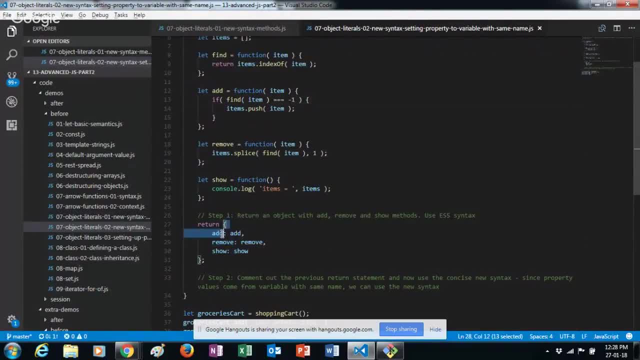 So don't worry if you don't understand it at all. The point is we have created an object here, Okay, Okay, which whose properties have the same name as the variable through which it is being set. so add property in javascript. all properties are strings, okay, so don't get confused that the left 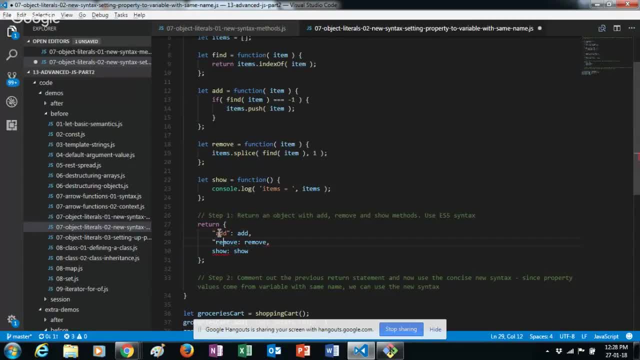 hand side and right hand side are same. left is actually a string, basically double or single quote, or even back to quote it now in mia6. it's actually this, okay, so you don't have to worry. okay, so basically you have your property names same as the variable through which it is set. 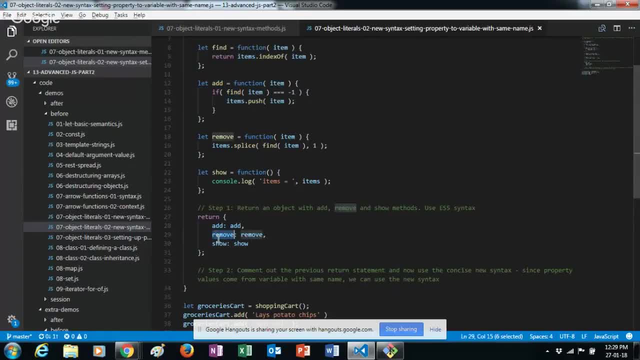 so add is nothing but this add function, remove is nothing but this remove function, and show is nothing but a show. the variable name and the property name happen to share the same identifier, so in such a case there is a simplified- it's a common pattern, okay, this thing comes across so many times. 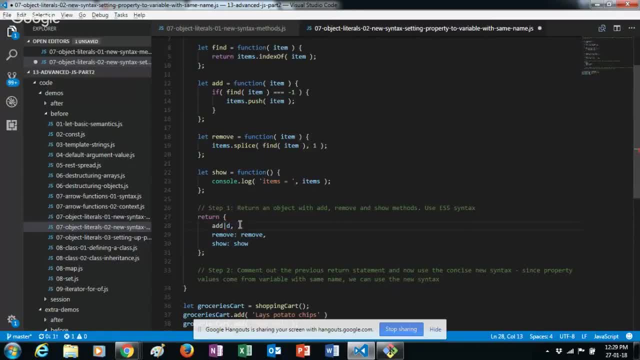 okay. so in such a case there is a simplified. you don't have to set it to that variable name, so you just give the one thing. don't have to say add colon, add okay, just say add comma. so at first glance this might seem really confusing. what's? 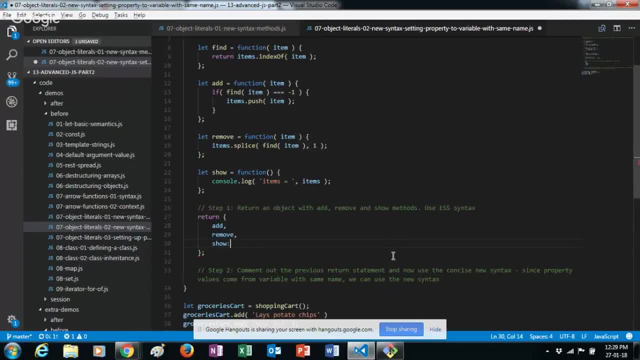 happening here. you're creating sort of an object and then you're saying: property, come up, property, come up, property with actually property, add colon, add, remove colon, remove, show, colon, show. okay, so that's the thing, right. so this is the old syntax. okay, all right, and this is the new syntax. 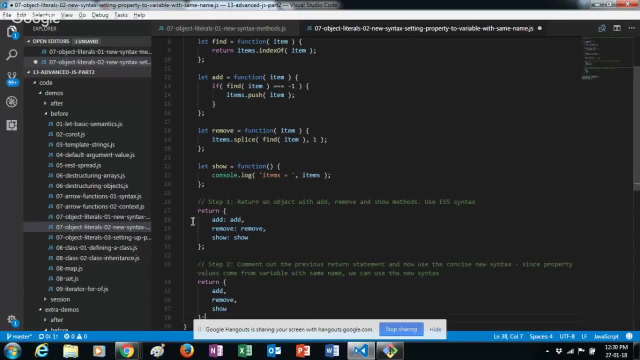 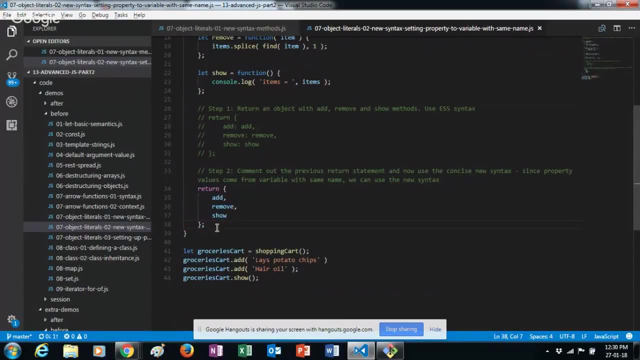 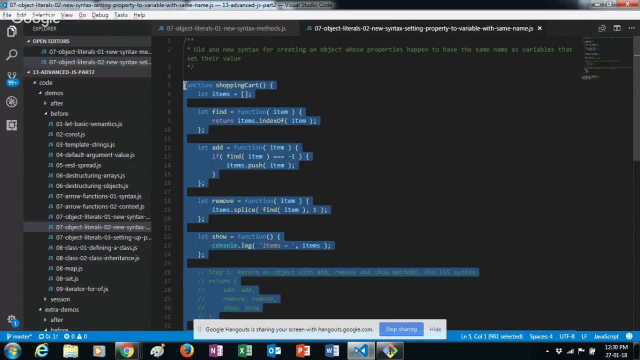 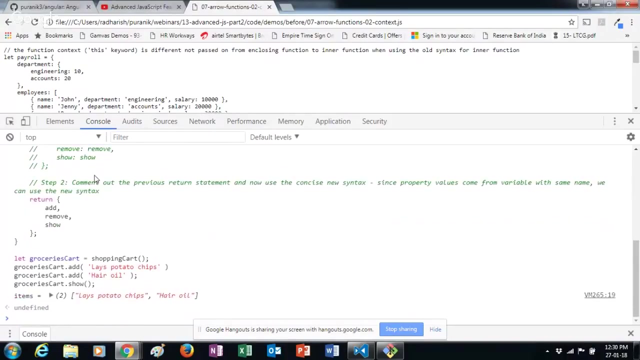 i'll just follow the steps. so this is actually the old syntax. all right, this is the new syntax. so that's about: uh, one more uh change to or one more new feature to object literal syntax. it will also work. fine, we can verify that. we can verify that. 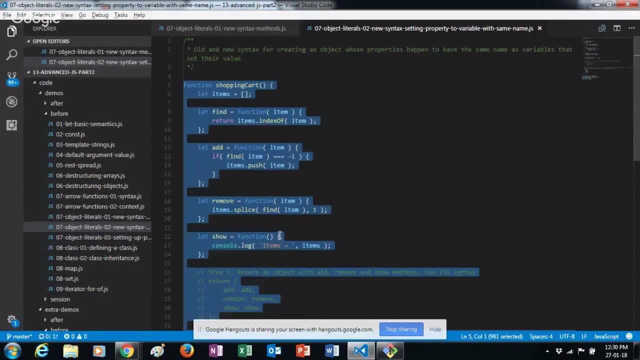 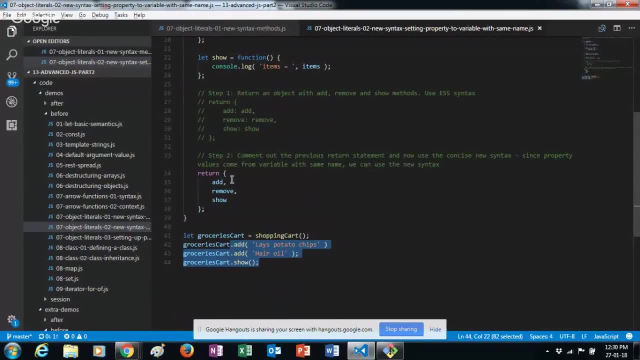 you can also caught in here. you can see there is no toolbar and the контакts so you can see that we returned to like. it is returned. see howgreen. so you can see here items. it's returning the state, so everything is working fine. we are able to use the object that is Alex's return task and show and so on. this is what is my habit: fading test. 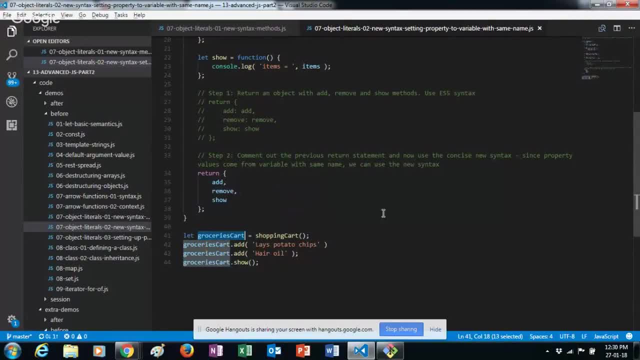 we can add show on on that object. we can use: Add shows up. okay, another one. and this means between: we run a call if this script gets deleted and we are able to set a check here to if the table will not enter. so in that case we can see the address, we can set a check. 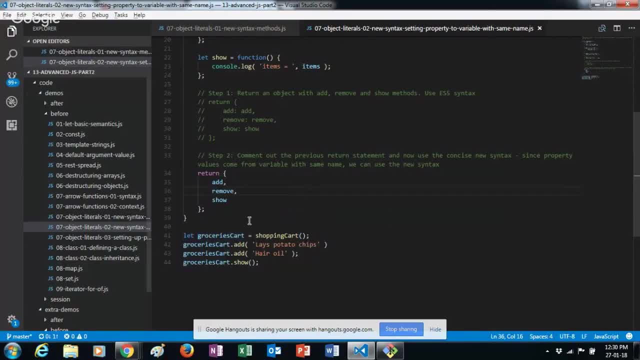 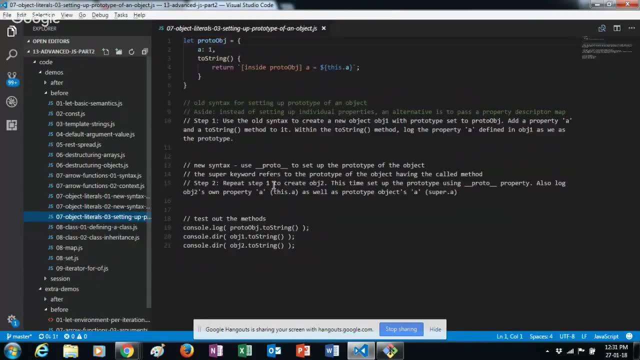 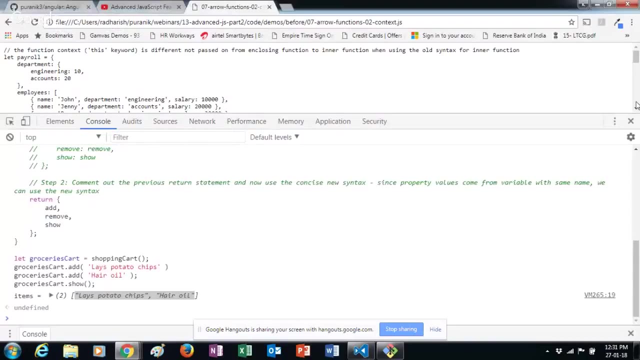 So that's one more change to the object: literal syntax. Finally, there are some changes to the way prototype can be set. If you're not aware of the prototype, no issues. So what the prototype is? every object has another. it's just like you have a father. 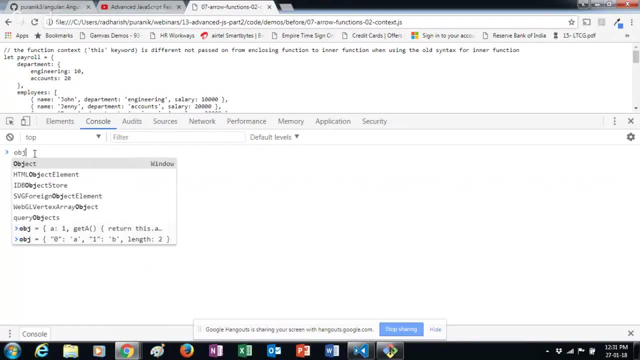 you have a mother. Every object is related to one more object, exactly one more object. that's called the prototype. For example, if you create an object like this with just one property, a set to one, it'll have a prototype. 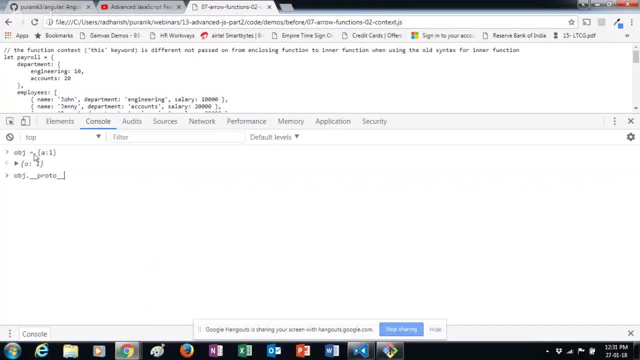 You shouldn't technically access it this way, but all browsers support the underscore, underscore, proto underscore underscore property. It's a double underscore before and a double underscore after, So every object is related. obj is related to this. one more object called this prototype. 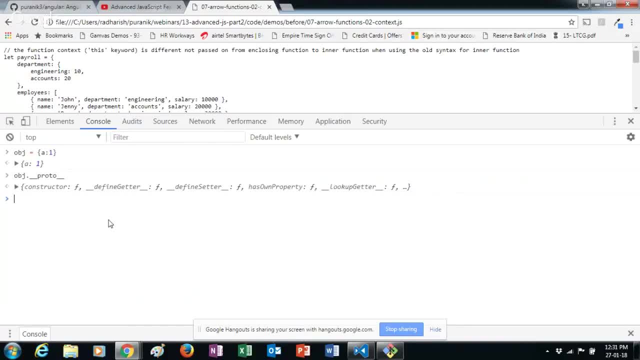 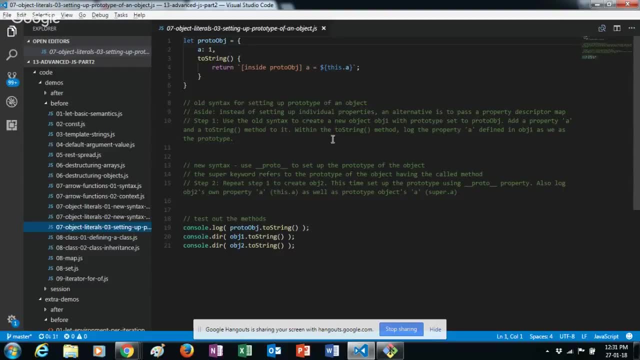 object. Okay, Earlier, if you had to set the prototype that used to be object dot, set prototype of all some circles used to be there, Okay. So let's see the old syntax. So let's say, with the old syntax we create a new object called obj one. 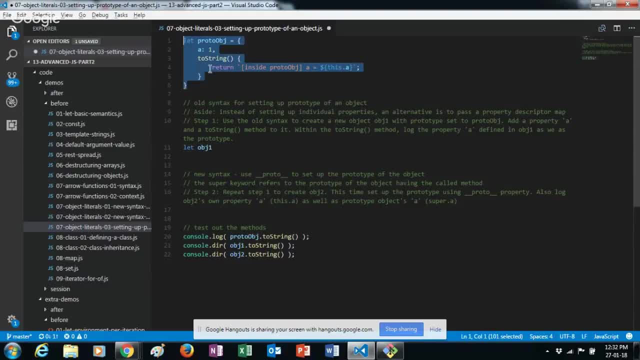 You can see there is already one object defined here, called proto obj. Okay, This is going to be the father or mother or whatever. This is of obj one. Okay, So obj one, let's create So equals. we had to say, okay, object dot create. 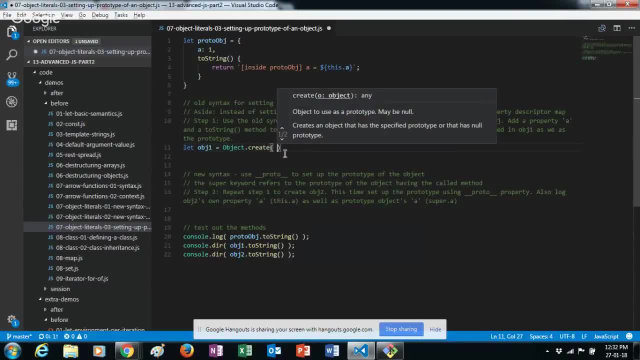 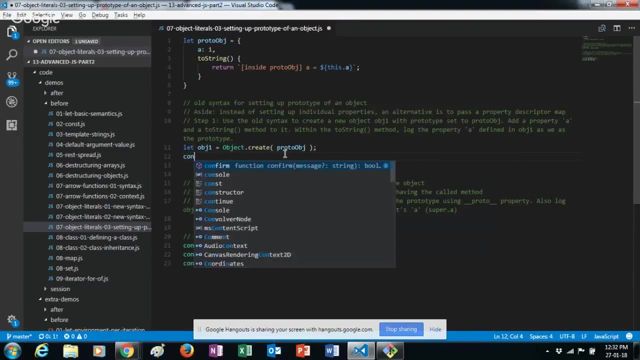 This is one way we could say okay. or then we could say: set prototype. or this is one way, Let's see, I'll show you. object dot create with the prototype being passed. So proto, obj. this way we could set, and then obj would have its prototype set to proto. 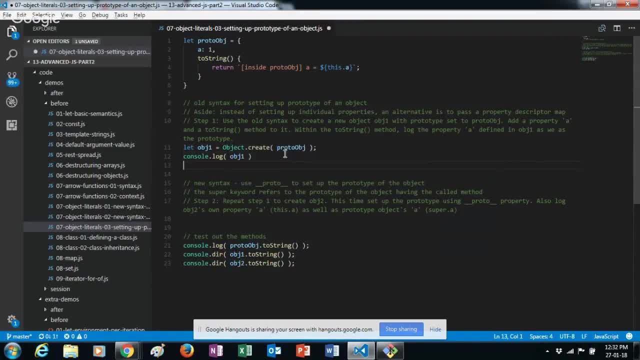 obj. Let's check that out. Okay, So that's a prototype object. And then there is an object which is a, whose prototype is being set to the prototype object. They're logging the object, All right. So you see that the new object is that it's empty, but it's prototype is set to our proto. 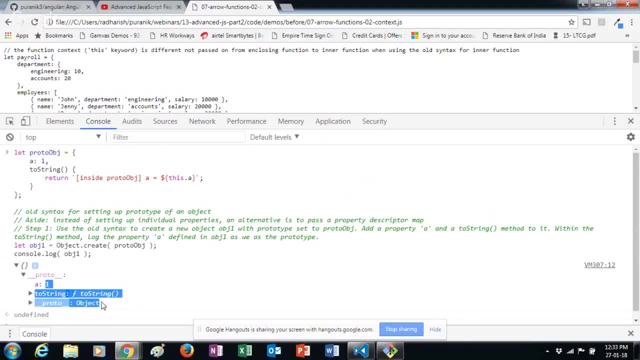 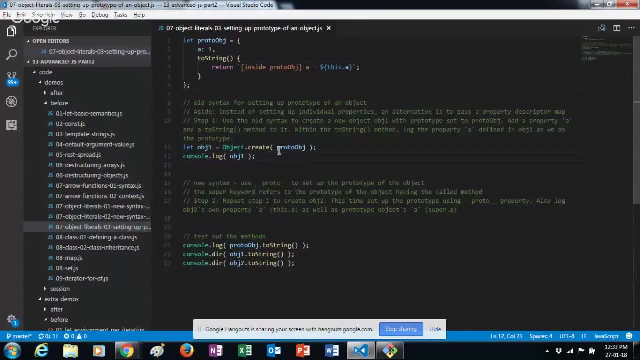 obj: A one, two string. Everything is there. A one, two string, And so on. Okay, Okay. So this is the one way, or what you could do is you would create the object. The other way was okay, I'll just come in this out. 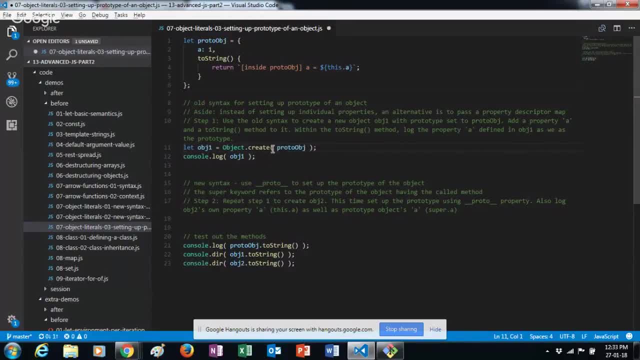 If you want to refer for future, what you would do is, when you're creating obj, you would say, okay, object, or you just create an object, empty object- Let's say a one- and set at least one property, And then you would say: go ahead and set object- dot set prototype of object. dot set prototype. 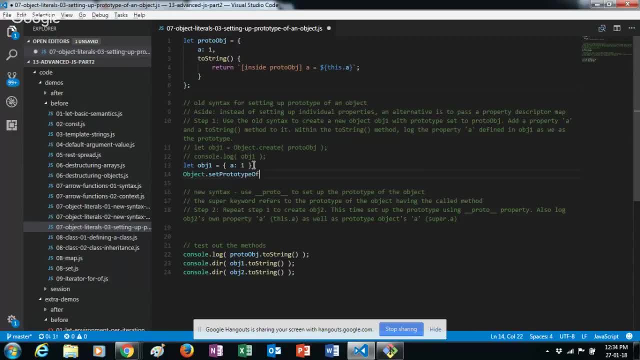 of obj one, two proto obj, proto obj. Okay. So this would set Okay. So this would set Okay. So this would set Okay. So you, you're born first, then your father and mother is decided in this case. 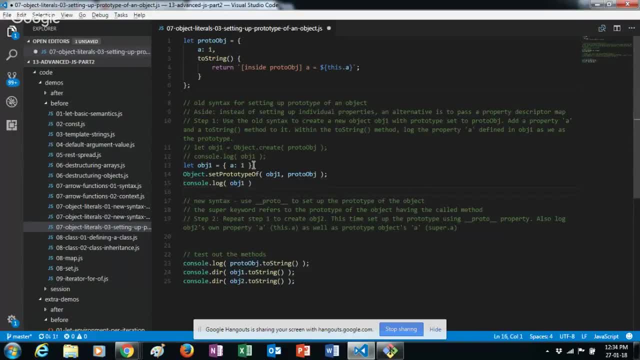 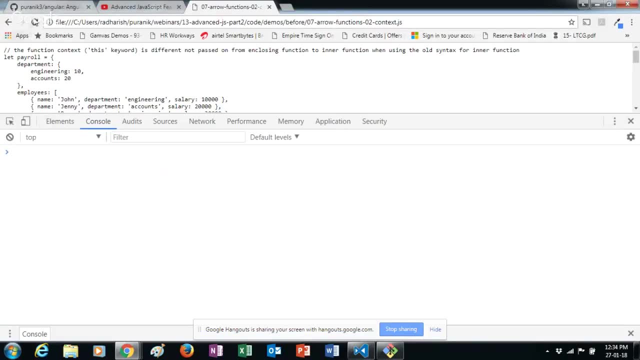 Okay, So sort of like that, or probably that it will have a father and mother, but it'll get adopted. That's the right way, Actually. Okay, So you'll see here, So we get one. Okay, I didn't paste obj one. 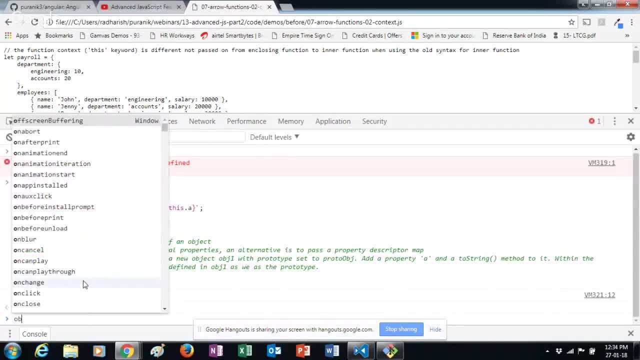 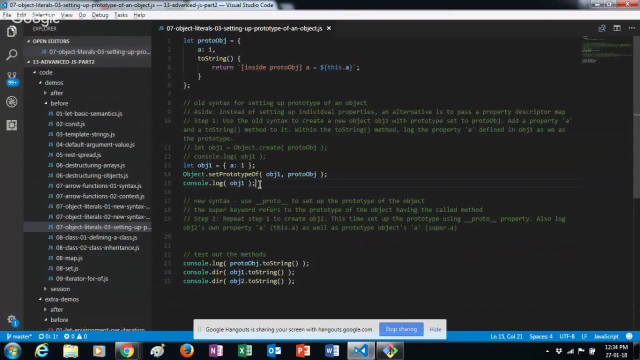 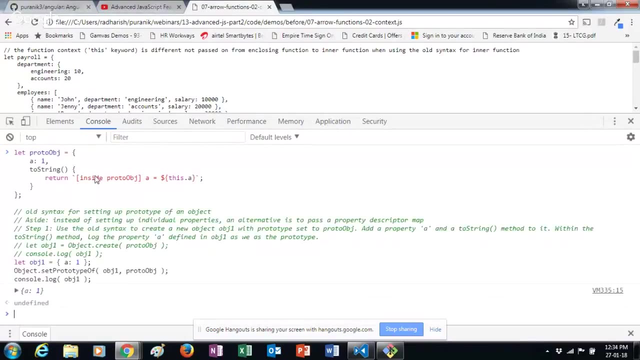 Let's kill the object. Okay, Okay, Okay, Okay, Okay, Okay, Okay. So this is the old code. Sorry, We can see here a one, And if you expand it, it's prototype is the proto obj. All right, 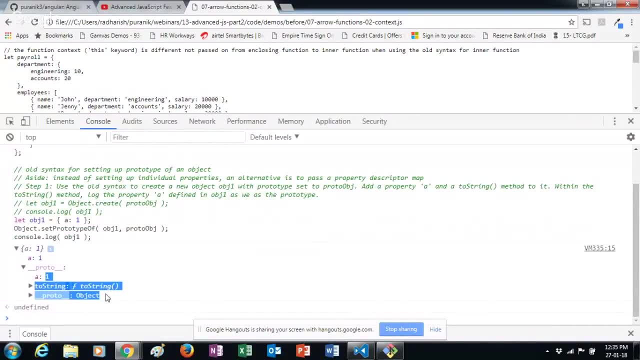 So we have set it up. We can actually, okay, We can set a to two, Okay, Okay. So we have set it up. We can actually, okay, We can set a to two. Okay, So we have set it up. 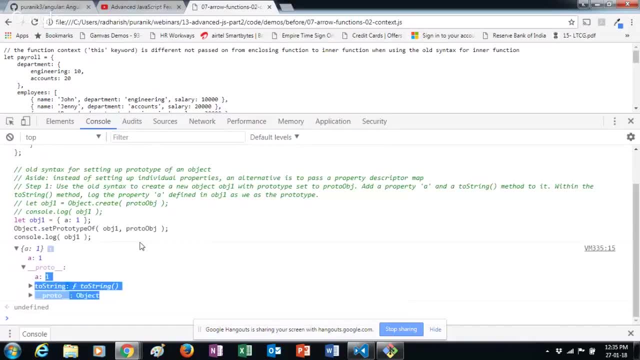 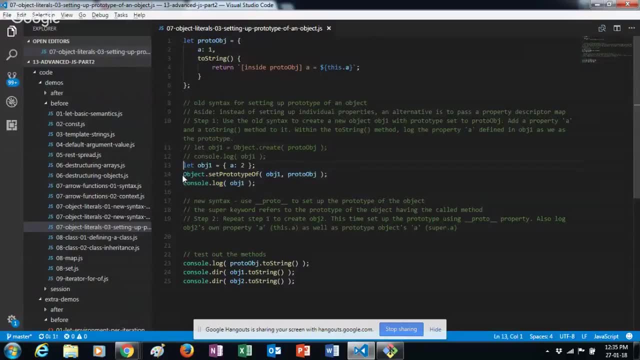 We can actually. okay, We can set a to two, Okay, Okay. So, instead of all of this circus- okay, Creating an object and then using set prototype of little lengthy, instead of all this, you can simply, while creating the object, set up like this: 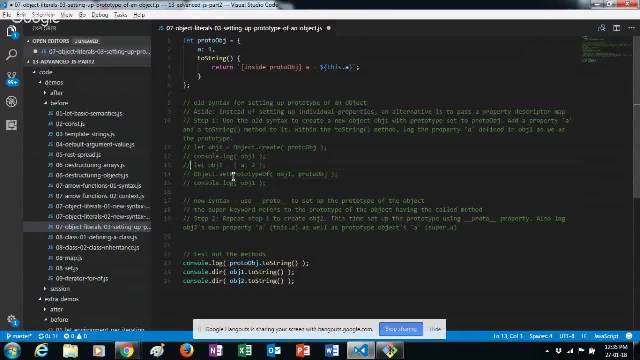 So we'll use a new syntax. Let this be there, All right, And actually let it be there Now, when you're creating the object. let's say let obj two equals Okay. So let's say a three and to set up a prototype, 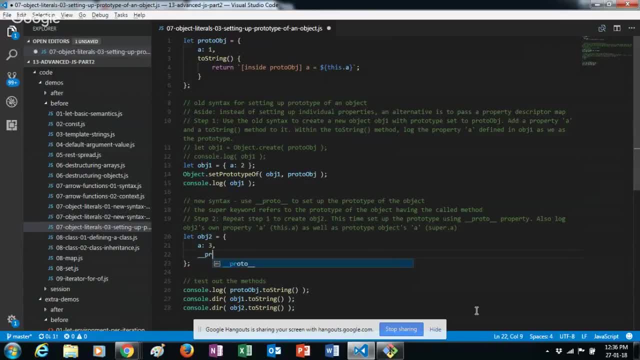 All you'll do is you say: underscore, underscore, proto, underscore, underscore- Earlier. you couldn't do this. The prototype could not be set using the product property And it's going to just go proto on this current scope property. It was not possible. 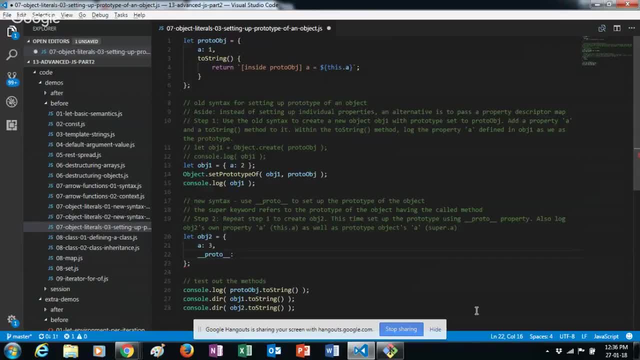 it was not possible, now it's allowed, so you can say: underscore, underscore, proto, underscore, underscore should be set to proto obj. that's it very straightforward, very clear. also, when you're creating the object, you'd say: the proto is set to proto obj. that's it very, very straightforward. 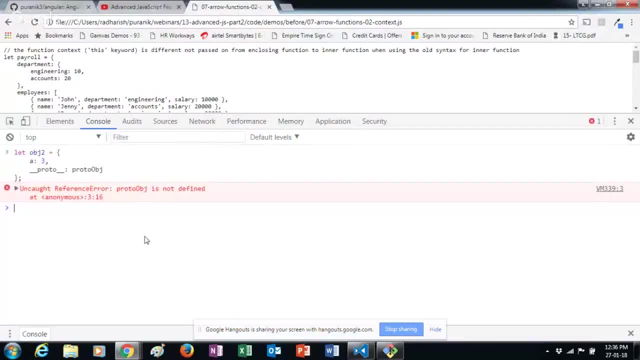 we have not defined, so let's copy this first. so proto obj is defined and obj2 is created and its prototype is set to proto obj. the obj2 has already been defined. it says: so let's make this three, all right? so obj3 is an object whose prototype. 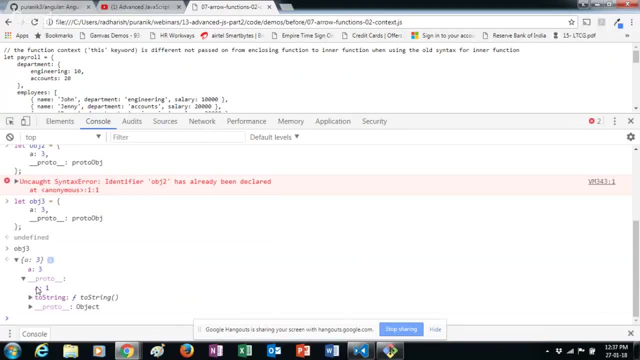 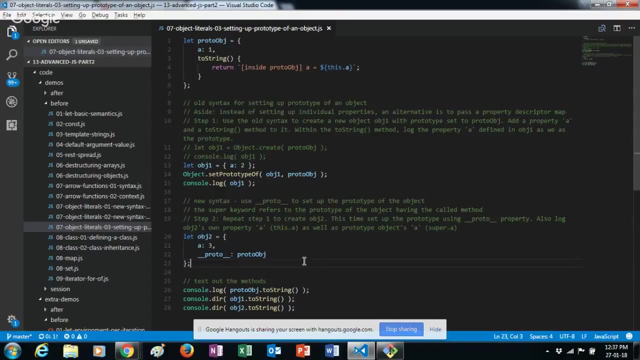 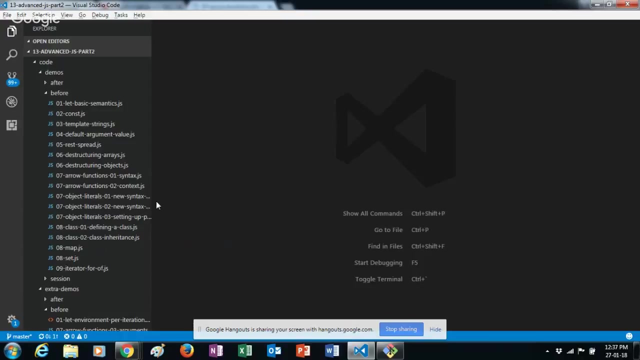 is nothing but proto obj. this is proto obj. okay, so this is obj 3, whose prototype is proto obj. all right, so these are the changes to the object literal syntax. okay. similar changes are also done to class. in fact, class is a an entirely new concept in javascript. 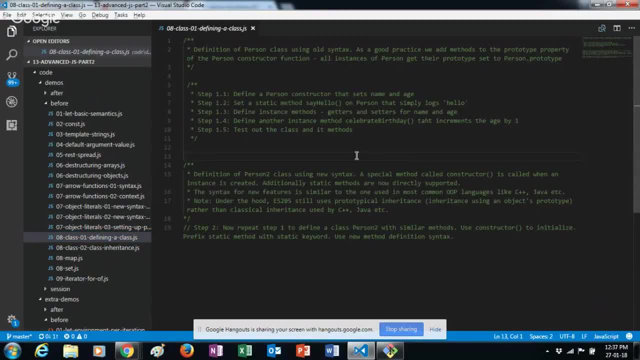 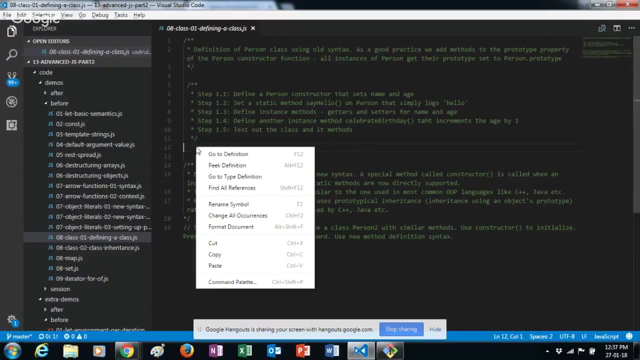 uh, behind again. i'm not getting into, uh, how inheritance works in javascript and how you used to do it in es2011, es5, okay, uh, i'm just okay, probably this. the step says you'll have to do it, so i'll just follow and quickly create one. so let's see how you would define a class. let's. see earlier. so there's no concept of a class as such in java script. there is no concept for jobides, no idea of geeks. so there's no concept or project class before do Como how to combine form into one. so there's no concept of a class as such in MAX. i'm just basically going to throw another class, okay, so 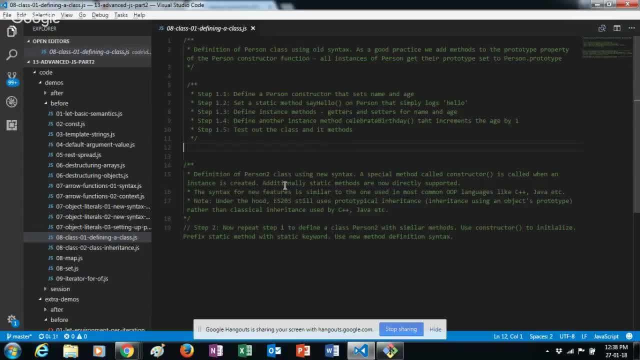 you can scan excel so you can see that. a few things for java script here and retrouver it. and then, if youакome heter, Niger is a two class, so no concept of a class as such in javascript till es5. okay, now es2015 actually brings in the class. 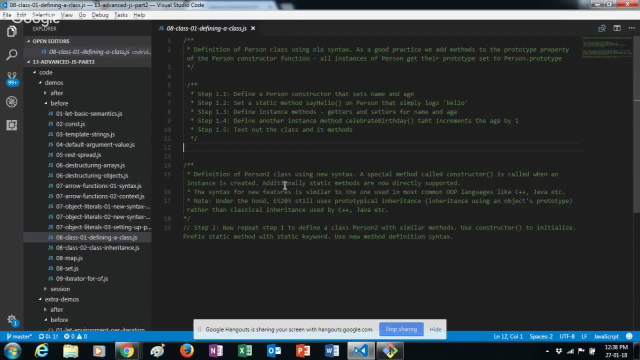 keyword through which you can define a class using classical inheritance, that is, inheritance as the the way you know it, in c plus plus in java and c sharp and so on, in most common object oriented languages, the way you know it, the way we most, most of us, are familiar with. the same way now, javascript. 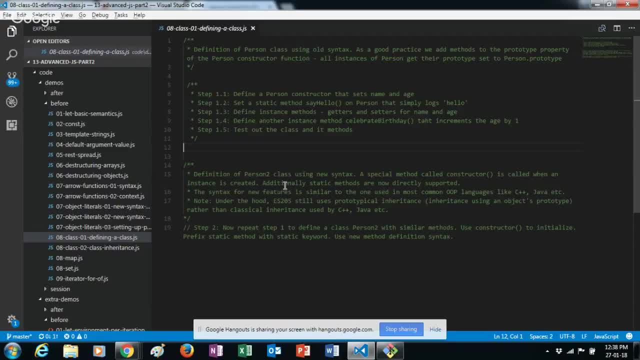 inheritance class definitions work okay under the hood. the way inheritance is implemented is completely different, actually, from the way inheritance works in these standard root languages like java, c, sharp and all, but at least at the level of the developer, at the code level, now, it is the same. okay, it is very, very similar, okay. so let's see the old way. 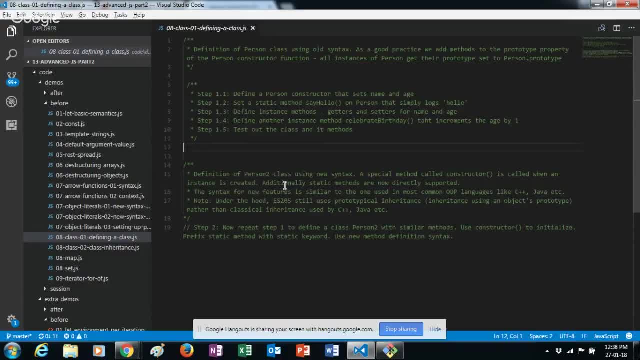 to define. there was no class as such, the way you would implement the concept of a class earlier in javascript and now: okay, so we are going to see that if you have to define a person class, this is how you do. earlier in javascript: no class keyword. you define a function which is: 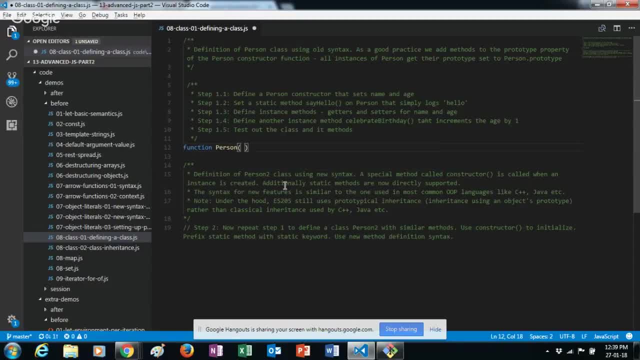 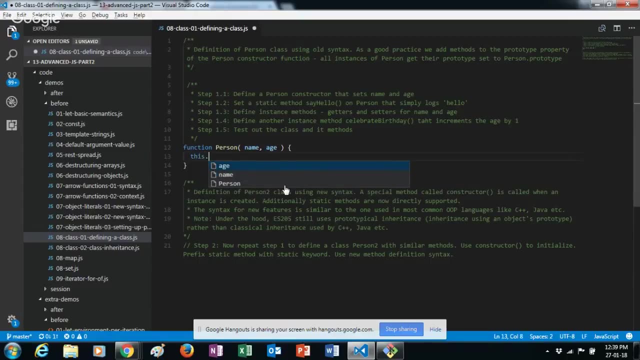 called the constructor function. nothing special about it, except that you're going to call it with a new keyword, always. so a general function takes name and age, okay, and let's say, uh, it sets those. so this is dot name equal to name, this dot age equal to age. 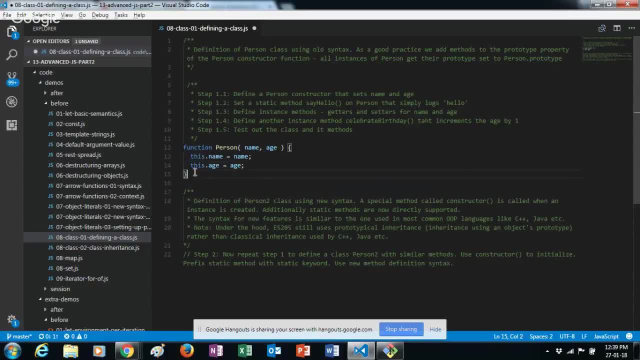 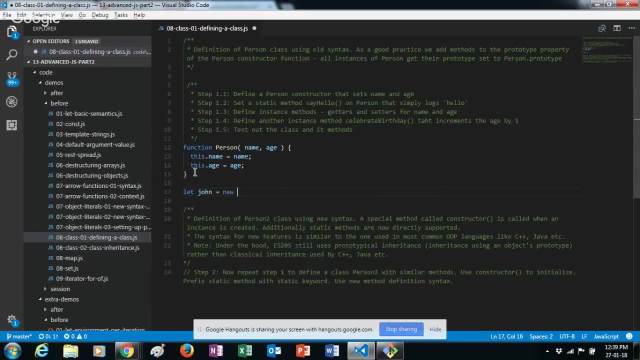 nothing special. okay, the function context, the way the function will get called, is, like you would do, in classical way, also new, followed by the constructor function, actually this time not the class. and then let's say john and age is, let's say, 32.. so this is how you would create in: this is a basic class. 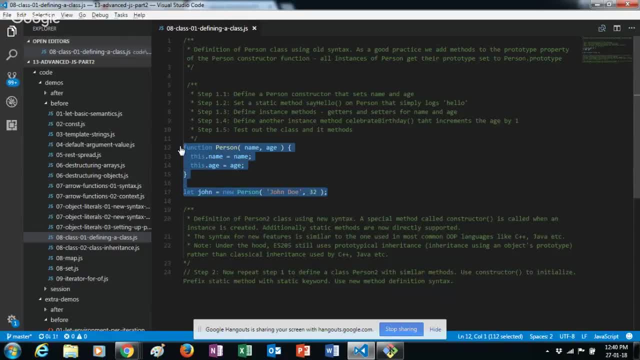 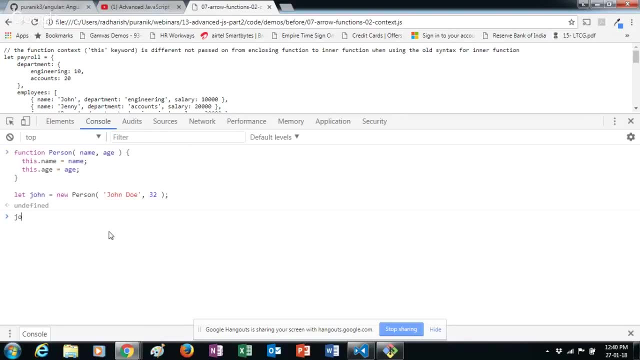 okay, just two properties. so this is what you do in es5 in old javascript. it works. so john is actually an object. now, age properties: you can create new, new persons. for example, you might create gita and okay, and githa be an object. okay, with name and age properties. so 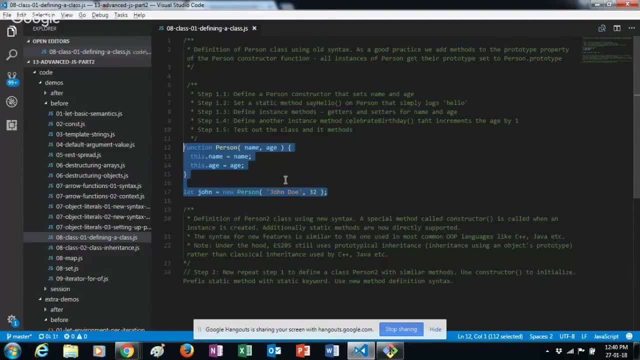 this is how you define a class in es5, or rather from. from the day javascript was born, it had this and this is how you do it all right. so if you had to define some static method that is a classical in a return oop language static method, that is some method that belongs to the class, rather. 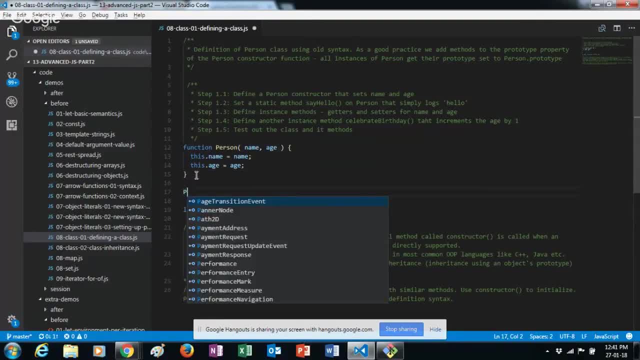 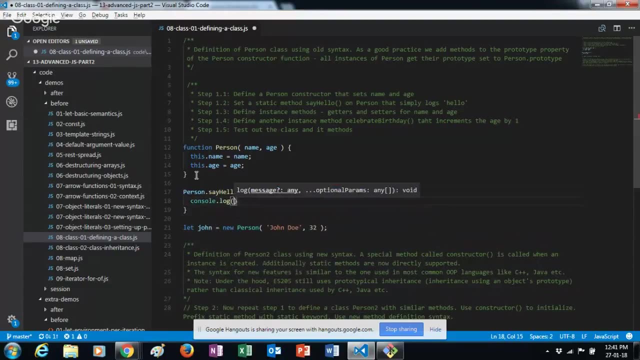 than the objects. so what you do is- since in javascript, even functions or objects- you can define methods for person and all it will do is it'll log hello. it's a dummy, then. it's not useful. but just to illustrate the point, this right you say personclo equal to function. 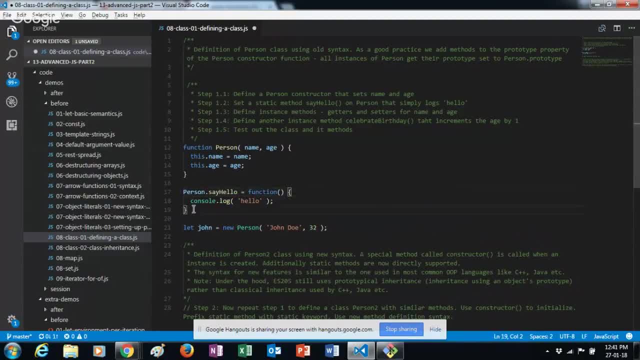 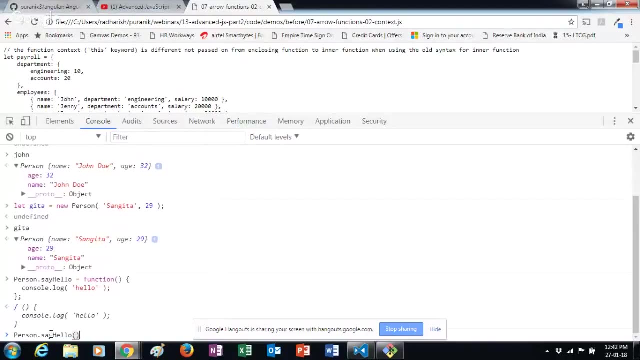 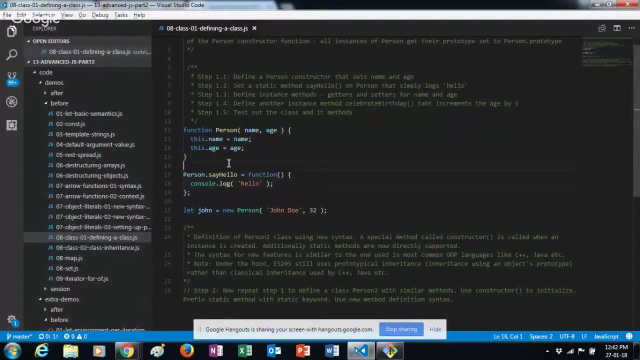 do it then, uh, javascript earlier, okay, so i'm just showing you the different things. so now, if you have this also, so you would say okay, percent dot say hello and it would say hello. so this is a static method equivalent of a static method in javascript old way, so you not yet come to the new way. 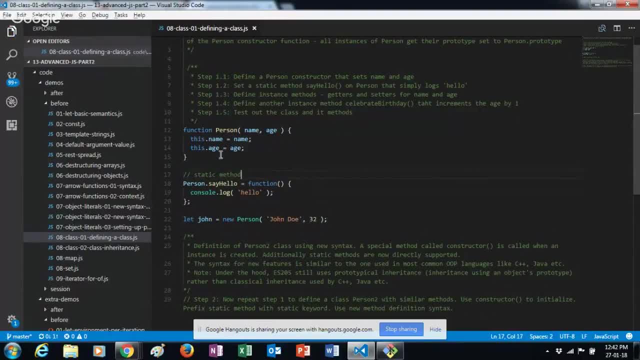 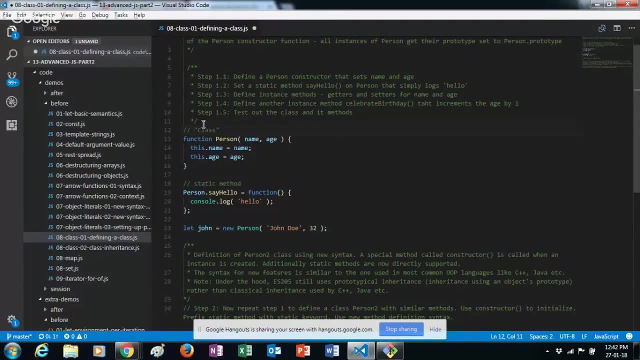 okay, this is a. in the old way you can call it a class, okay, but it's actually a function: call it with a new keyword. so when you come to the new way, you can call it a class, okay, but it's actually a function- call it with a new keyword. so 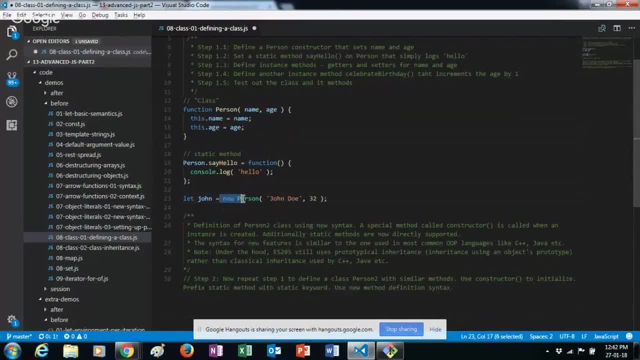 So I'm not going into details. So it's called the new keyword. It's going to create an empty object. that is going to become the context, That is, that this, the newly created empty object, will be this within this person function, So static object would be clear. 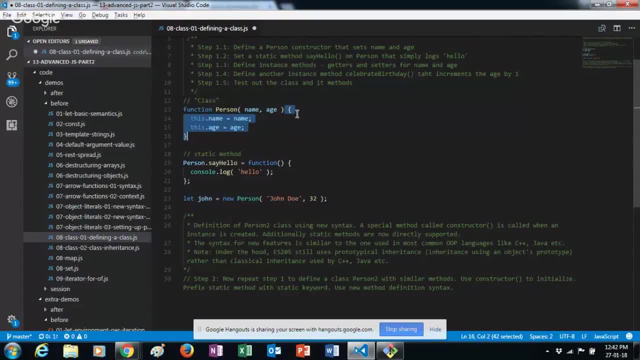 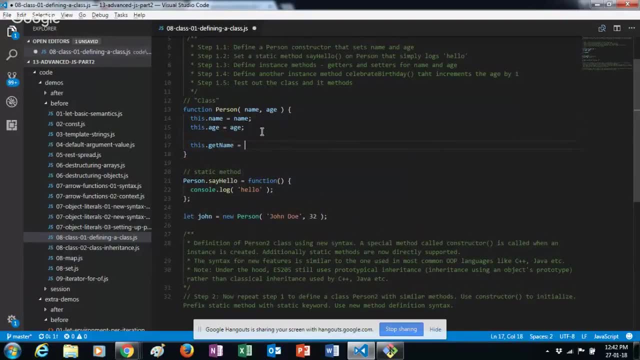 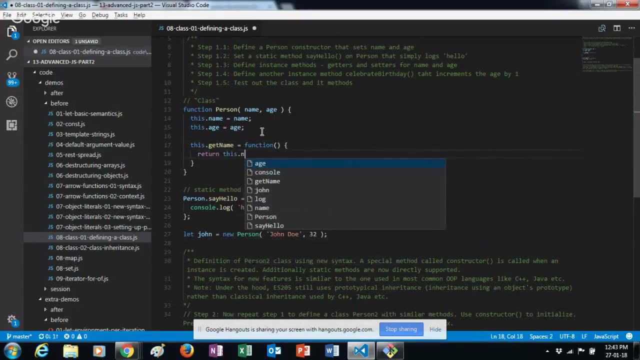 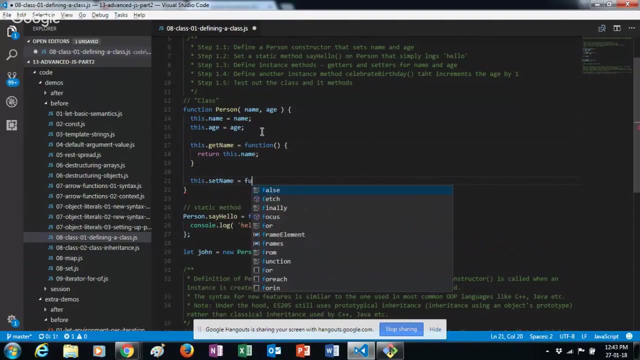 If you want to get us a status, you do something like this. So you'd either do this like this: dot get name. I'll just do for name. So you'd either do like this or you'd either do like this: get us and set us. 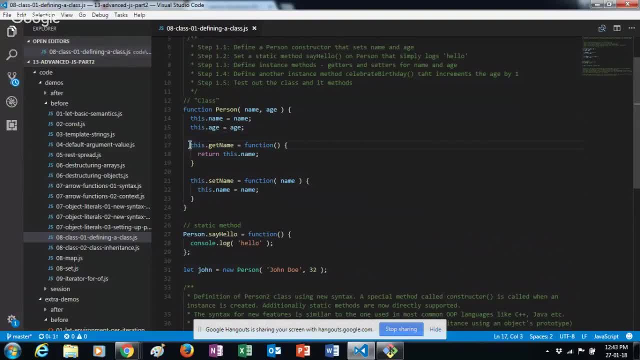 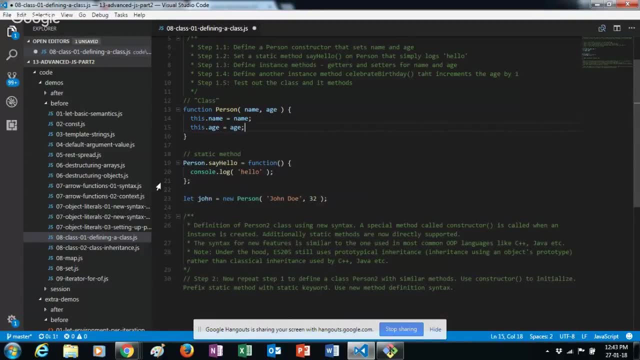 Or what you do, even better is you would create them on the prototype property of the function. I'm not going into details again. This is whole JavaScript. So you, what you do is: if you're aware of it, good, If you're not aware, it's okay. 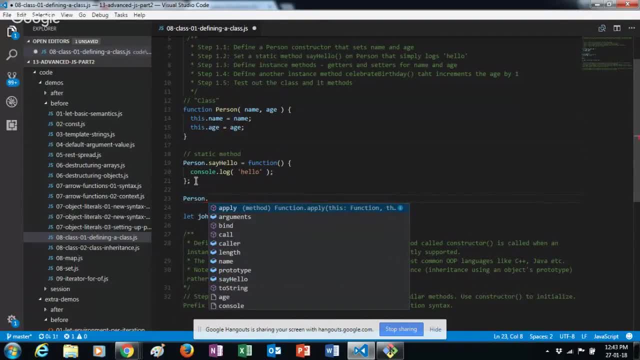 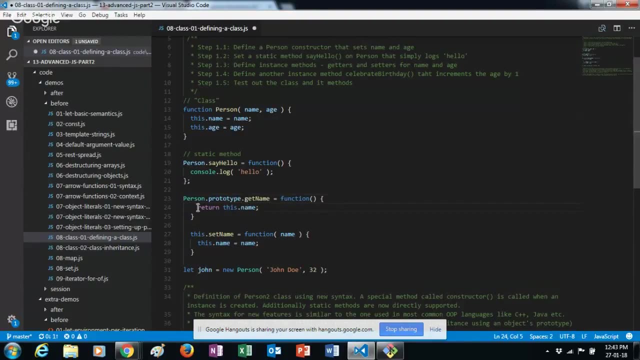 because that's the whole point of today's webinar, which is how JavaScript- later JavaScript- simplifies these things. Okay, dot, get name equals And similarly, here I'm going to create an empty object. So let me create an empty object. 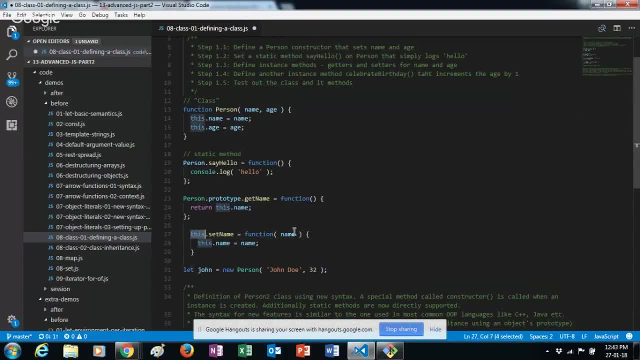 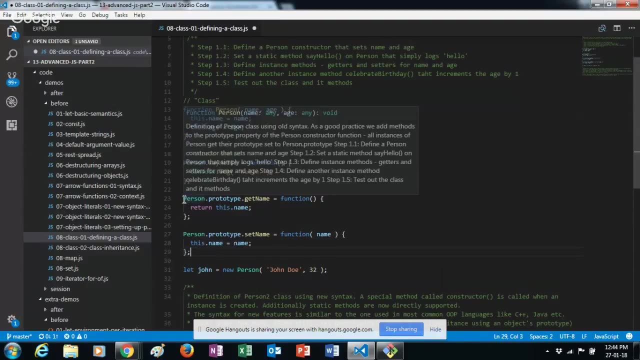 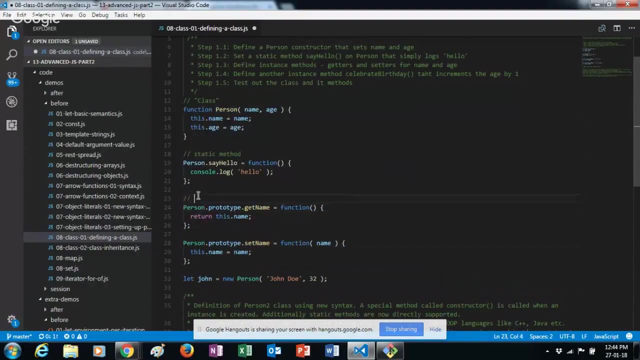 let me create a new object here here: person dot. prototype dot. setname equals okay. so basically get us and set up any instance methods you would usually define like this. so all this is old JavaScript. most common way to define would be like this: all right, let's say 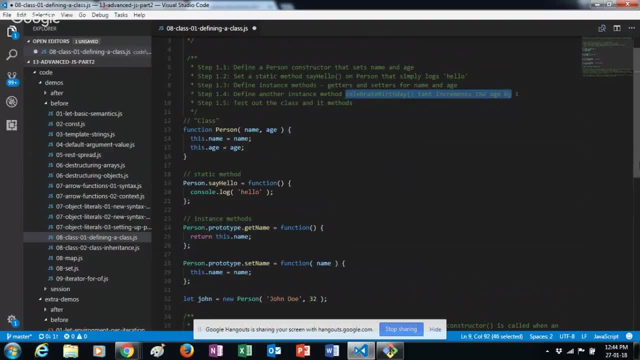 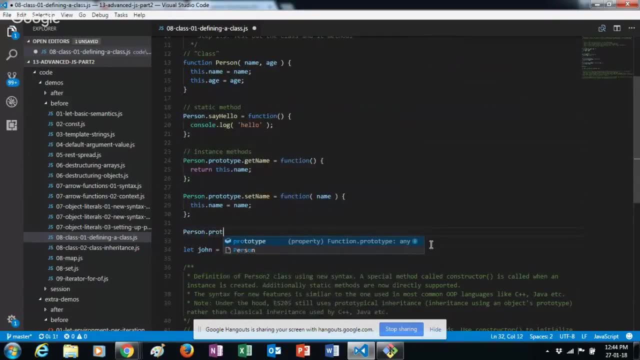 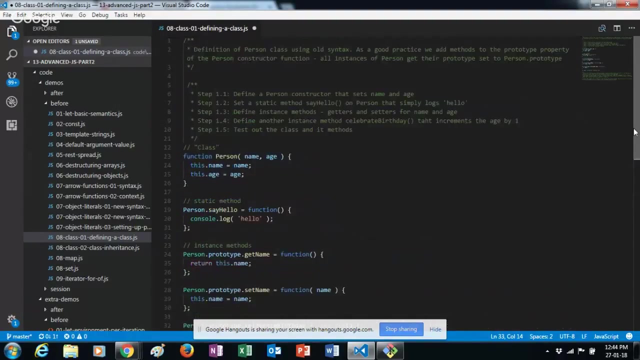 there's one more: celebrate birthday that increments the age by one. so how would we try that? we basically say something like person dot, prototype dot, celebrate birthday equals the function which is going to increment the age. all right, so this is what is going to do and we can test out all the methods. for example, we can check. 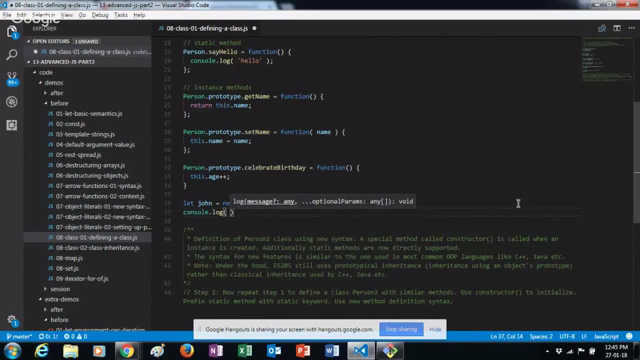 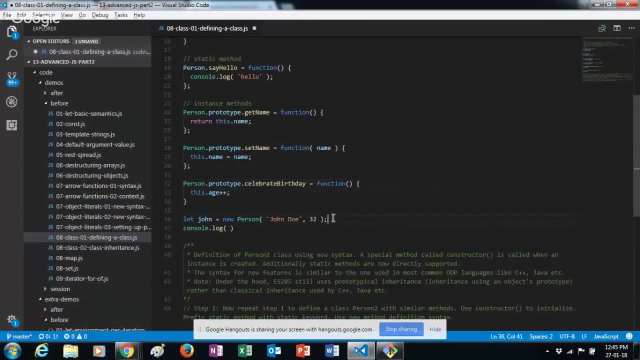 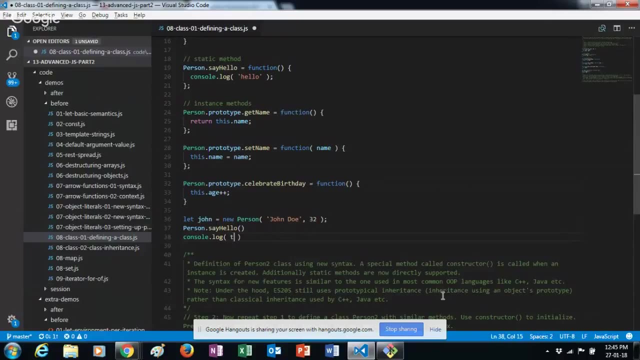 out what is on page. we can check out the static method, which we have already done here. so person dot C LOA. basically that they could. we have already done. checking out the instance methods, we could say, okay, console dot log. what is John's- sorry, John's name? okay. 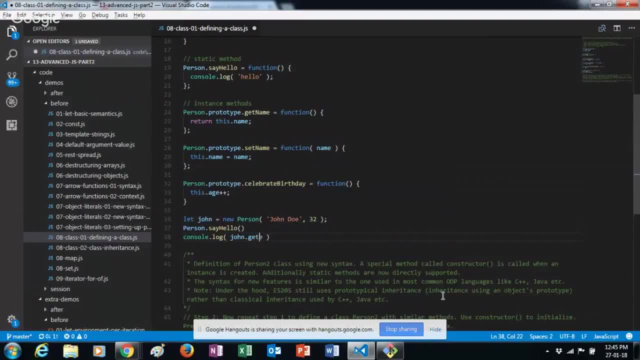 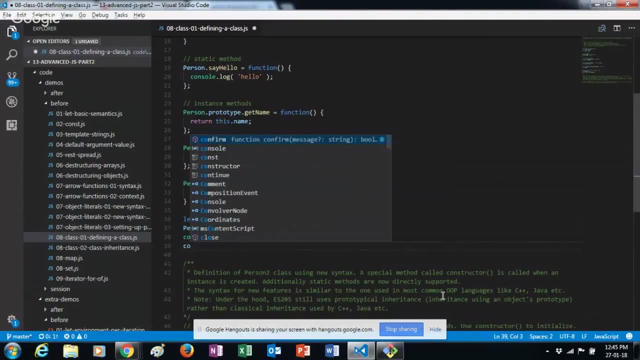 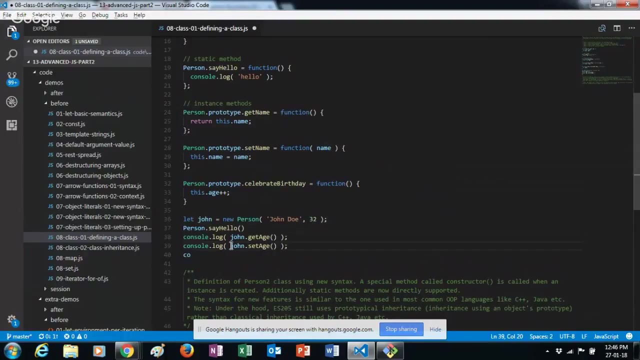 we could get name to get name. let's, let's not use the property directly. it means, similarly, if you want to set the age, or let me actually get the age. similarly, if you want to set the age, or let me actually get the age separate and then test out the age again at the age and then set the age, not 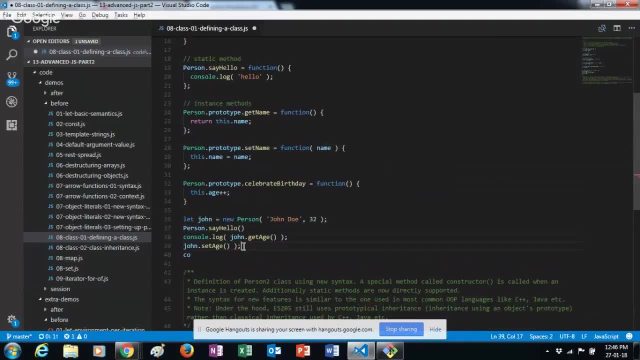 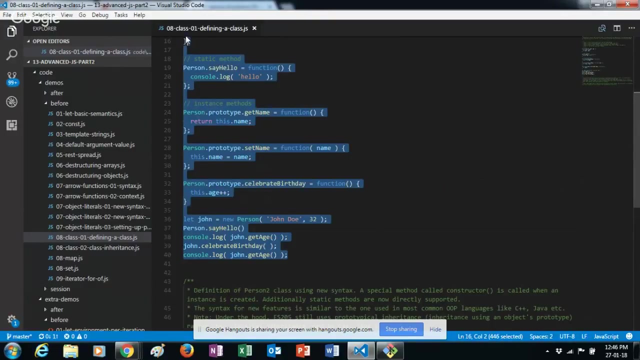 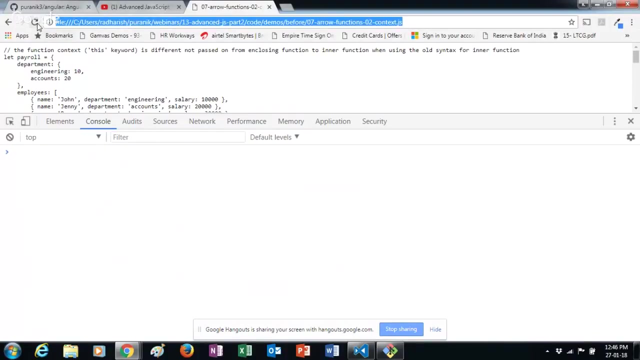 logging it at the edge to. let's celebrate, but let's tell it so age will increase by one. then let's log the edge again. all right, let's test this much out. okay, let's. we have defined static methods, instance methods, all right, so dawn has already. 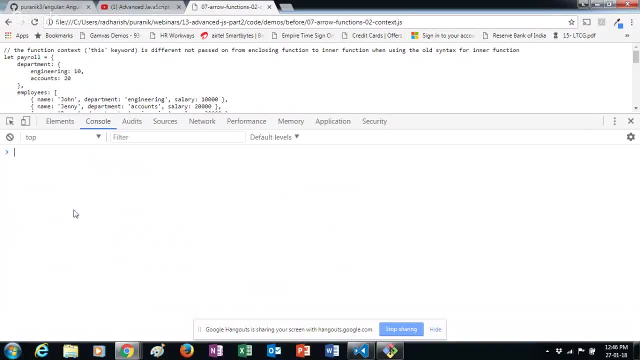 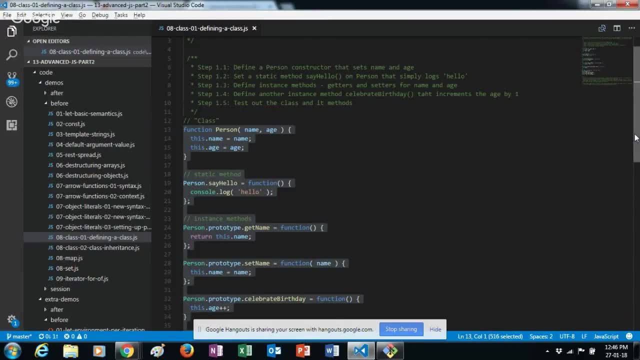 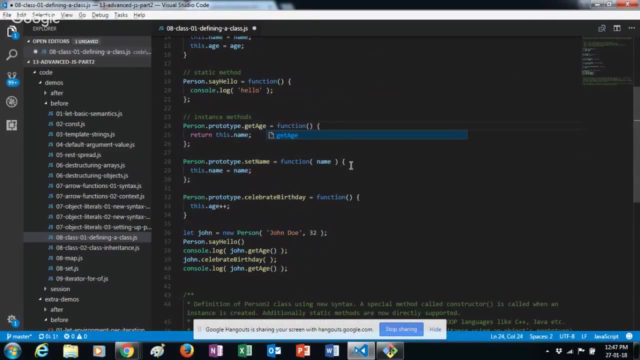 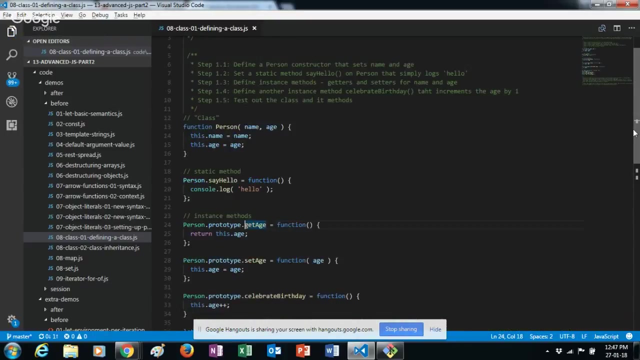 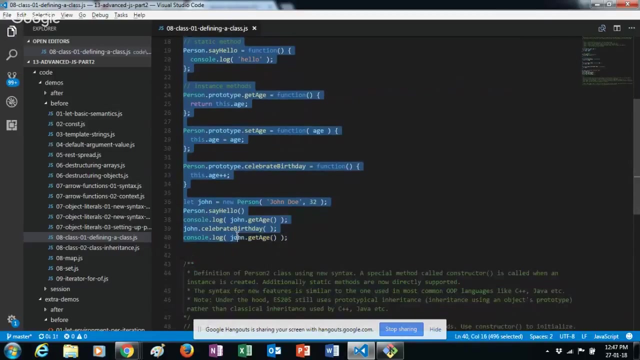 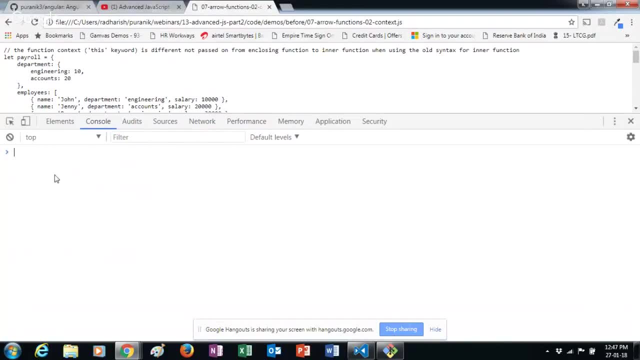 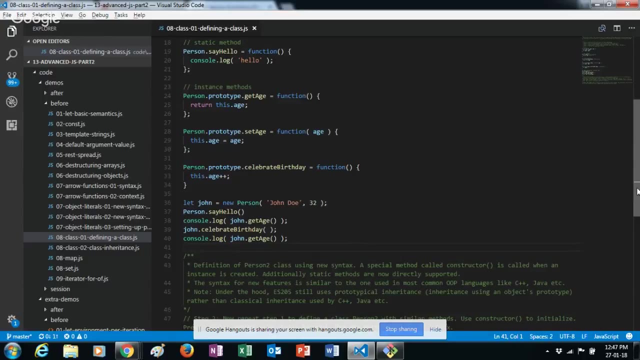 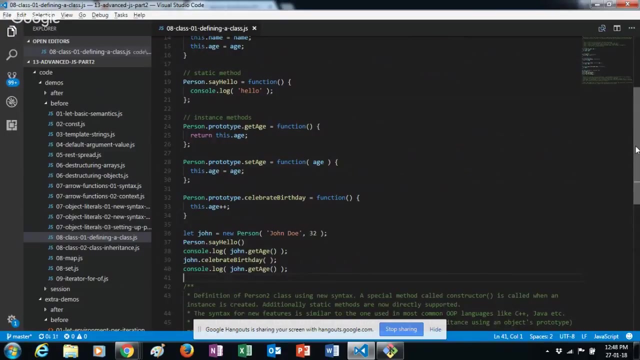 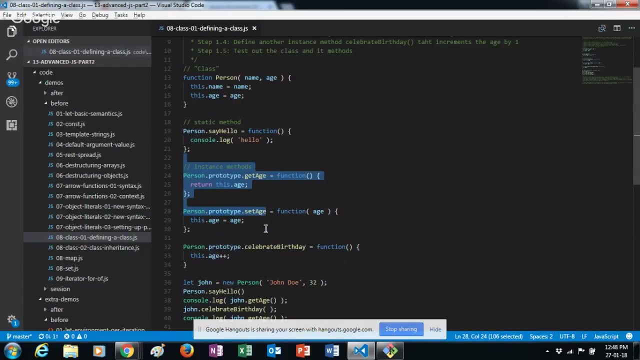 age, age Arrange, Arrange Casヱ Or Tax الث Cas. why Cas 2010? hint, hint, hint. Let's see one thing. I'll landing article class immediately. Look at all this. Why such a complex syntax? Why not the straightforward syntax that other languages use? 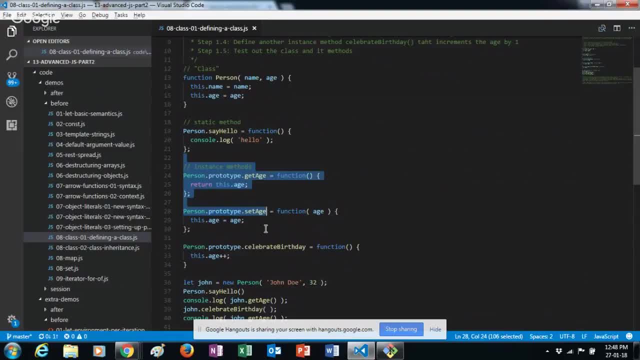 Okay, It's not that JavaScript as such is so complex, but it's more like a familiarity bias. When you come from some other language where the classical model of inheritance is there, it really becomes difficult to adjust to this kind of syntax. So what JavaScript has now done? 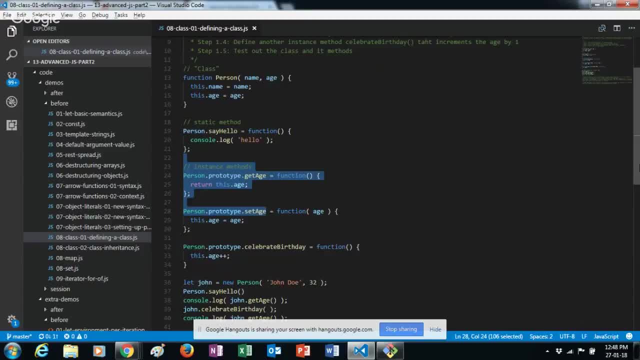 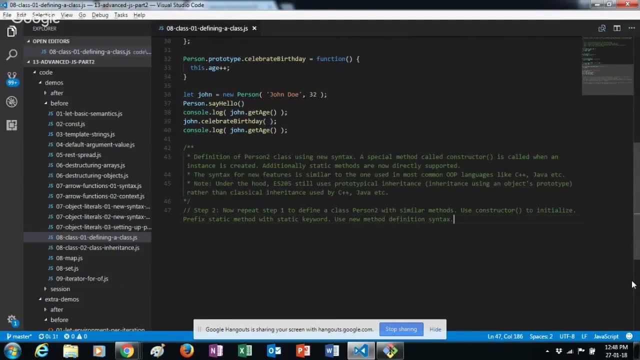 it has given the classical way of inheritance. So what you can do is you can use a syntax very similar to the classical inheritance syntax. So now the same thing. let me translate into classical inheritance syntax. So this is available only in ES 2015 onwards. 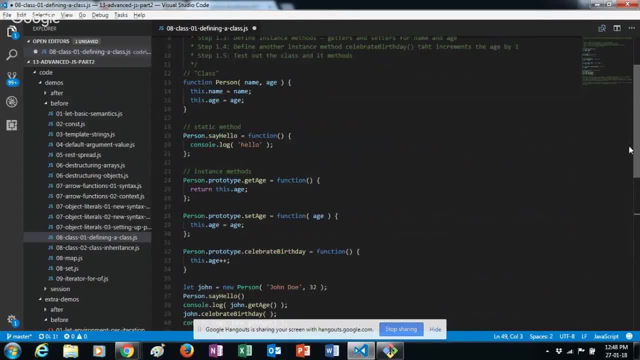 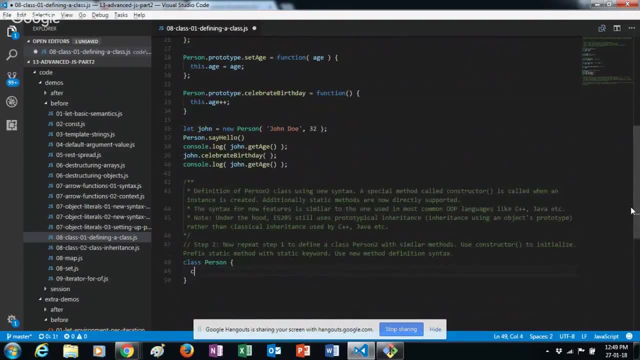 Class person, which you understand very well. So name and age: you don't have to declare it. So members need not be declared The constructor. So you use the constructor keyword except name and age, do that? Okay, it should be called constructor. 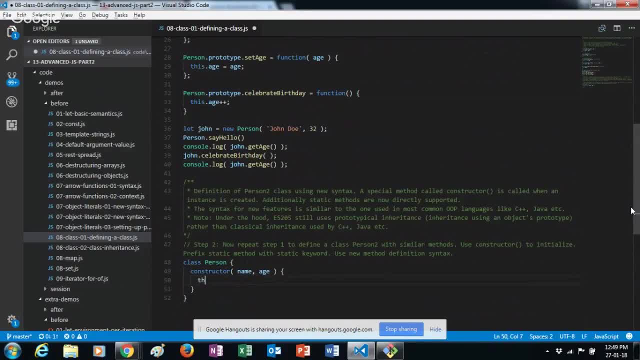 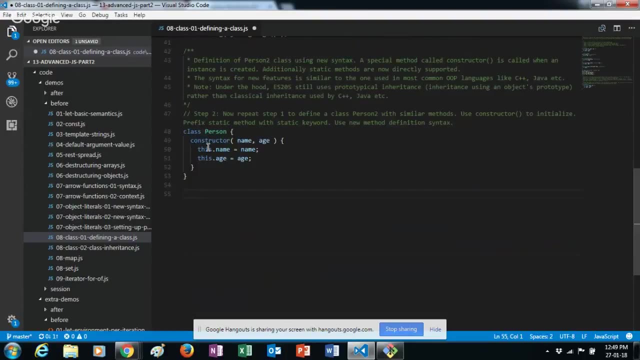 It's a keyword again. So name and age. And then this dot name is equal to name, this dot age equal to age. So that's the constructor part. Let's go step by step. Read: no semicolon after class. So that's one method. 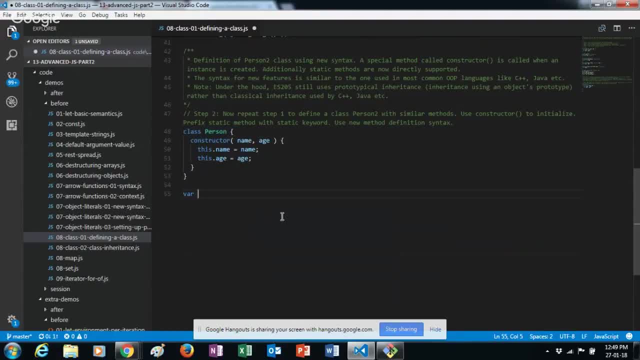 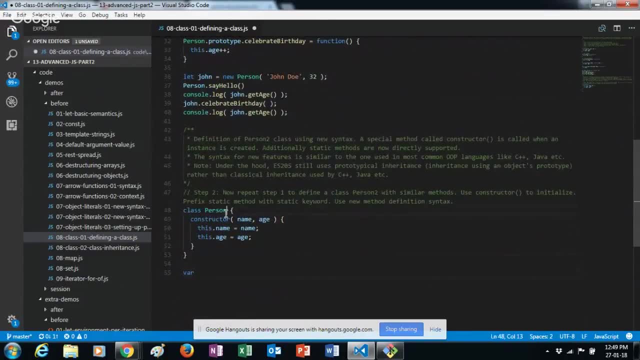 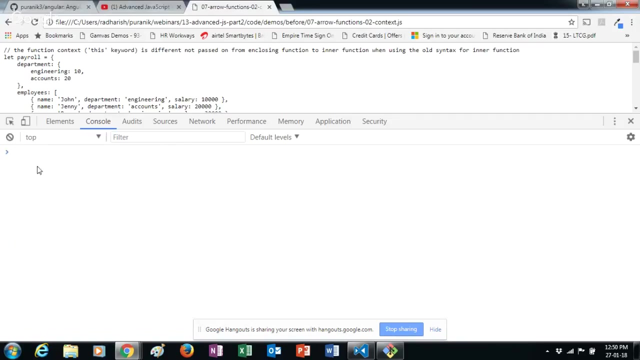 The constructor method. Now we create, let's say: but there's already a person here, So I'll just name this person to this class. So let's say, it will have now the character Beautiful, All right. So this syntax, that's when compared to, it's very similar to color classical. 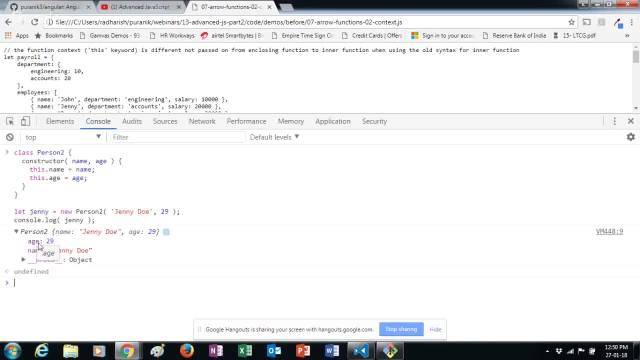 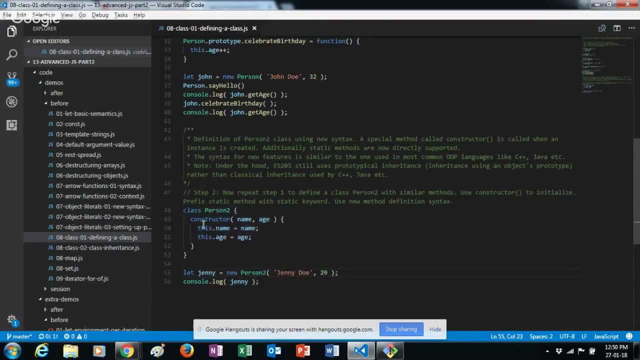 So Right, So you can see that person. they mean, these object has been created Really. Wow is basically, uh, of type person two, of class percent two. so it shows that. and then jenny has two properties: name and age. they need to query name. so this is straightforward, right? 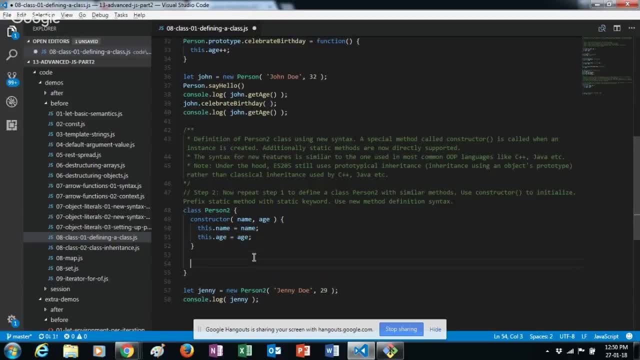 and then you can create instance methods, also in a straightforward fashion within classes, so you can say: get name or get age. yes, this is syntax which is very similar to the object literal new syntax, right? so you just say: get age. any arguments you can take in here, you don't have arguments for get. 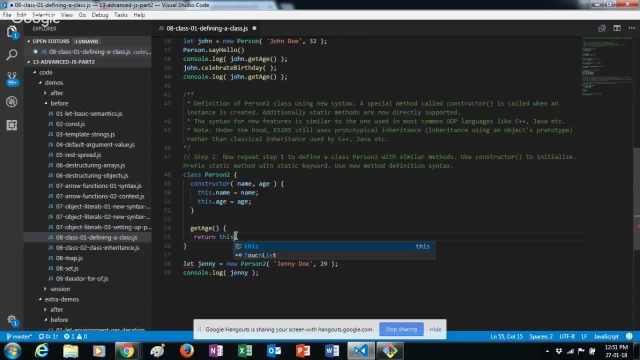 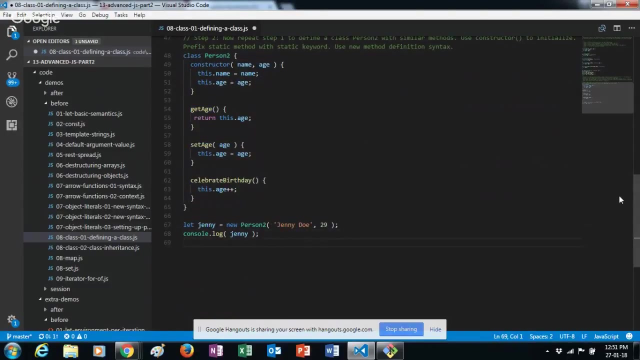 so return this dot age, okay. similarly, set set age: takes an age and sets the age. similarly, celebrate birthday: it simply increments the age. okay, so this is very much straightforward and very much like your normal loop languages and it works. so we can do the same thing, okay, so i'll keep the tests. 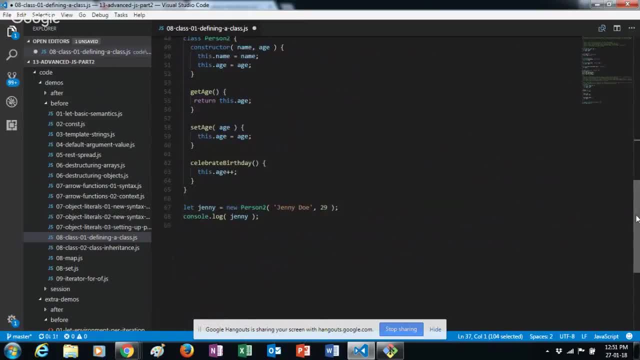 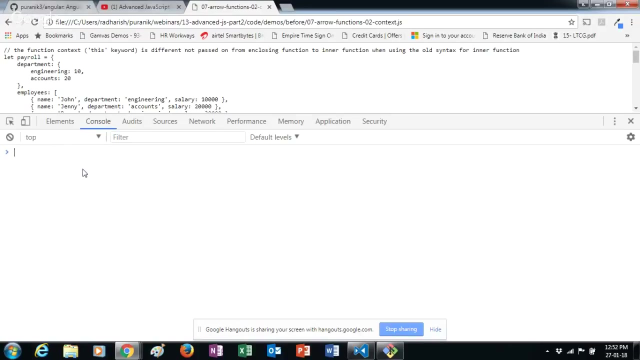 say hello, that we haven't done yet. let's see how to do that too. all right, so this is going to throw an error right now. okay, but i commented for timing, okay, so all right. so reference error: john is non-defined. okay, so it's jenny. 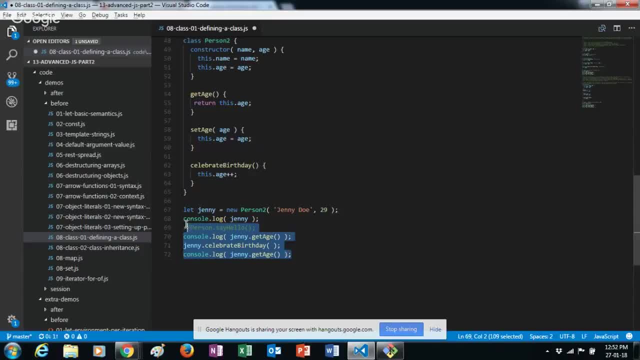 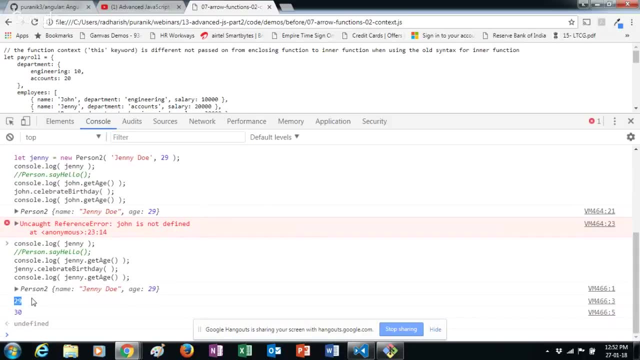 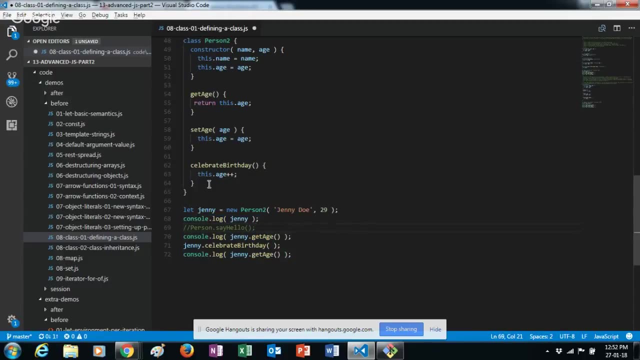 is wrong. okay, all right. so reference error: john is non-defined, okay, so we can see everything. i can see everything is working. 29 after celebrate birthday has become 30.. so this is the new syntax. now, if you want to define a static method, let's say hello, like we did so. 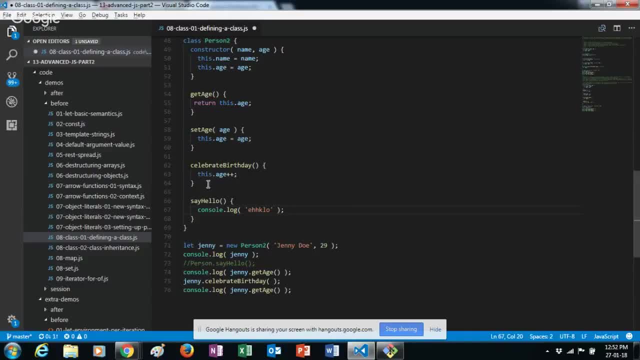 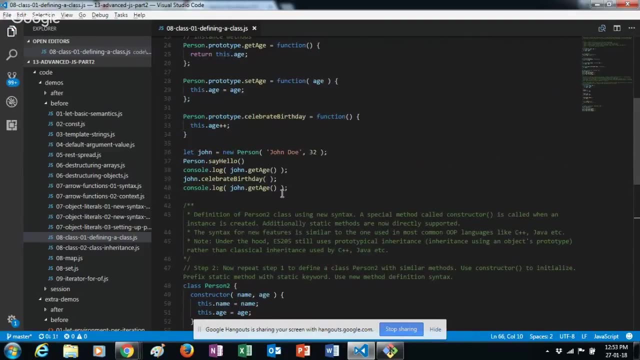 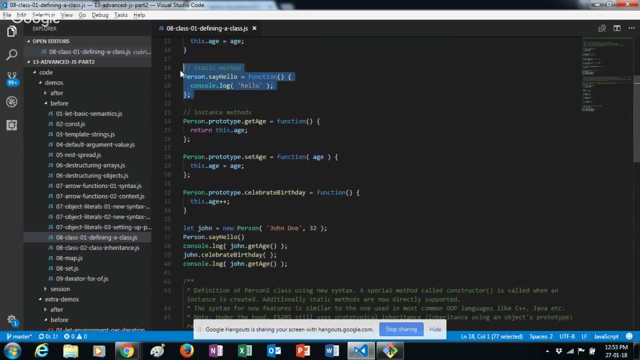 before you that say hello definition, which is just going to log hello, just need to include these static keyword. so I say static much more obvious than something like this. a person again looking at this static method which is defined this way will get really confused. you are saying function, a person is a function and suddenly on the function, 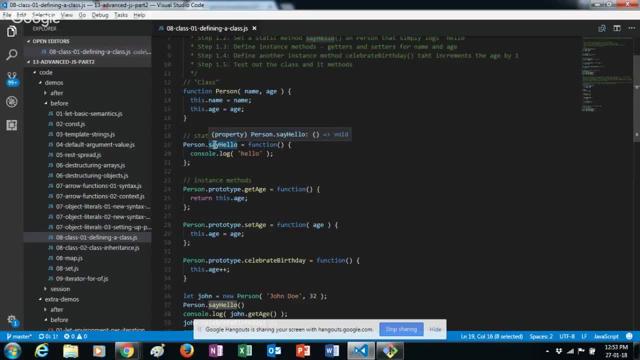 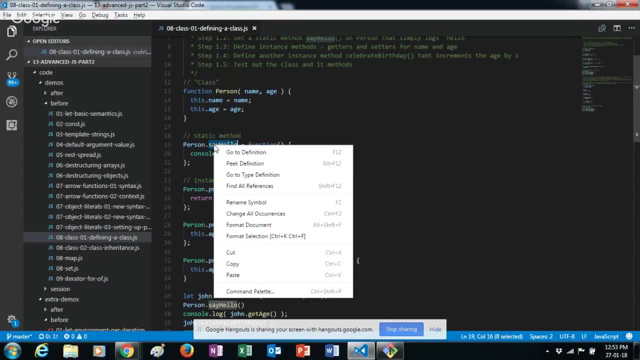 you are setting a property called CLO. how is that possible? how can functions have properties? this may this will be a question that anybody coming from other languages will have. in JavaScript, functions are also objects, so they can have properties and we are making use of that feature. 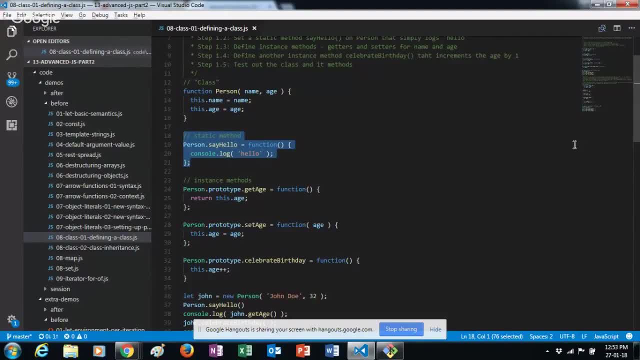 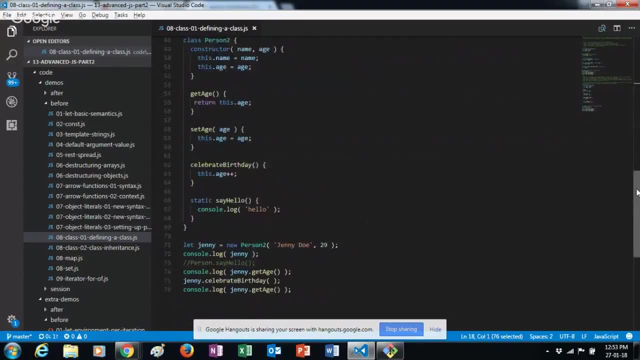 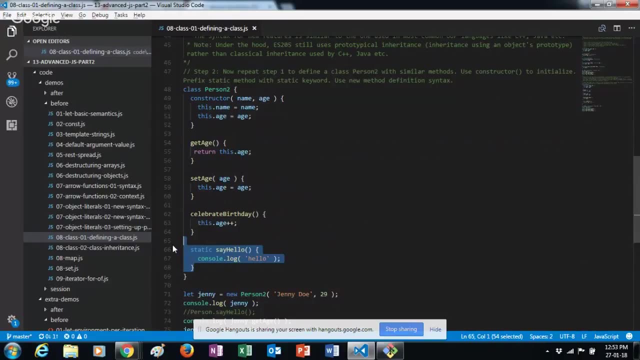 to actually define something like a static method in this case. but for a person coming new to JavaScript, okay, that will be really confusing. but this a person coming from a background of Java or C, sharp C++. Okay, This is very straightforward. you just say static and then name of the function. and now 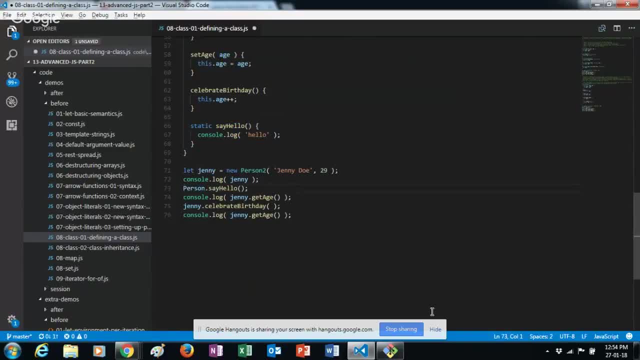 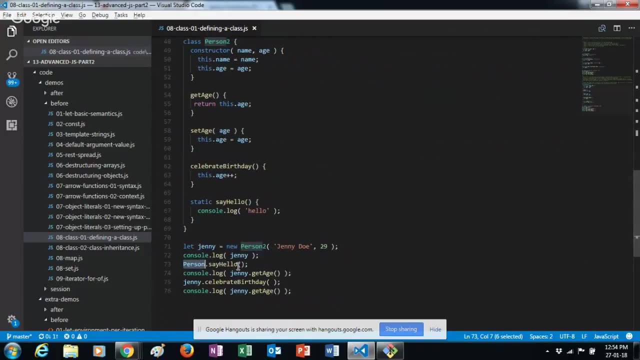 that function becomes a property of the of person, so you can say personhello. so instead of you cannot say jennyhello. it's not an instance method. you have told static, which is why you have to call it on the person class and not on the object, so there will be person. 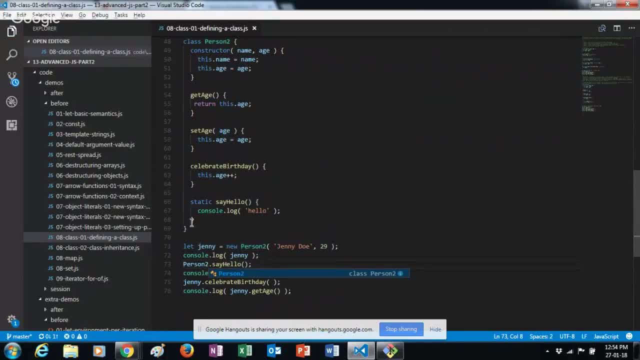 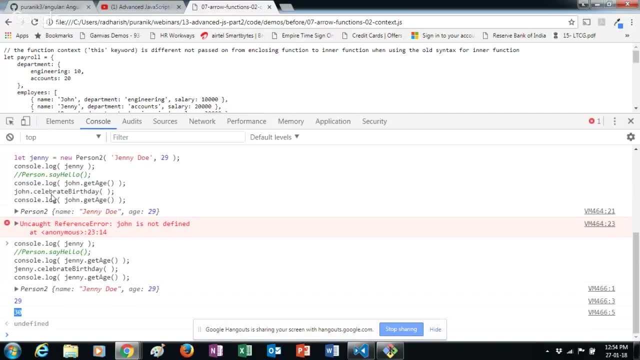 two dots here, okay, so let's just check that out also. All right, it's almost time, so I'll stop here and continue later, so I'll just complete this, if possible. we look into inheritance next time, though that's not in the plan. there's an extends keyword also, so you can see it works. basically, hello is come, so that's a. 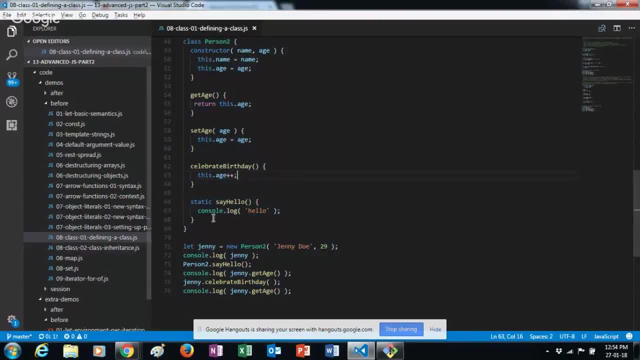 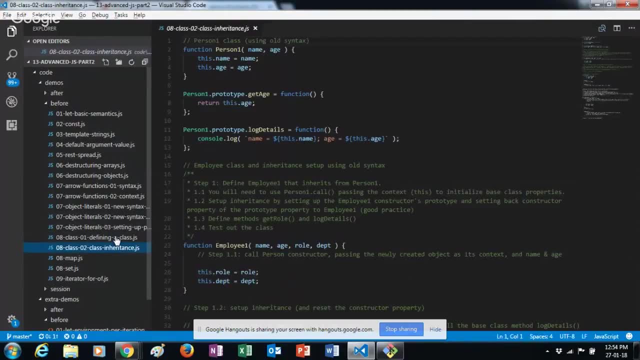 static method. all right. oh, it is in the plan actually, so we will be seeing inheritance. we have seen Right now how to define a class. in fact, maybe I can just quickly show inheritance also if there is time. Yeah, let me show inheritance. so we have person one: okay function. person one accepts name. 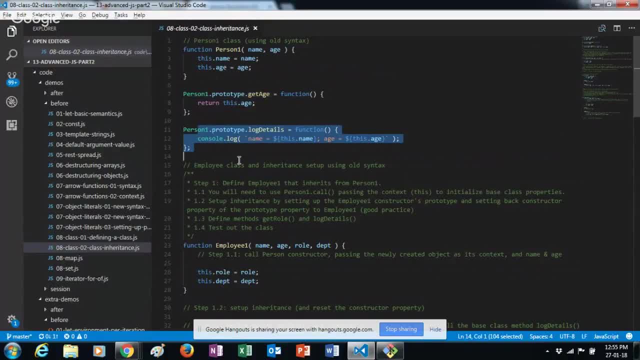 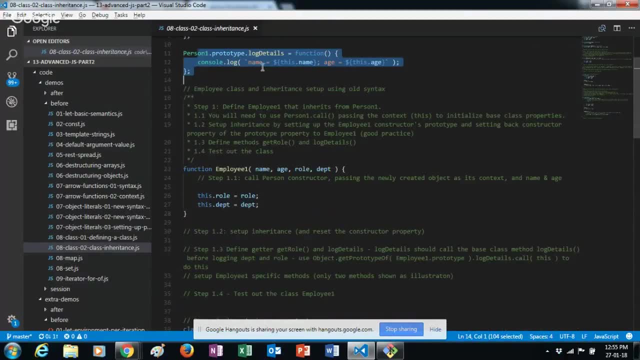 and age same thing: get age, and this is the old way. this is how we do. in the old way, inheritance would have been very difficult to establish. for example, this is a person and there's a lot of details. Actually, I think it's better to stop. 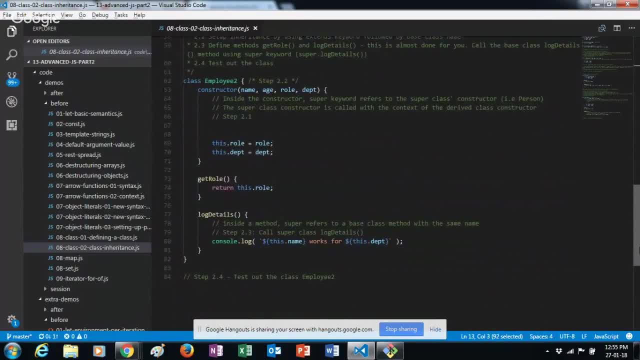 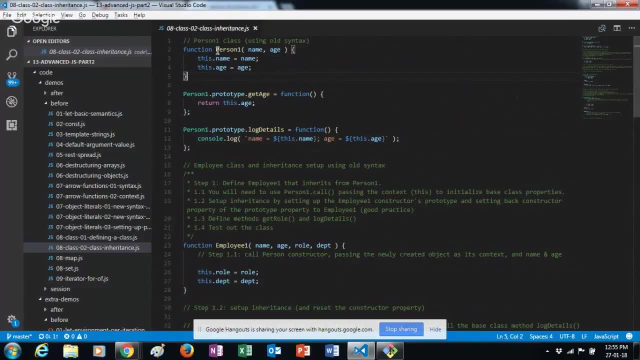 No, because this is going to take some time to explain, all right, so I would require some time. so the next time we'll see how to inherit in ES 2015. that is, using the extends keyword, you'll see map set and promises how to. how to handle promise. asynchronous code, that is. 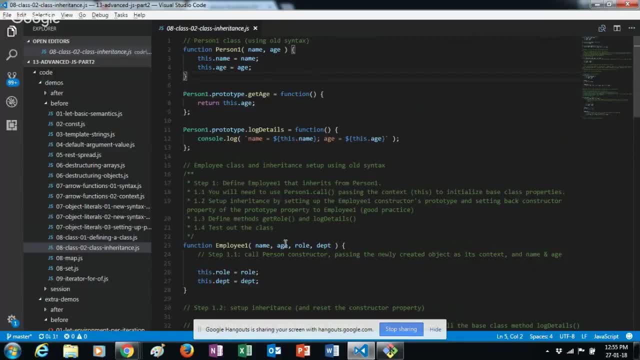 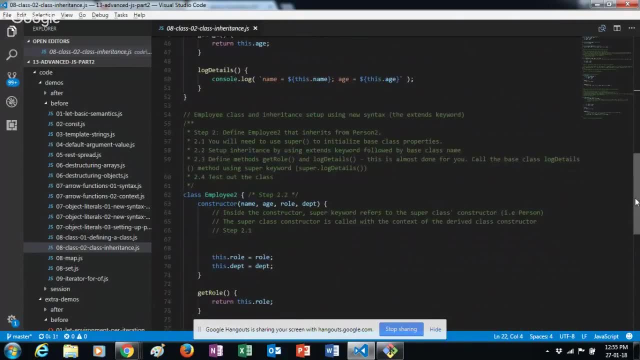 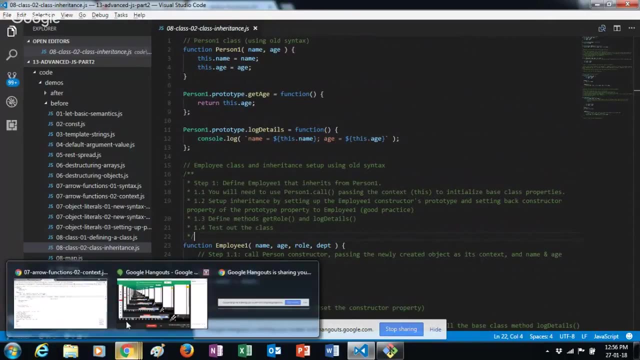 through promises, async await and generators. okay, so I think that's about it. the time is up for this, For this webinar. I would have liked to continue, but there is a time constraint, all right, so I'll stop here for today. I'll take your questions for next five to ten minutes. 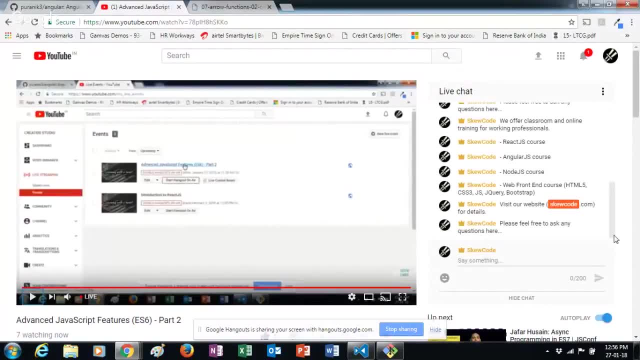 Okay, any questions? I hope this is clear, Whatever we discussed. if something is not clear, please do let me know. I can help. you guys can quickly go through whatever parts are in here. okay, we can. please feel free. please don't hesitate to ask any questions and that's for to answer your. 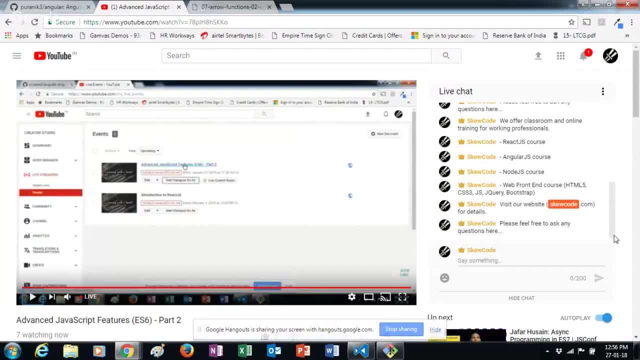 questions and I would be happy if you take away something from this webinar. so please do ask your questions if you have any. okay, what is the use of prototype and object literals? I'm not clear. okay for this. some Vishnu has the question. this is question is by Vishnu Vinayan. Vishnu do you, are you already aware of? 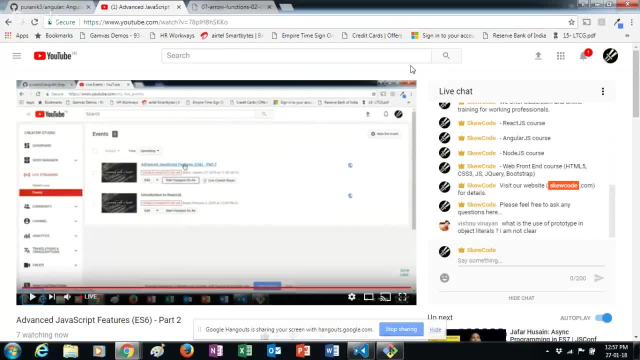 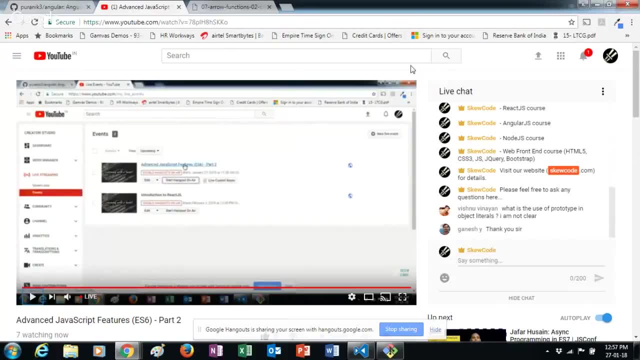 Vishnu. thanks Ganesh, if, yeah, if, if you are gay in a hurry, guys. I am NOT going to take up any more topics. this is just a questions. feel free to leave the webinar. you, you will get a link to the recording after this. you're not ever, alright, let. 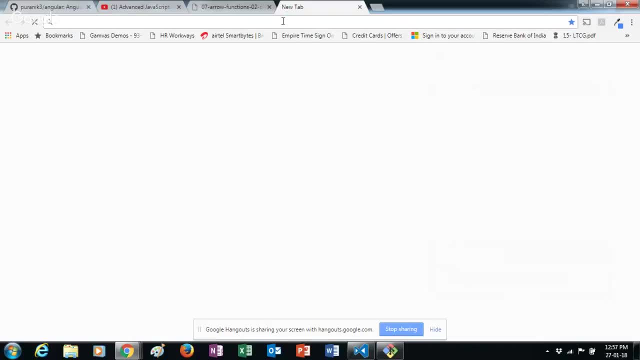 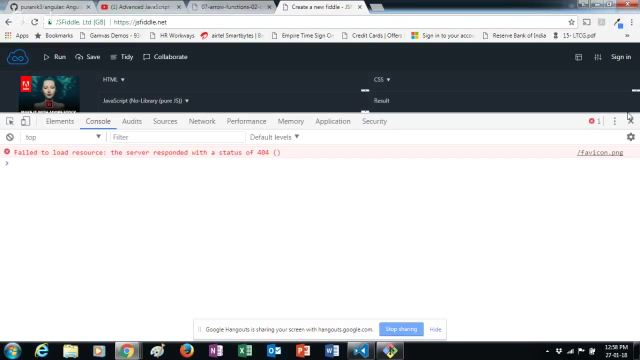 me quickly explain it then. so let's open some editor like J's fiddle. let me actually do it off here itself, or actually let do so. I'll open up this fiddle where I can experiment. you can use whatever you like. yes, fiddle code, pen, right and all right. so in JavaScript every object has something called a. 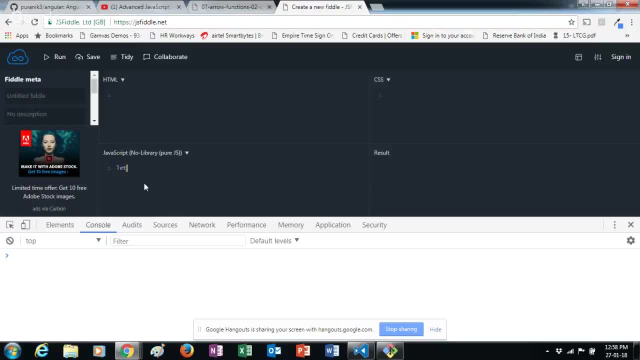 prototype object. so, for example, let OBJ, which has property a1 in JavaScript, this is considered an object as a bag of properties, bag of key value, perhaps, nothing more than that. don't compare them against objects and other languages, for now. so you're creating an object with one property, a, whose value is one. 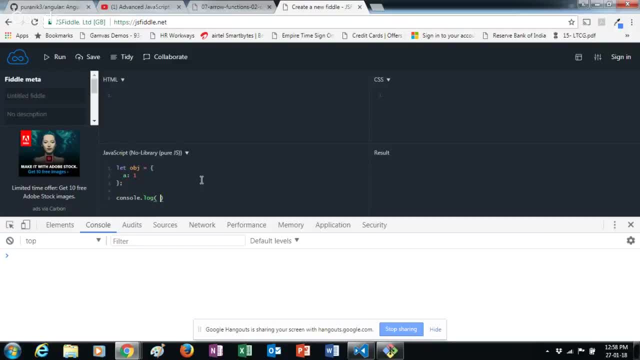 all right, and if you lock that, all right. if you log that, you will see that a has something apart from the a property. it has one more property called underscore, underscore, proto, underscore. okay, this is not a standard property for an object, though most all browsers will implement it. okay, all browsers do implement this, but it's not a standard. 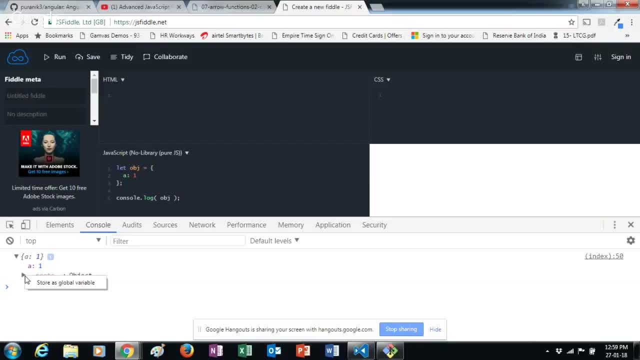 it's not that they have to implement this property and it has to be named this way, but what it should have is something called a prototype. so just like you have a father, you have a mother. okay, every object in JavaScript has exactly, is related to exactly one more object that is called a prototype. okay, so 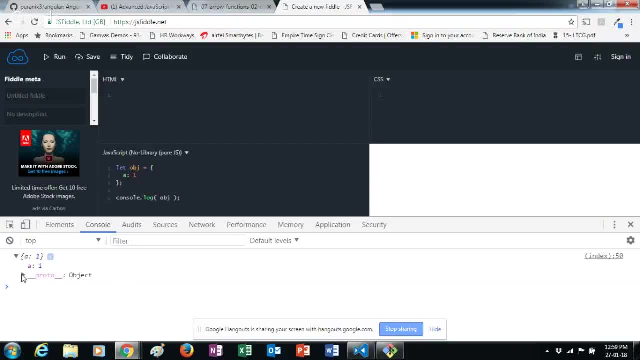 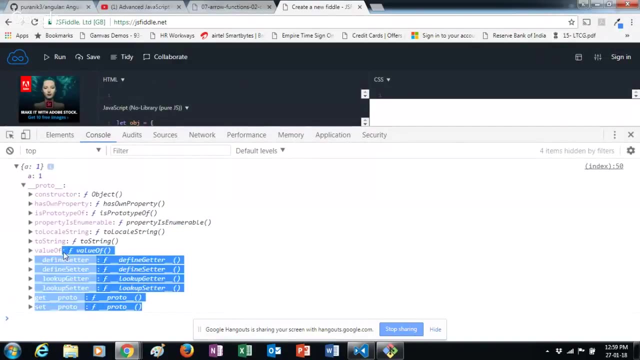 there are. whenever you create an object, it is related to another object called the prototype. now there is a default prototype object for all objects in JavaScript. let's do this object which has all these 10, 12 properties. whatever constructor has on products, it's there is. this is the default prototype object. so this a1, the object that 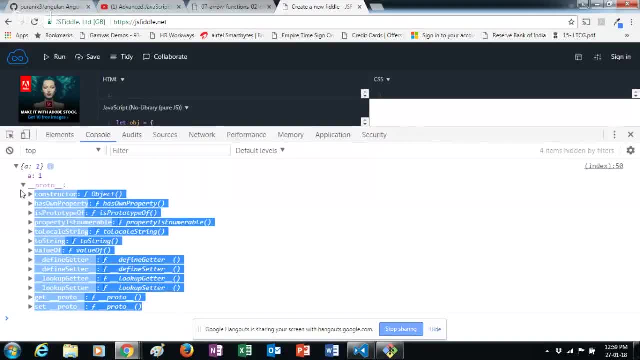 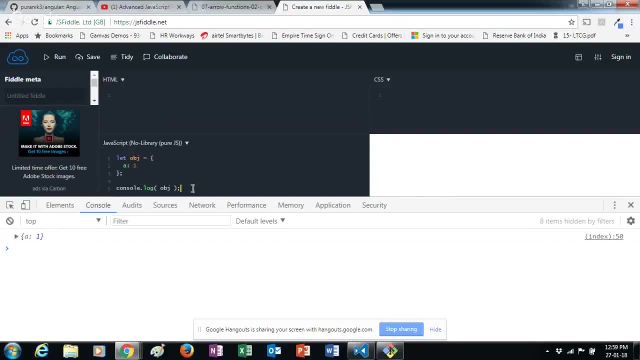 you created is related to this object which has these properties. okay, so that's one thing. all we are saying is okay. by the way, just to give a flavor of what prototype is. you're not going to discuss in detail. so what that basically is is you check out what the prototype is, what 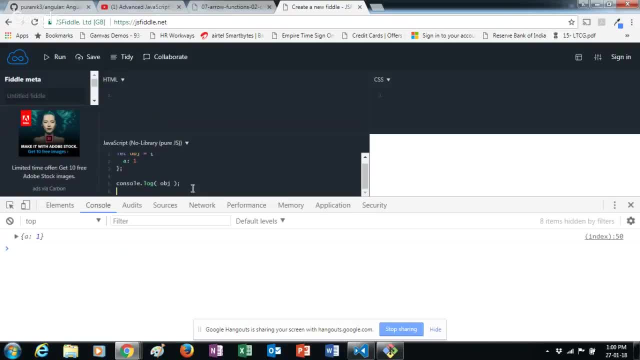 it is for actually now in this object, have we created anything called house on property? no, that is only a property called a. but if you check out OBJ- okay, not has own property and sold out log for busy about a straight endorser who has own property, is. this is rather power of JavaScript comes. has own property and 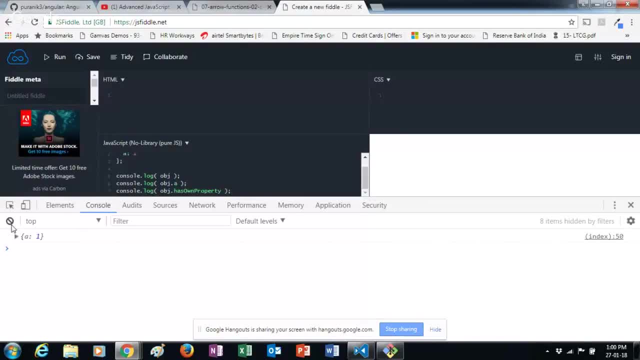 you will see that that also exists. let me run this okay. so you see that is a fortune property and a function. it's a function. it's not saying undefined, because if you have tried out something like objb, that would be undefined. for example, if we try out objb, that will give undefined, because 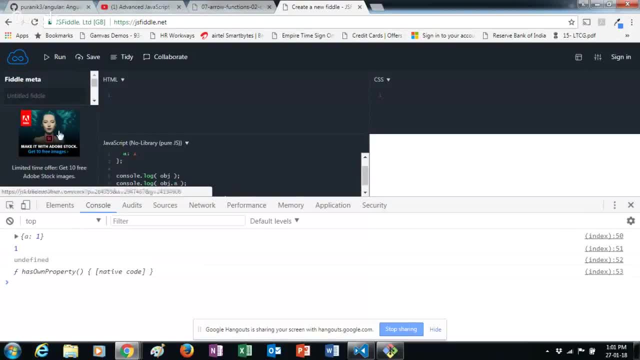 there is no property called b. right, there is no property called b, so it's undefined. a is one, b is undefined, but has own property is not undefined. it is a function. now where did this come from? this came from the prototype object. see in classical oop language. you know that if 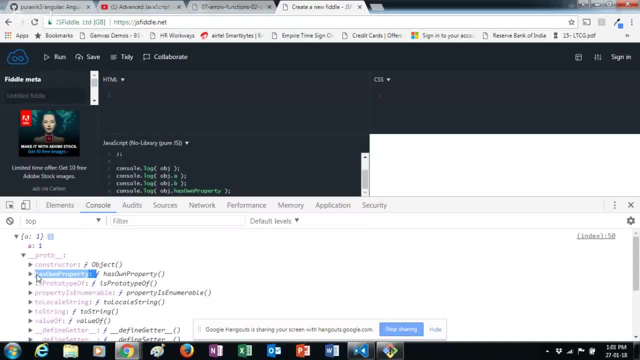 employee inherits from person, then employee will have all the methods, or at least all the protected and, in a standard loop language, all the methods of from the base class. here in javascript there is no concept of classes. objects inherit from objects. so you can see that our object obj. 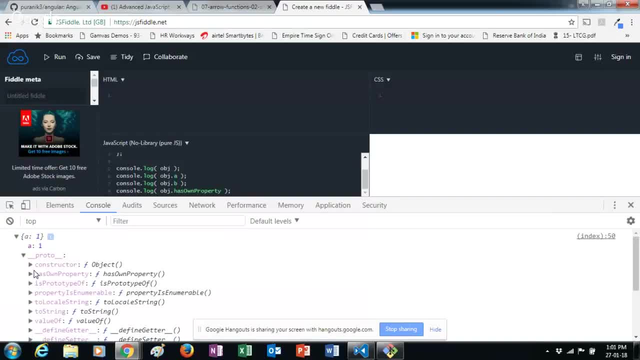 it has access to the properties and functions methods of the hazard property which is on the prototype, can be used by obj. obj dot has one property, okay, so that's the gist of what prototype is. so in javascript there is no class class inheritance because there is no concept of a class. 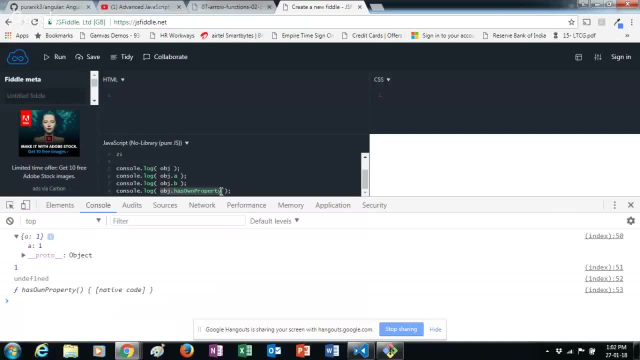 itself. even the whatever class we saw today is actually under the hood. it is actually still using a different model of inheritance called prototypical inheritance. okay, so we are not seeing that. but that is basic standard. uh, javascript, uh concepts in javascript. so we are not seeing that. 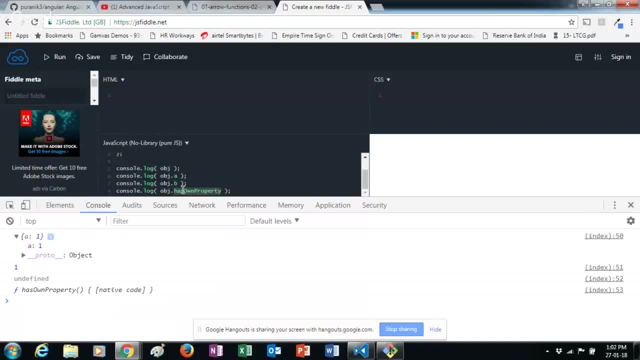 so has on property is being inherited. all right, how is it coming? it's coming from the prototype object. so that's what a prototype object is. earlier we couldn't set the prototype object using underscore, underscore, proto, underscore, underscore property. now you can set it, so you can. 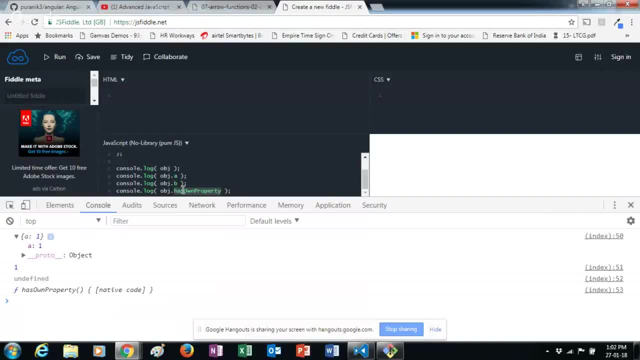 change the pro. so let's say: you can set the model of inheritance. so you can set the model of inheritance- uh, you want to. and just for a joke, let's say your parent, you want to change right. so you can say: okay, my object dot, parent equal to some other object. now, similarly, you're saying: my object dot. 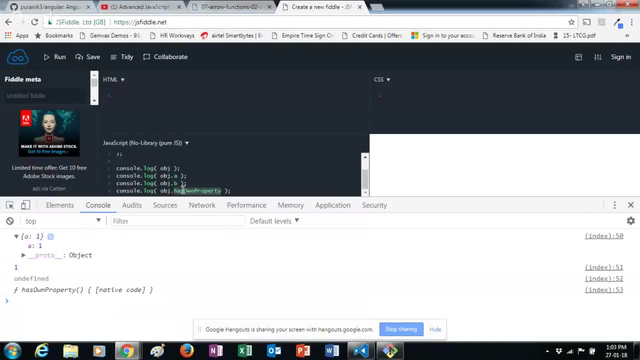 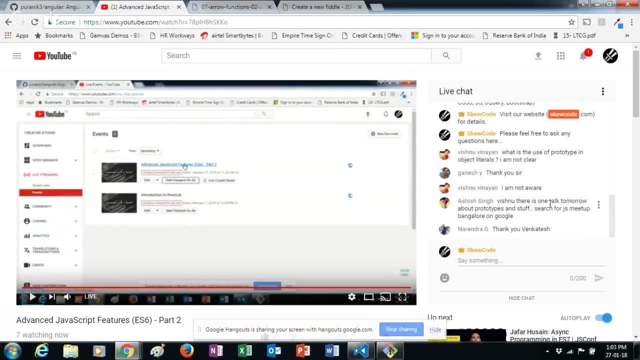 proto equal to underscore, underscore proto equal to some other object. you couldn't do that earlier, now you can do, okay, so is that? uh, does that clear your answer your question, vishnu? so ashish has shared a link. vishnu, that is ashish. i'm just reading over. told vishnu there is one. 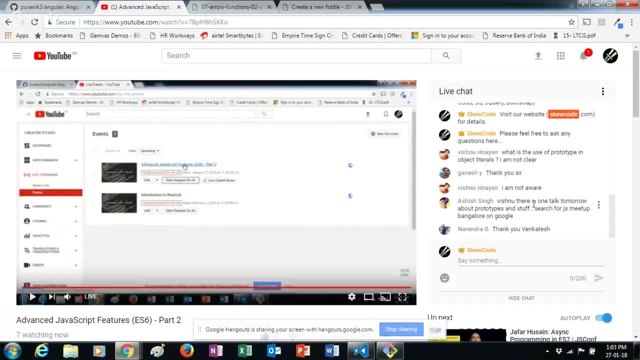 talk tomorrow about prototypes and stuff. search for js meter bangalore on google. okay, so, vishnu, you can do that. all right, but i hope i answered your question. vishnu, i tried my best, but that's basically the how hoop is clear with: uh sorry, is you're clear? 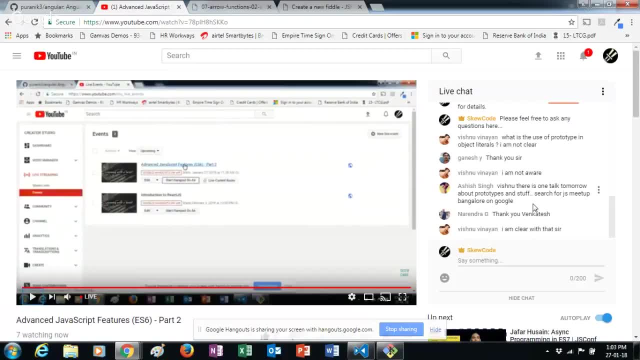 with that. okay, thanks. so how hoop works in javascript? all right, any other questions, guys? so the normal questions. i think we can end the webinar all right, so i don't see any other questions. thanks, uh, thanks to you, thanks, uh, thank you everyone, so we'll uh meet once again. there'll be one more webinar where i'll be covering some of 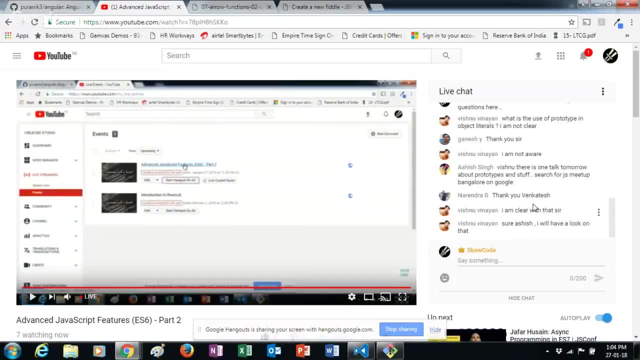 some of the other topics. those will be much more advanced actually. so we'll be saying how to handle asynchronous code using promises, async await generators and stuff like that. all right, modules also. so please, uh, do join us for that webinar too. it'll be very interesting. okay, i assure it'll be very interesting because the topics there are quite advanced and 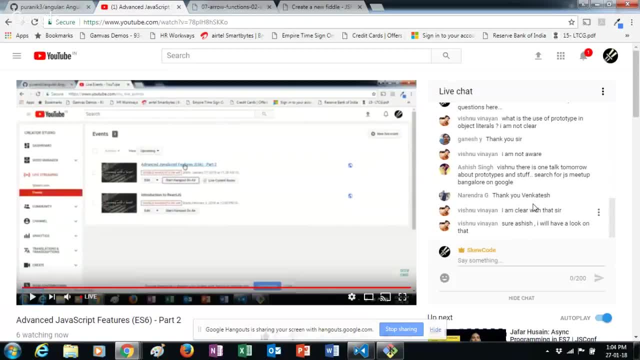 i'll try to cover that, uh in a simple manner, as simple as i can. all right, guys, thanks, thanks a lot, so i think there is no more questions. thank you, thanks, vishnu. all right, no more questions. so i think we can call it a day.